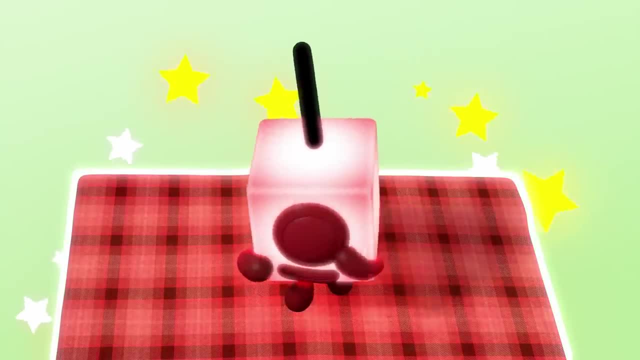 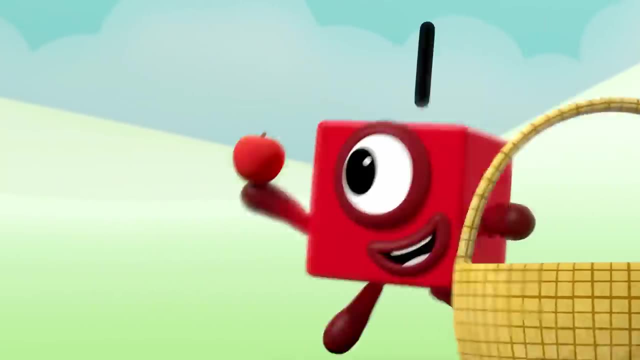 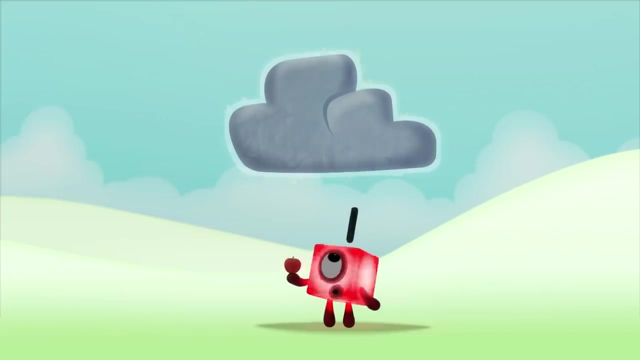 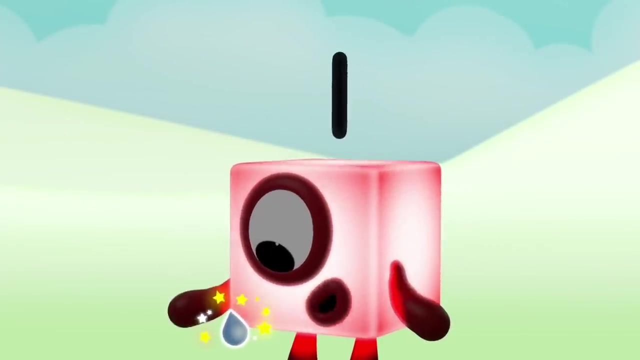 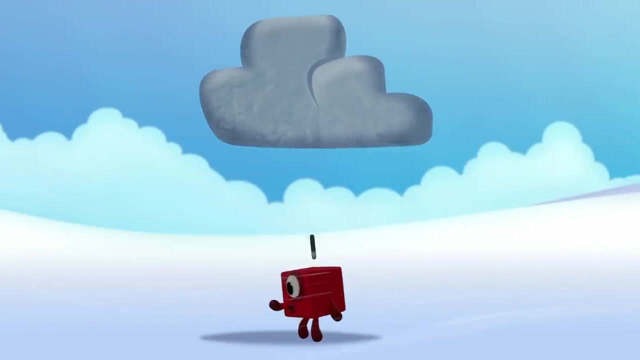 I'm one of a kind: Oh One One blanket, One One basket One Hello, apple One One cloud. Oh One One raindrop, Aha One One umbrella, Oh One One wet me. 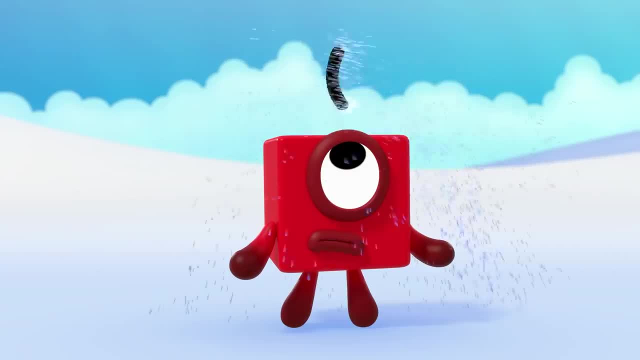 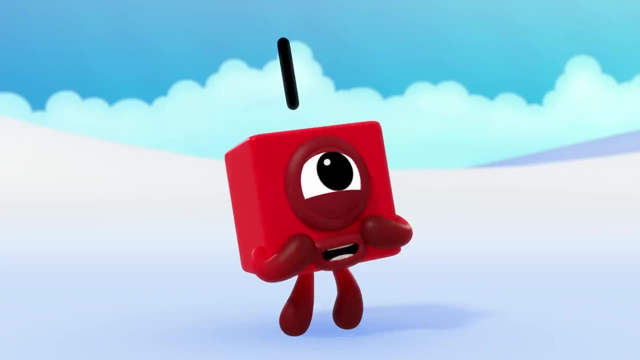 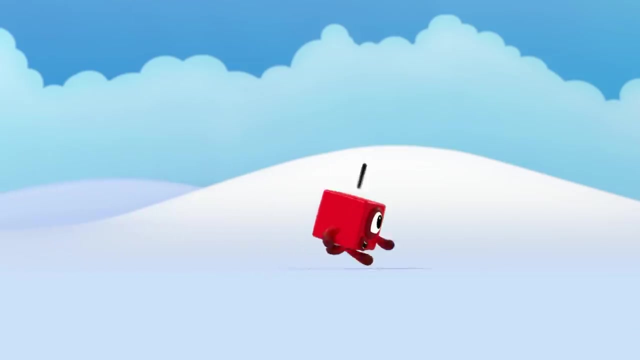 Did you see that, Hello? Oh, It could be lonely If I'm the only one. It might not be much fun Being a single figure, But I'm number one And I'm winning. I'm only at the beginning. I could be the start of something. 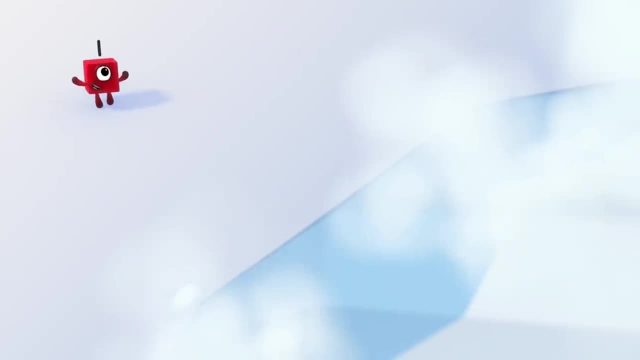 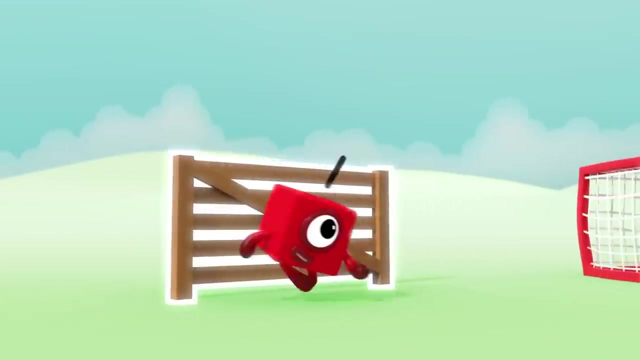 Maybe I could be part of something Bigger: One mountain to climb, One sun, One step at a time. One horse in this race, One smile on my face. One bat, one ball. One box, one boat, One gate, one goal, One goose, one goat. 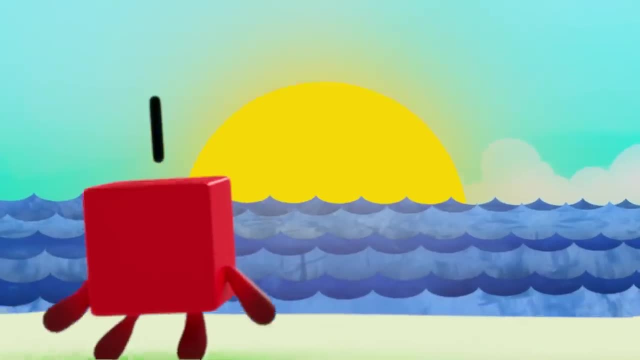 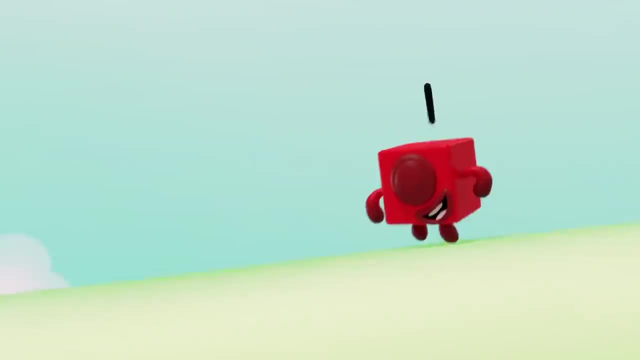 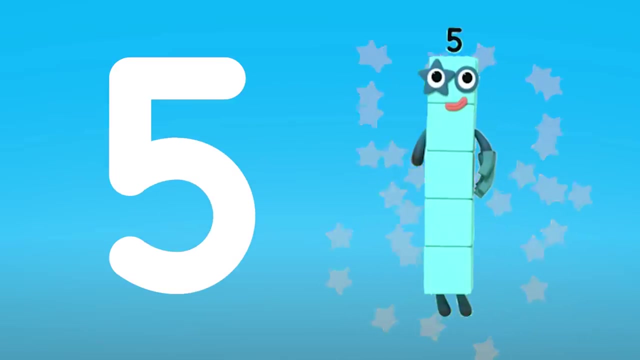 One cat, one cow, One cake, one cat, One hole, one hop, One hen, one cat, One wonderful, beautiful view As far as the eye can see. One wonderful world. One wonderful world And one me. I Am One, One, two, One, two, three, four. 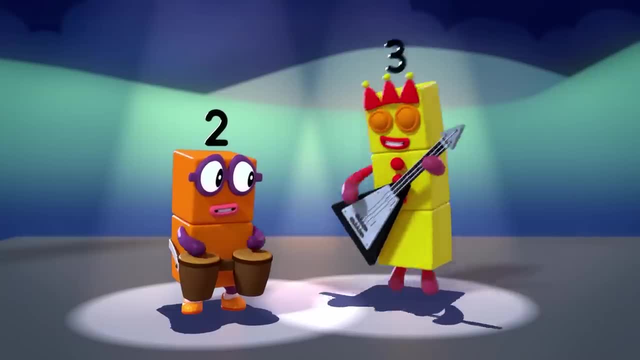 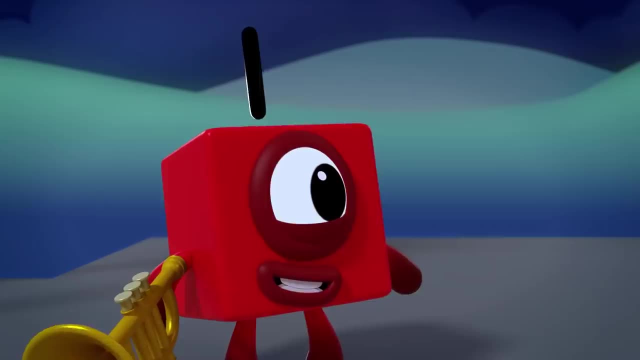 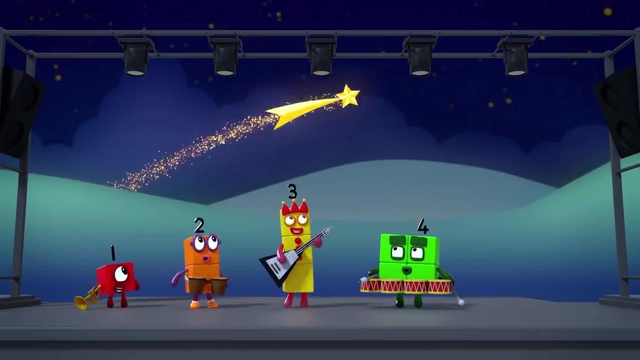 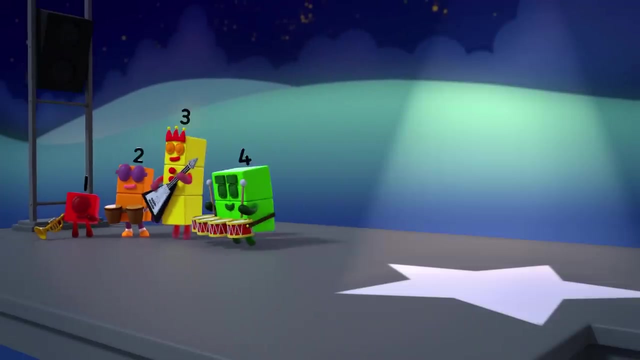 Oh, Too slow, You're too fast, I can't keep up. Stop. That was one awful sound. We need someone to sort us out. We need someone to sort us out. Let's see who's the best. Oh, A shooting star, Make a wish. Oh, 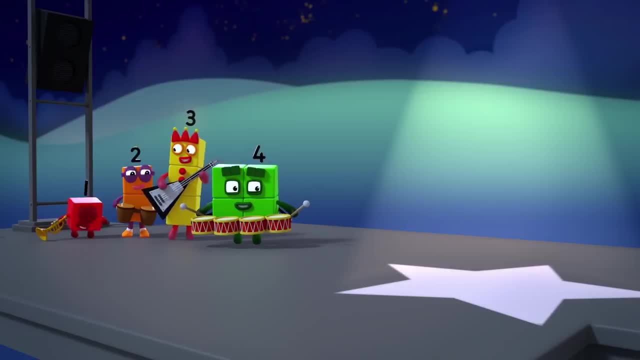 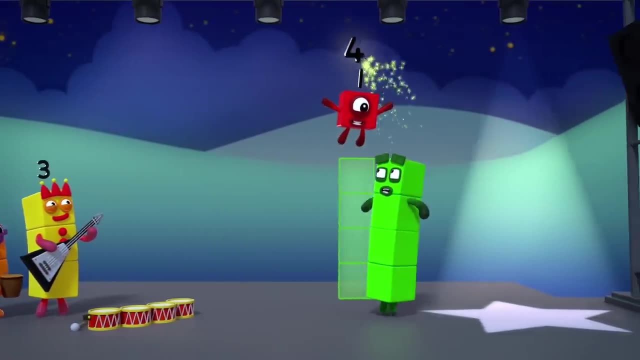 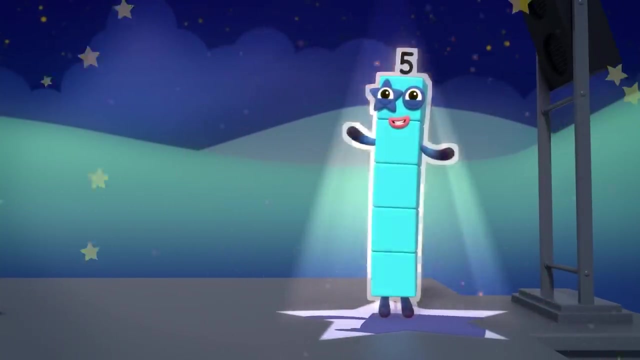 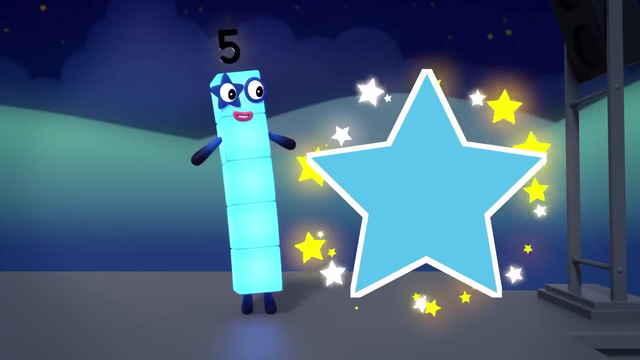 It's star shaped. Who's it for Me? Well, I'm the biggest, I'll go first. Four Plus one equals Five. I am five. I feel so alive. One, two, three, four, five, Five points. Oh, a star is born. 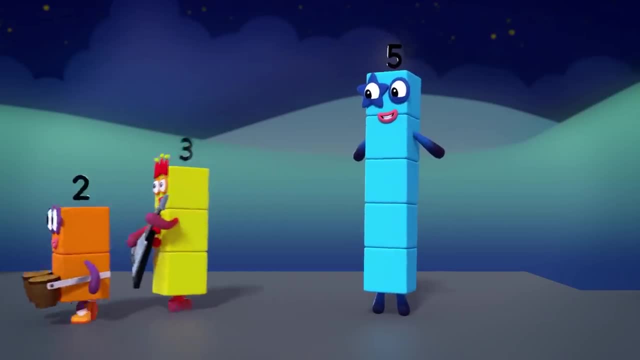 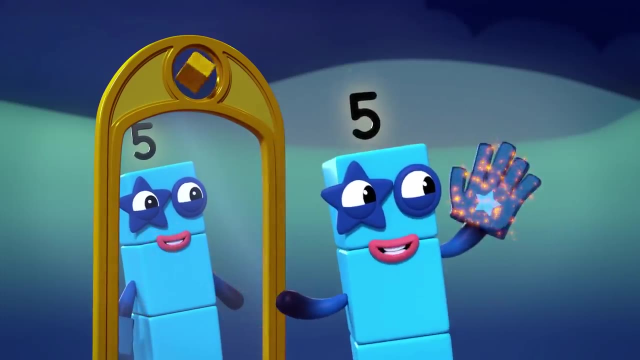 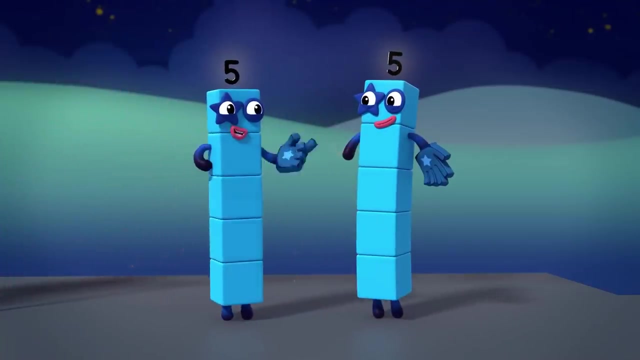 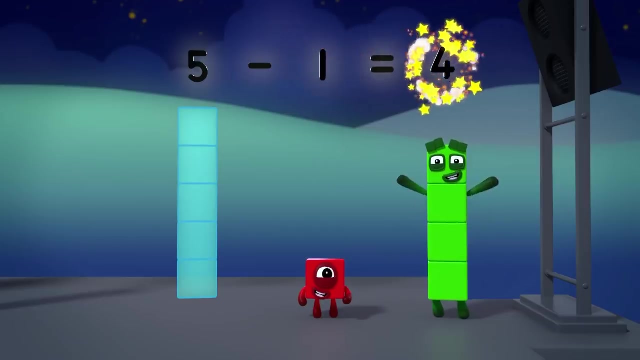 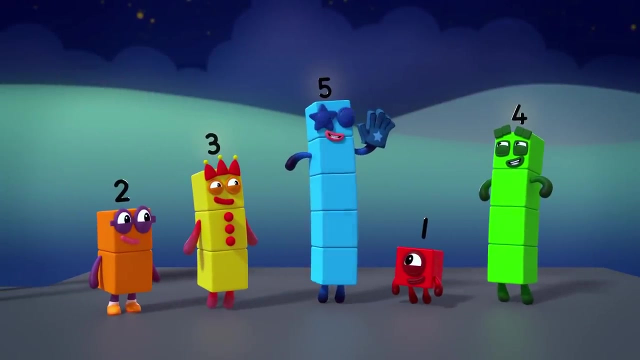 I don't know about that. Take a look, High five, High five. Oh, A big hand for you, High five. Five minus one Equals four. And who are you? I'm five And you can count on me to get this party started. 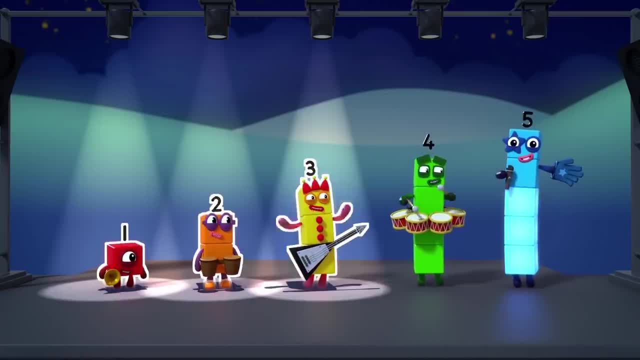 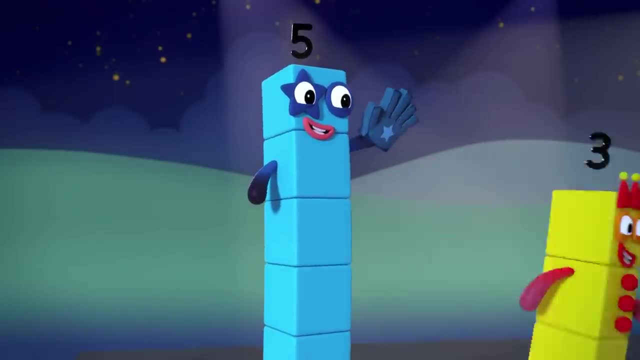 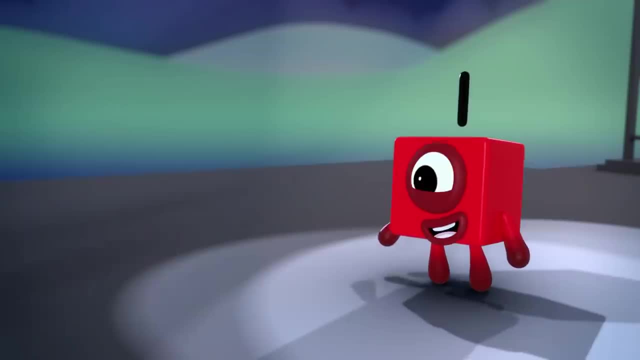 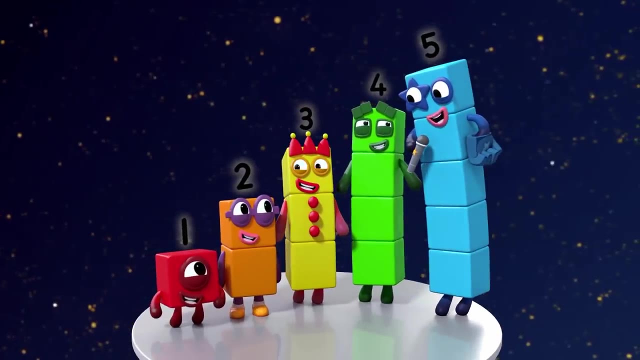 High five, High five, High five To the side up above, down low, too slow. High five. Oh, I feel so alive. You know that you've arrived when you're with number five: Five points and a shooting star. 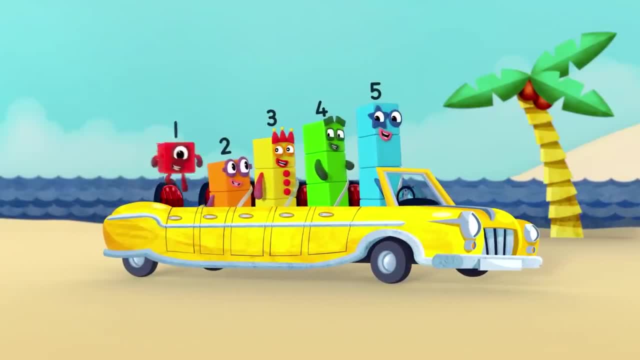 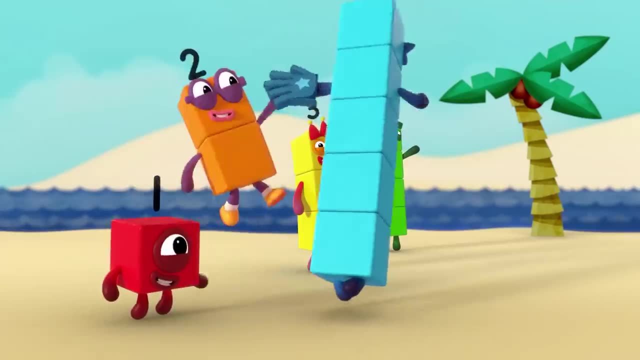 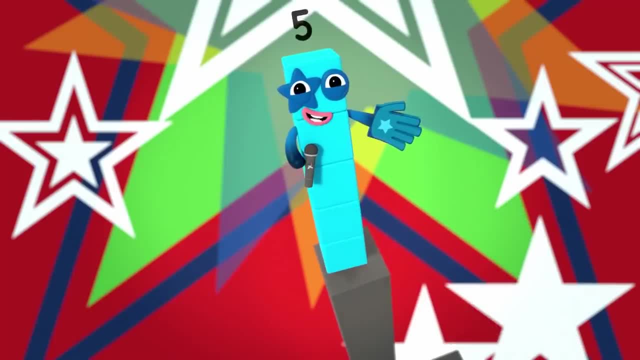 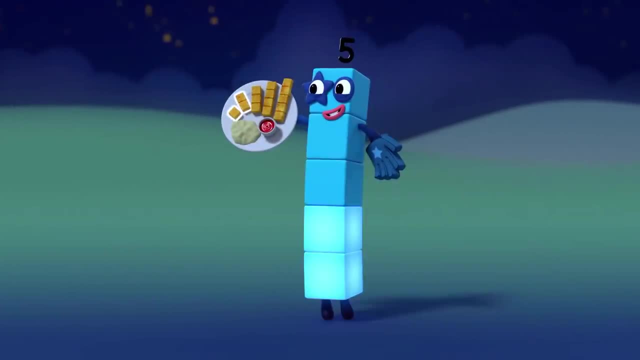 Ooh, I feel so alive. You know that you've arrived When you're with number five. Five fish fingers on a plate: One, two, three, four, five. Five bars on a five-bar gate: One, two, three, four, five. I'm fine. 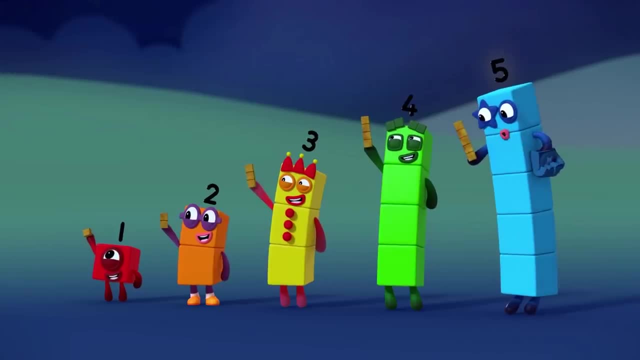 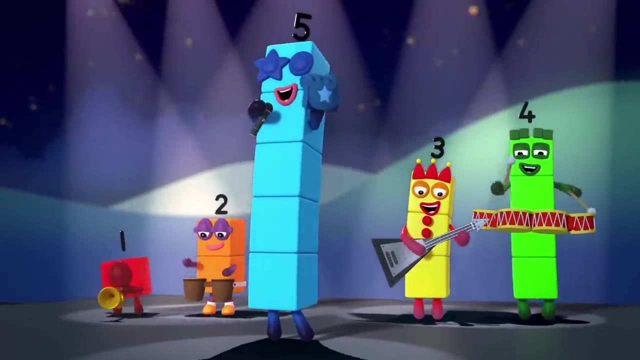 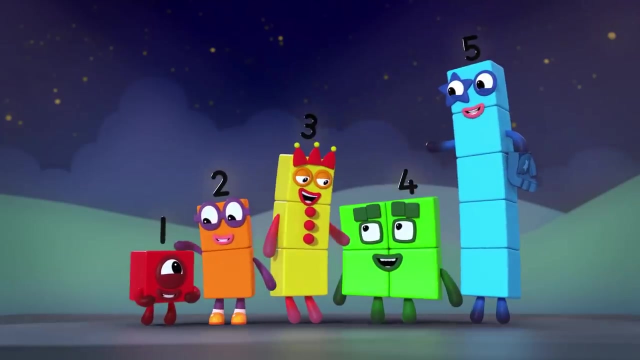 Ooh, I feel so alive. You know that you've arrived. When you're with number five, I'm number five And I hope you understand. Whenever you need help, I'll be there to lend a hand. Now the band is all together. The rest can join the queue. 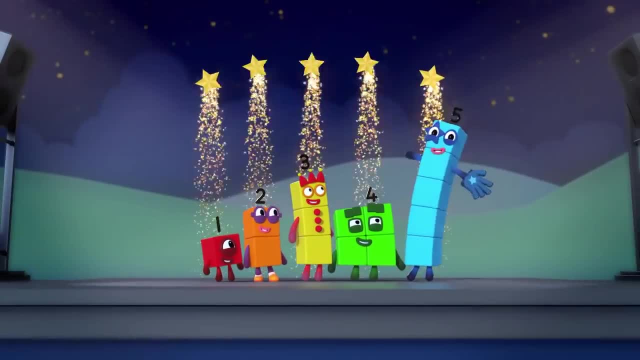 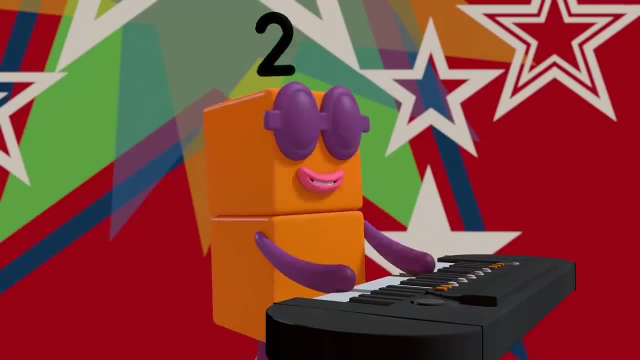 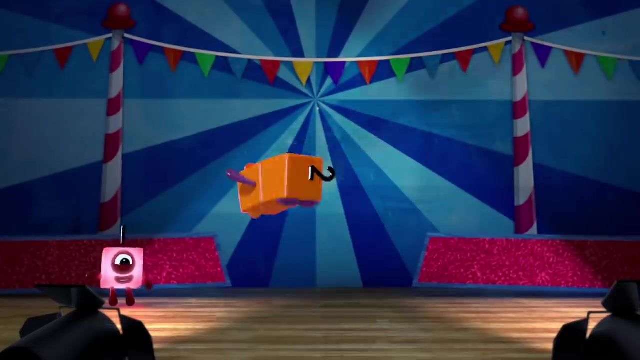 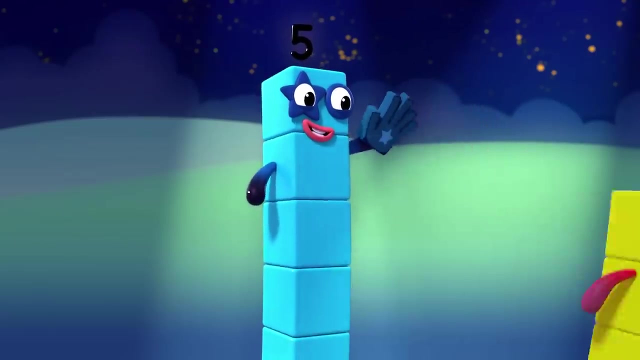 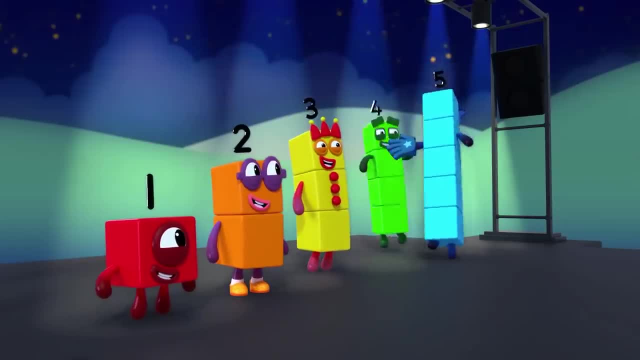 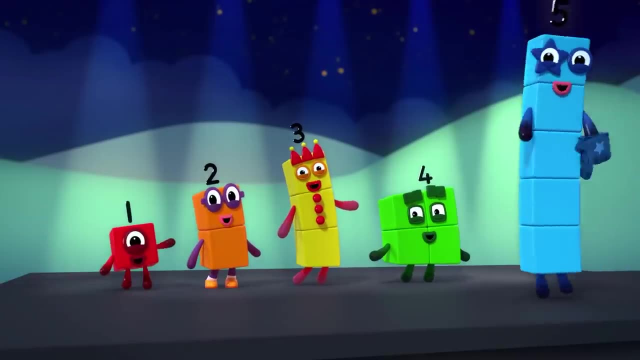 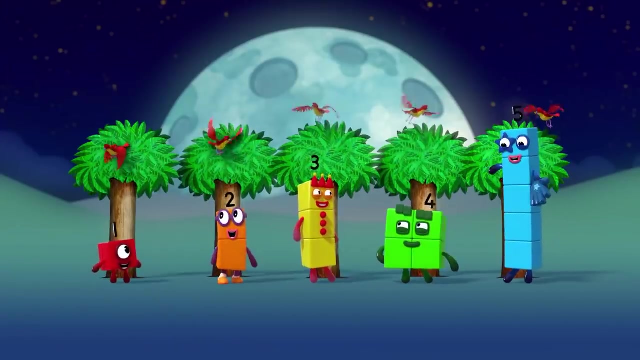 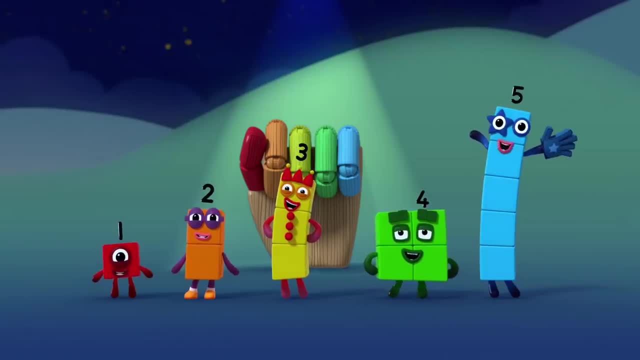 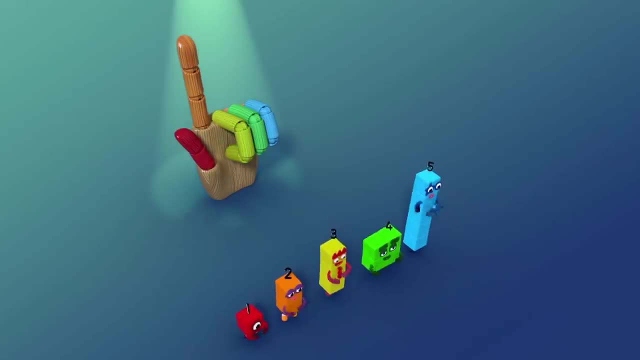 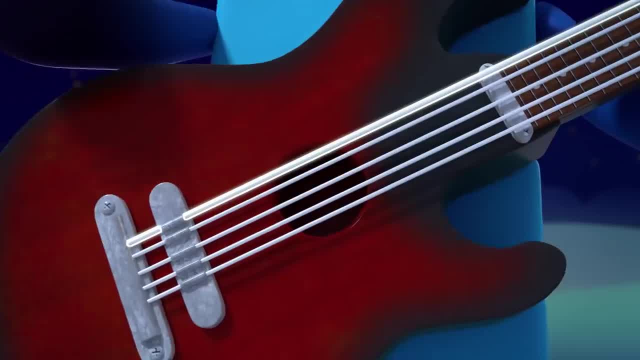 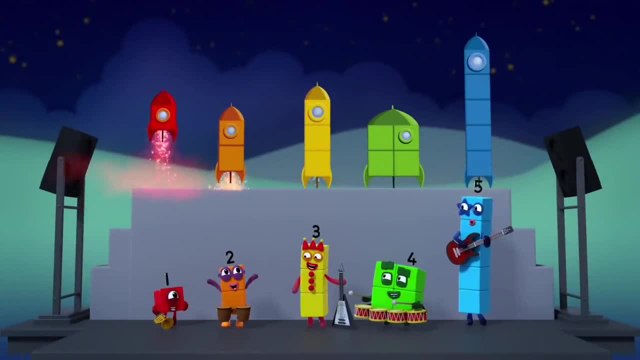 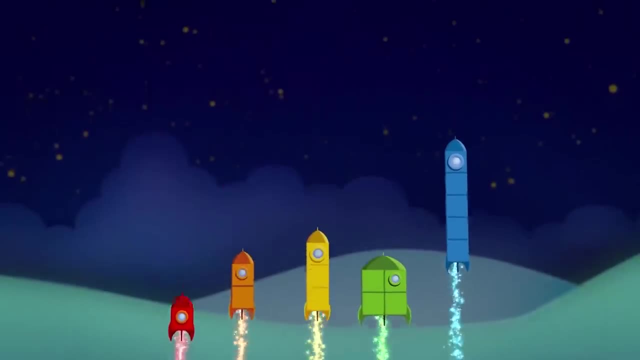 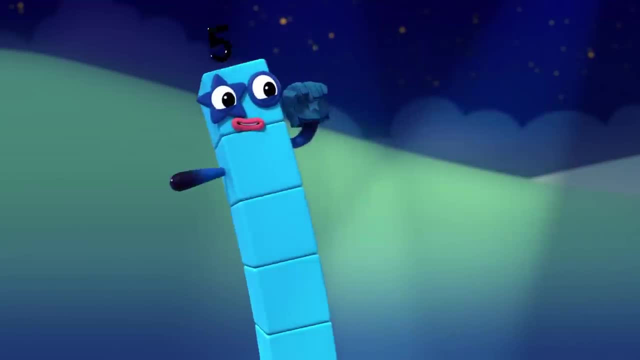 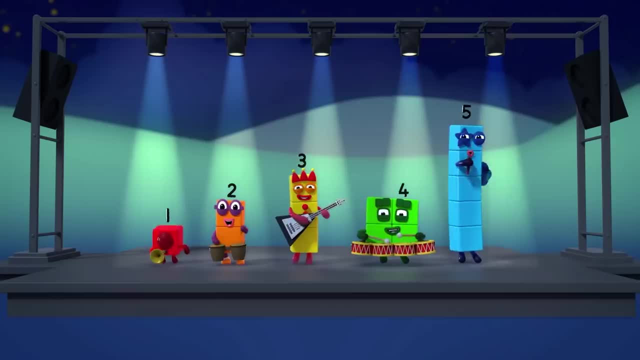 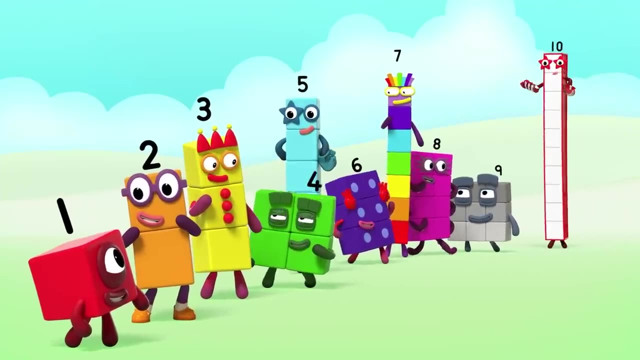 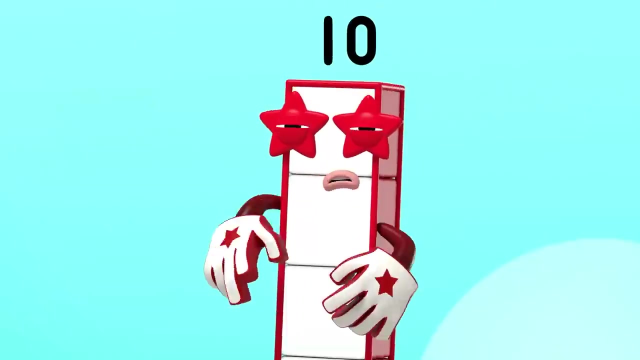 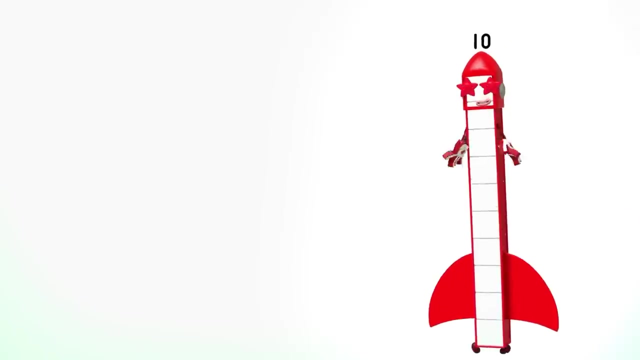 Ooh, I'm so alive. You know you've arrived. When you're with number five. What shall we do today, Please, Oh, okay, Let's do everything. Everything, Yes, Ten, nine, eight, seven, six, five, four, three, two, one. 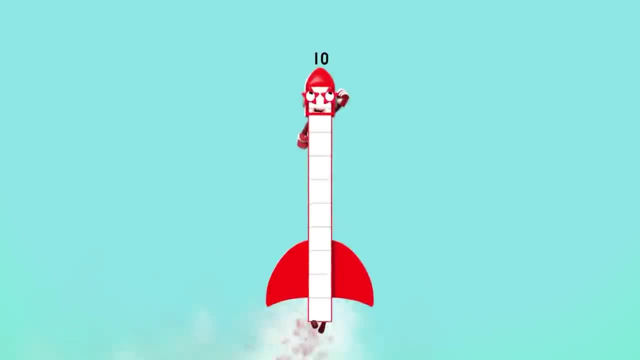 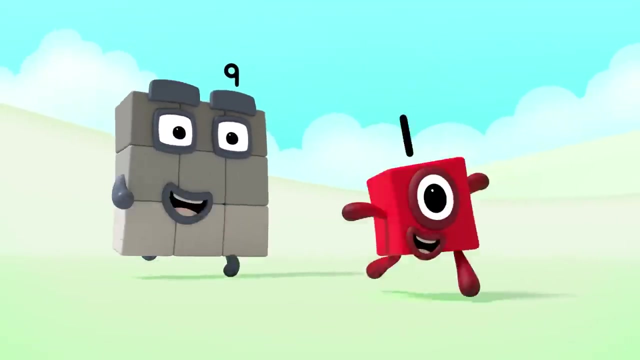 Blast off. I'm ten ten, ten And I'm flying through the sky. I'm ten, ten, ten. You can break me up any way you like. I can be Nine plus one, Going for a run, Trying not to sneeze And having lots of fun. 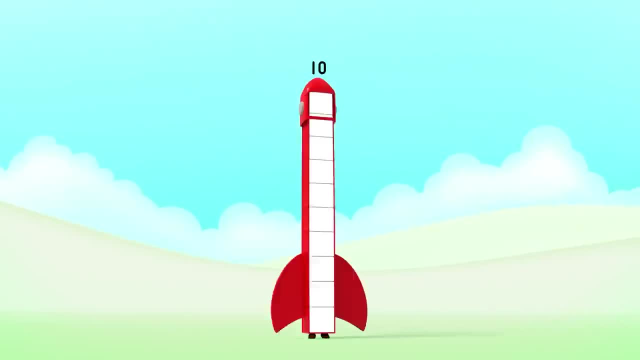 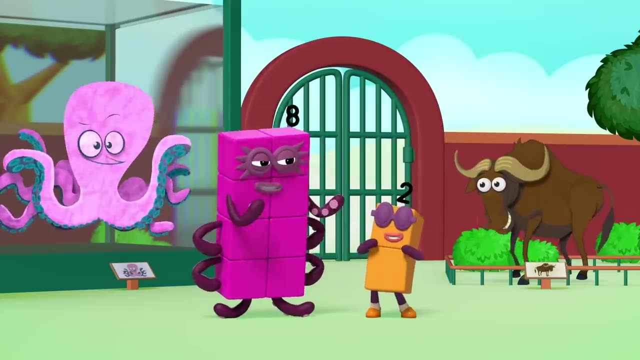 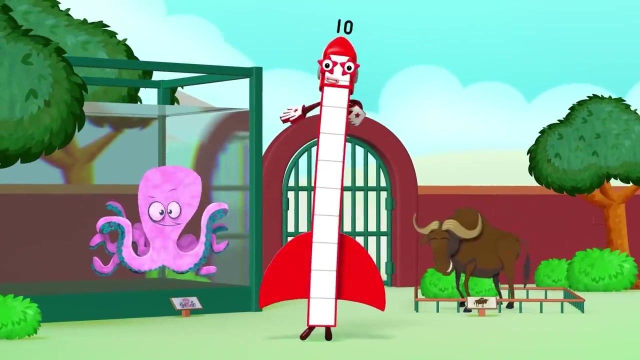 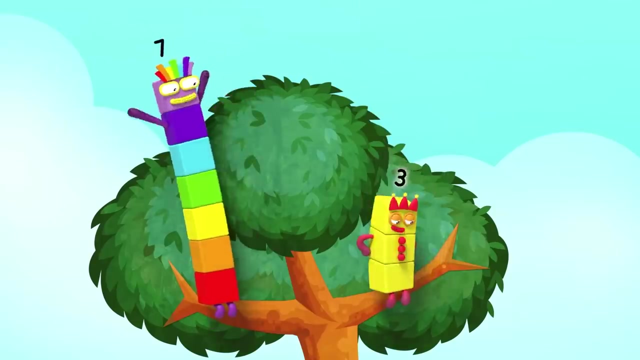 And then I'm ten, ten, ten again. I can be Eight plus two Visiting the zoo, Talking to the octopus And dancing with a canoe. And then I'm ten, ten, ten again. I can be Seven plus three Sitting in a tree. 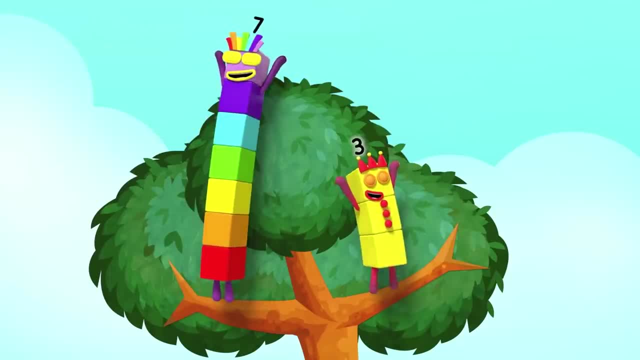 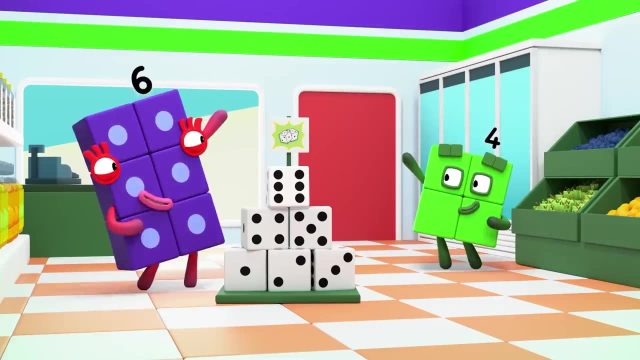 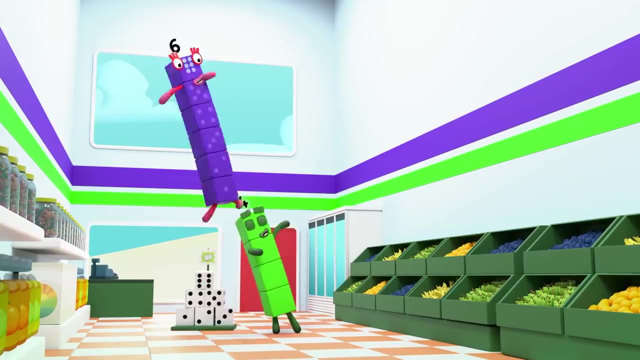 Making rainbows And looking at me. And then I'm ten, ten, ten again I can be. Six plus four: Shopping at the store, Playing with a dice On a square tile floor. And then I'm ten, ten, ten again I can be. 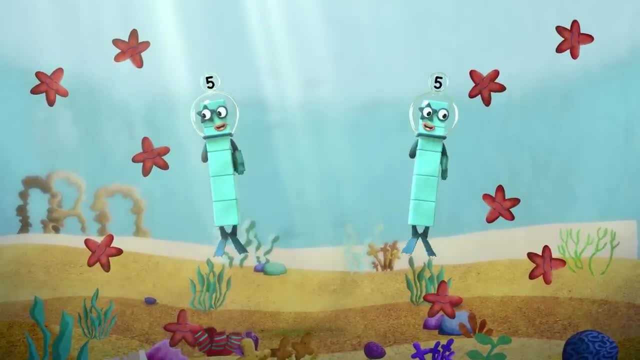 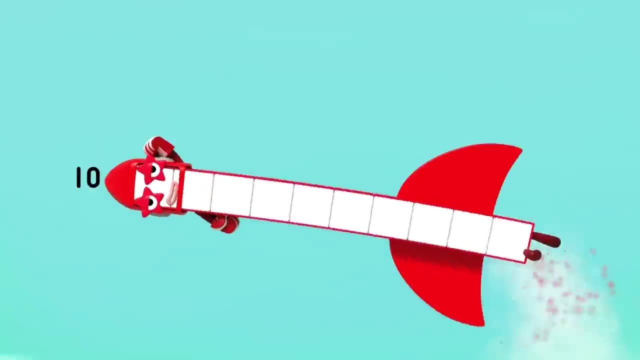 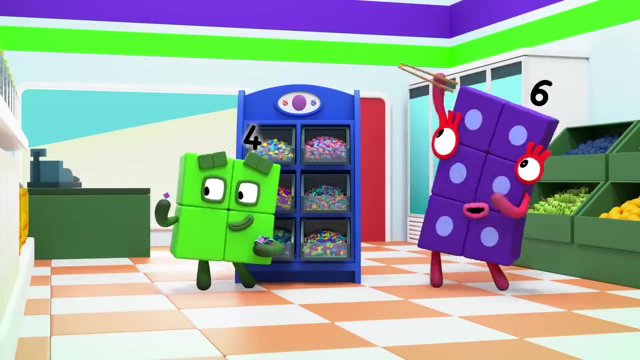 Five plus five On the scuba dive, Swimming with a starfish And doing a jive, And then I'm ten, ten, ten again I can be Four plus six, Playing pick and mix, Picking out the square ones And using chopsticks, And then 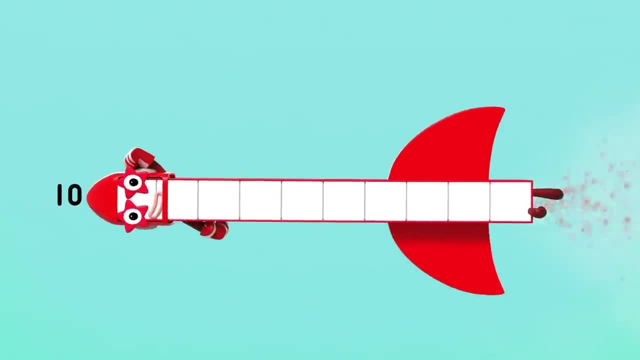 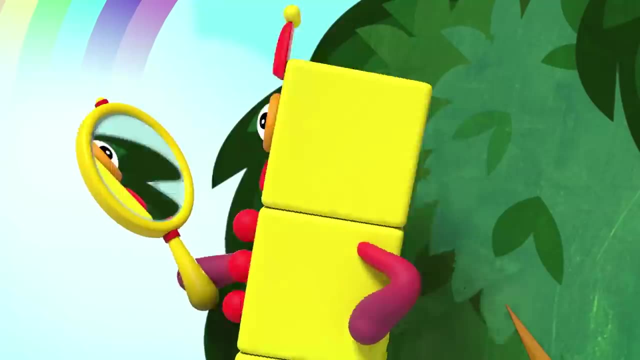 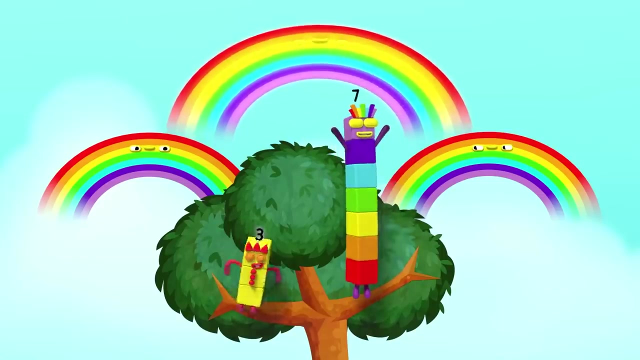 I'm ten, ten, ten again, I can be Three plus seven, Gazing up to heaven, No, looking at me, And a rainbow called Kevin. Kevin And all my rainbows have names: Kevin, Rainbowdina, And that's Big Bob. Hello, And then. 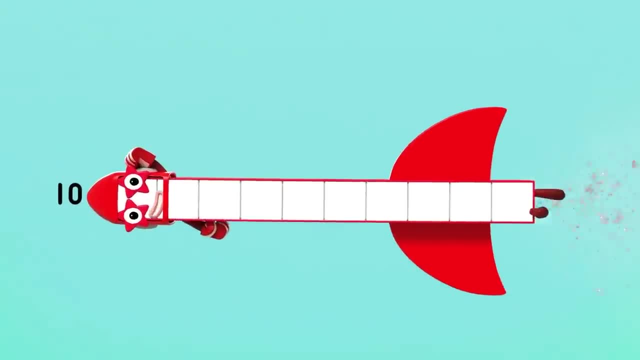 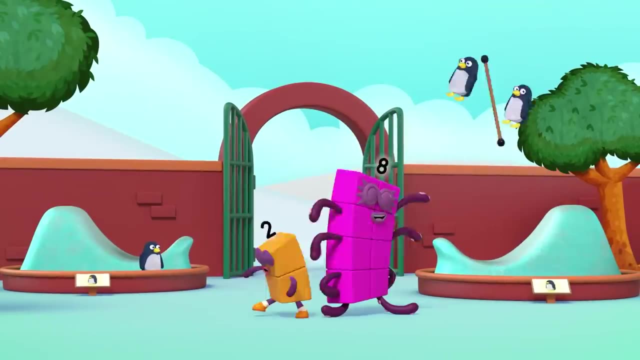 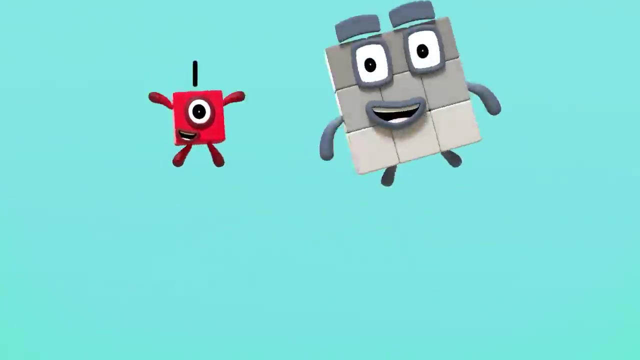 I'm ten, ten, ten again. I can be Two plus eight, Opening a gate, Dancing with a penguin Lifting heavy weights. And then I'm ten, ten, ten again. I can be One plus nine, Starting on a climb, Getting out of breath. now. 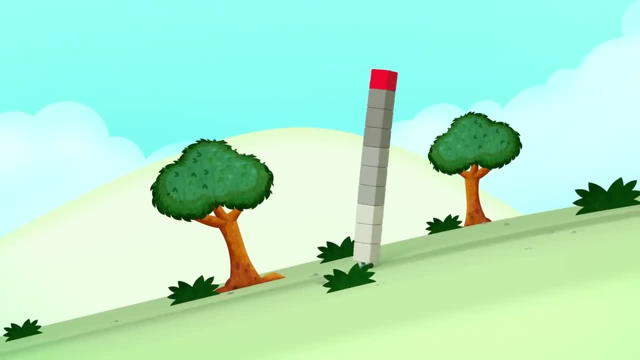 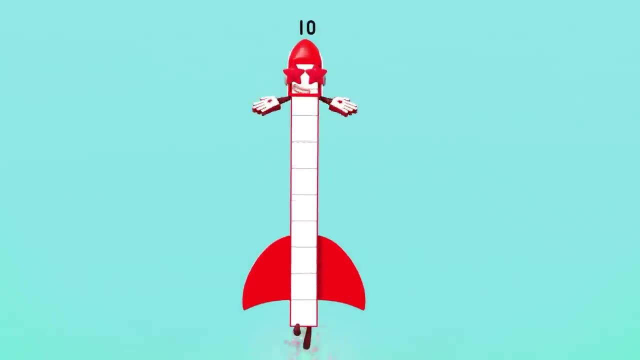 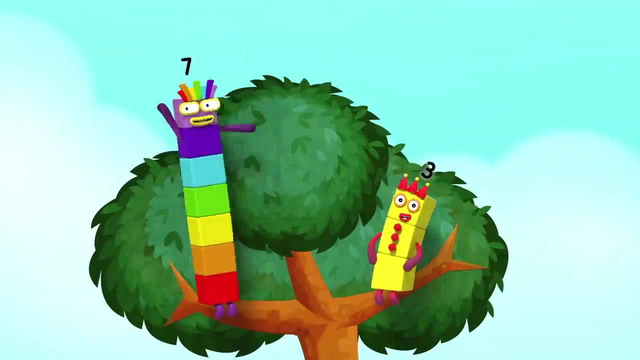 Sneezing all the time. Achoo, I'm ten, ten, ten again, Ten, ten, ten again Again. Nine plus one Going for a run. Eight plus two Visiting the zoo. Seven plus three Sitting in a tree. Six plus four Shopping at the store. 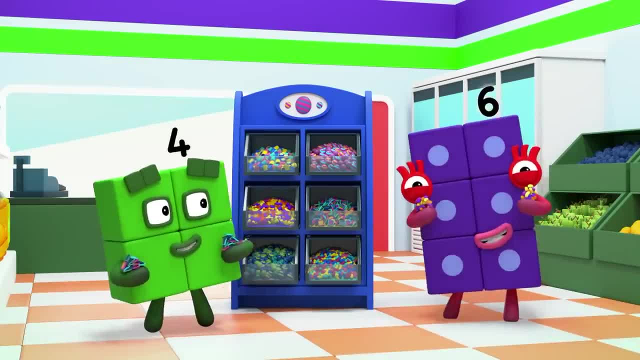 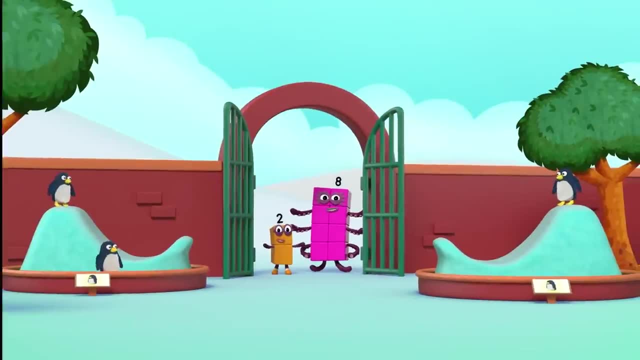 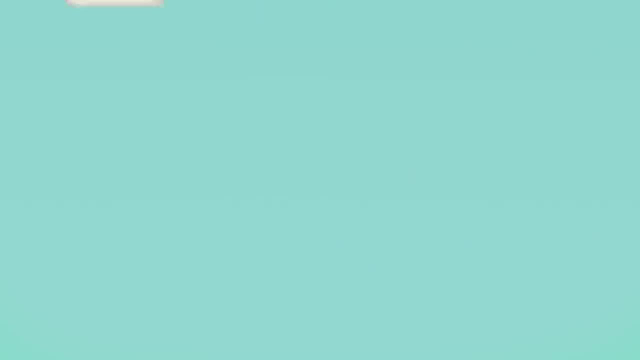 Five plus five On a scuba dive, Four plus six Playing pick and mix, Three plus seven Gazing up to heaven, Two plus eight Opening a gate, One plus nine Starting on a climb. And then I'm ten, ten, ten again, Again Nine plus one. 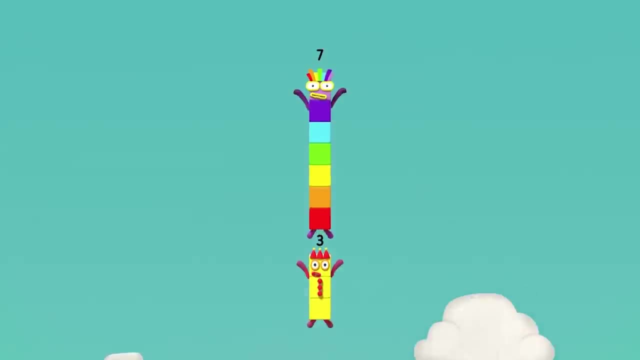 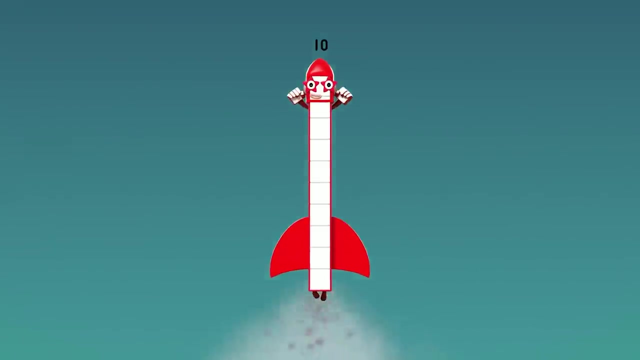 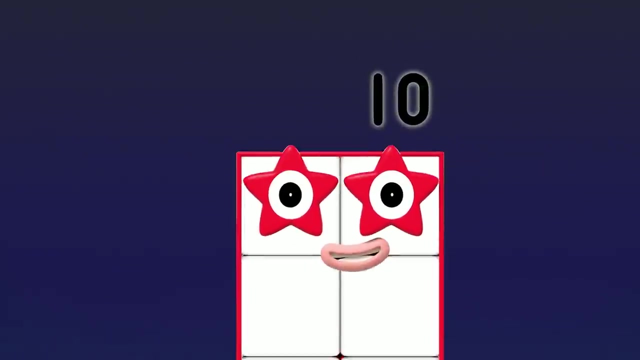 Ten again Eight plus two, Ten again Seven plus three, Ten again Six plus four, Ten again Five plus five, Ten again Four plus six. Ten again Three plus seven. Ten again Two plus eight, Ten again One plus nine, Ten again Ten, when Ten again Nine plus one. 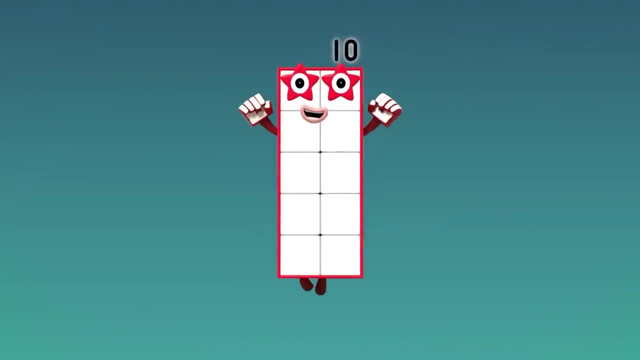 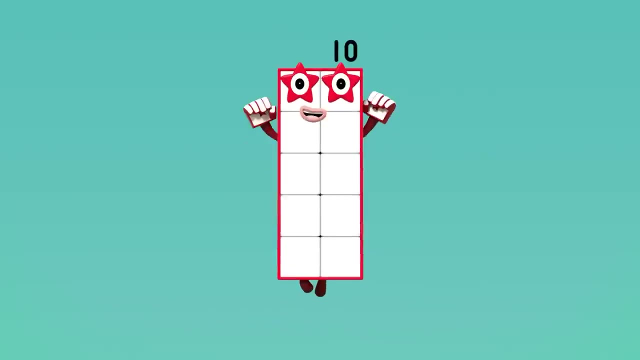 Ten again Eight plus two. Ten again Seven plus three. Ten again Six plus four. Ten again Five plus five. Four plus six. Ten again Three plus seven. Ten again Two plus eight. Ten again One plus nine. Ten again Ten. ten. ten again Again Nine plus one. 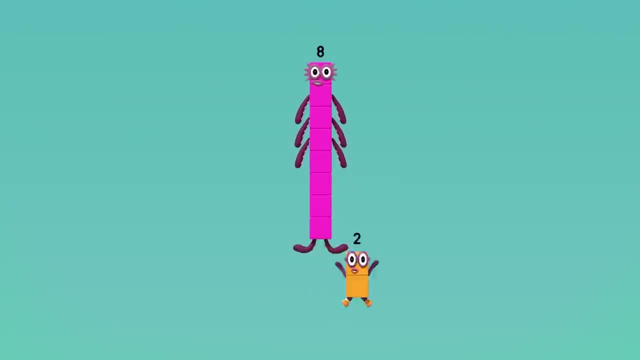 Or one plus nine, Ten, Eight plus two, Or two plus eight, Ten, Seven plus three Or three plus seven, Ten, Six plus four Or four plus six, Ten, Five plus five Or five plus five, Ten, Ten, ten, ten again, Ten, ten, ten again. 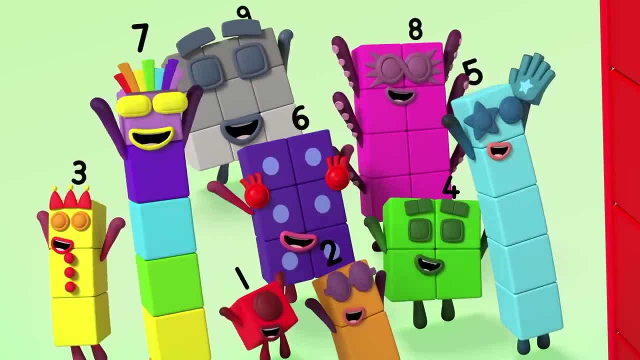 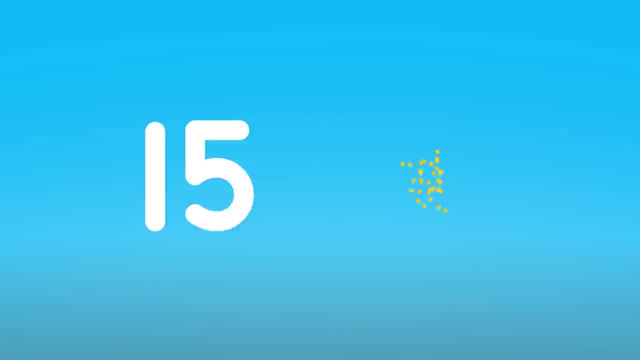 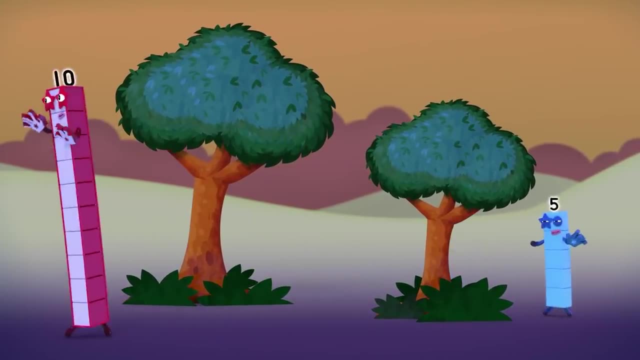 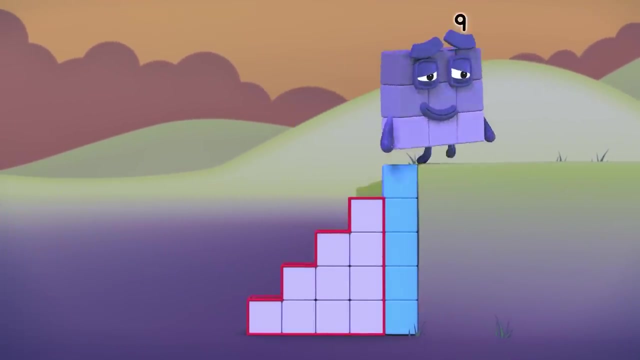 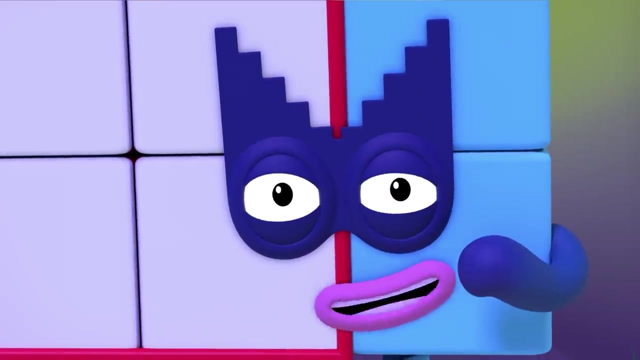 Ten, ten, ten again. And what do you want to do today? Ten, I need a nap. Oh, Hush hush. Ten plus five equals fifteen. Hush hush, I am fifteen And I am a super special, step-shaped secret agent. 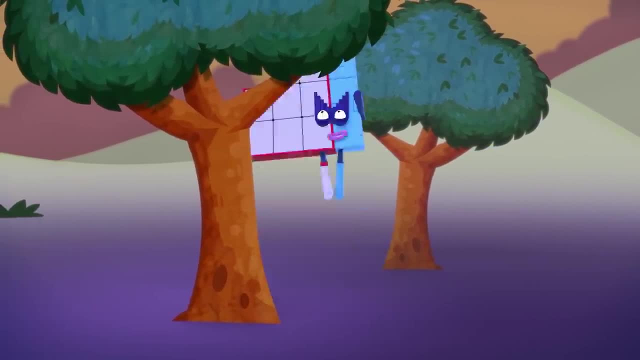 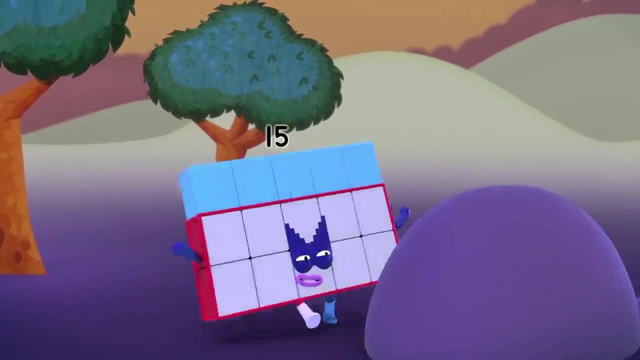 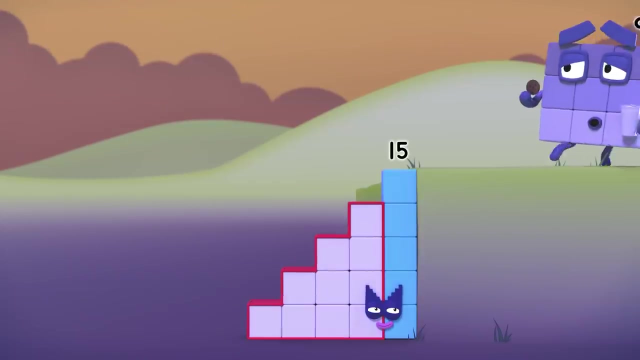 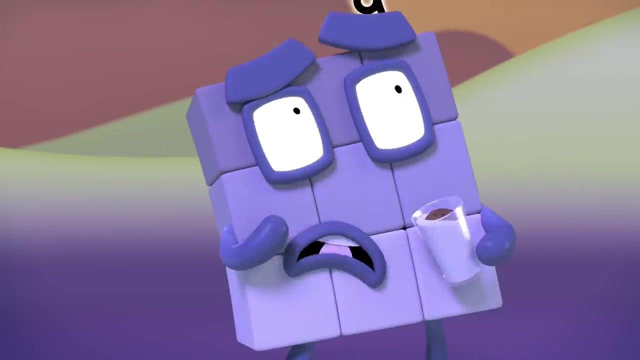 I'm a number with ambition. I'm a number on a mission, With a talent that you won't believe, Despite my size. I'm a master of disguise And I've got a little trick Up my sleeve: Hush, hush, Ah help, My biscuit has fallen into my milk. 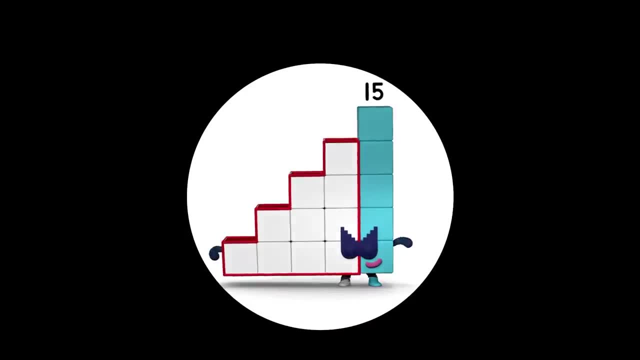 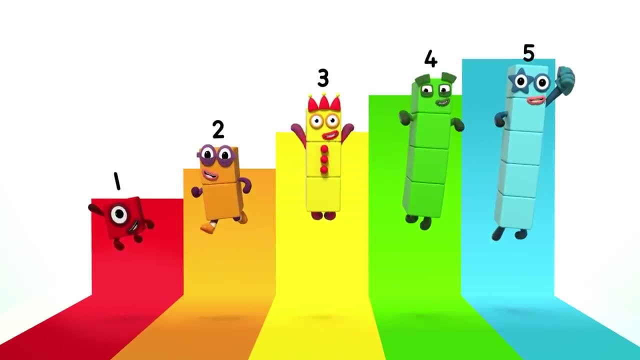 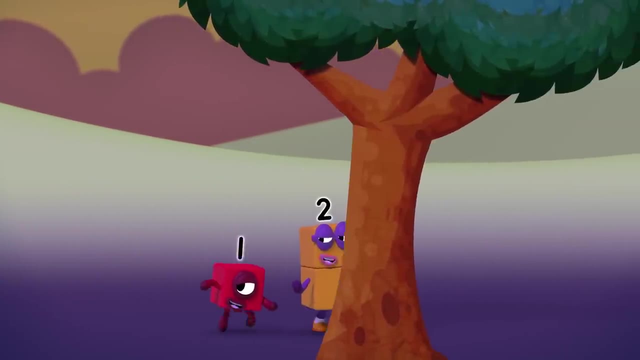 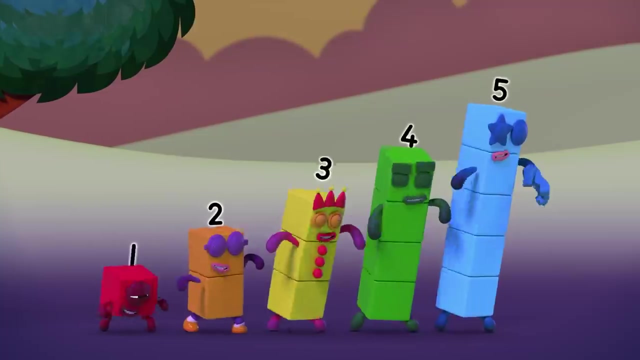 This is a job for Step Squad Five, Four, Three, Two, One Step Squad. We're the super special secret step squad. Step Squad, We can make your problem disappear. We're the super special secret step squad. We're gonna make it better. You'll never even know I was here. 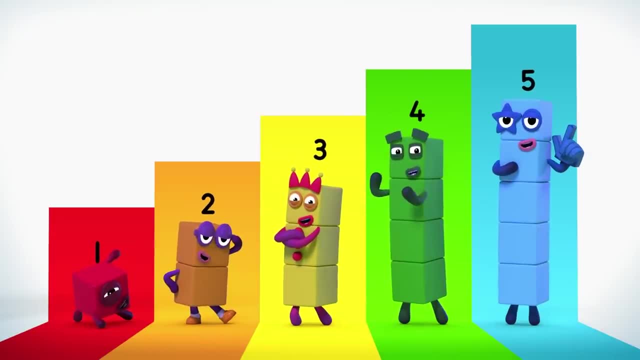 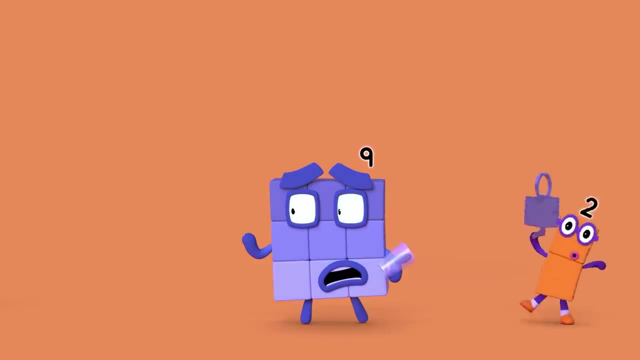 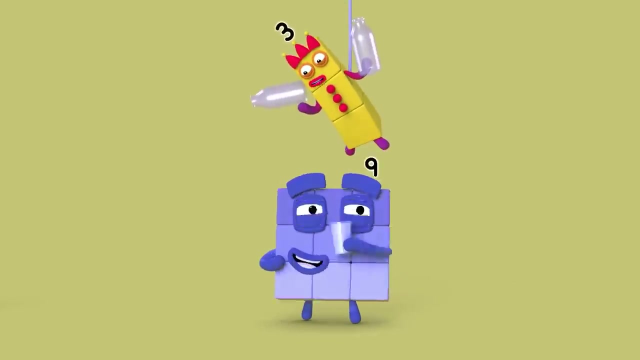 The super special secret step squad is here. Step one: remove the milk. That'll get you started. Step two: remove the biscuits. And now we're on our way. Step three: replace the milk. Don't be downhearted. Step four: replace the biscuits. We're gonna save the day. 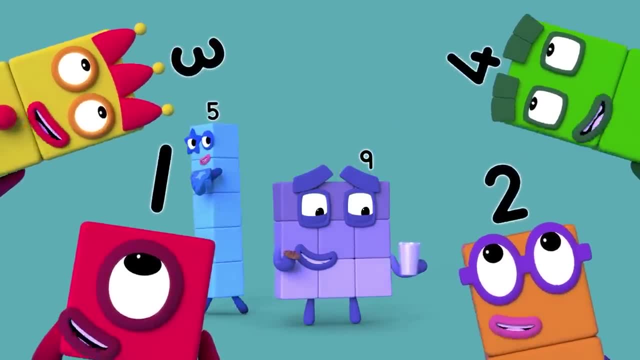 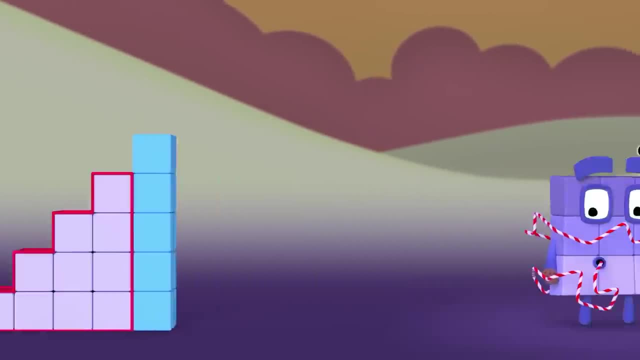 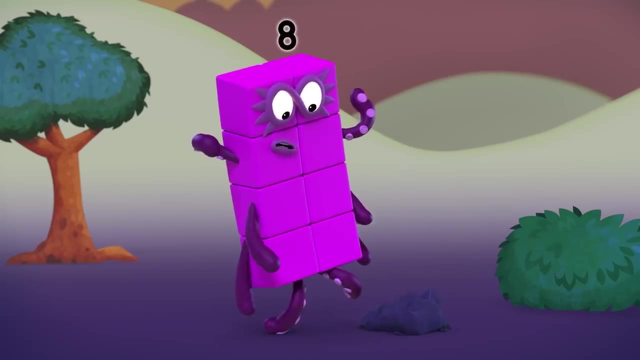 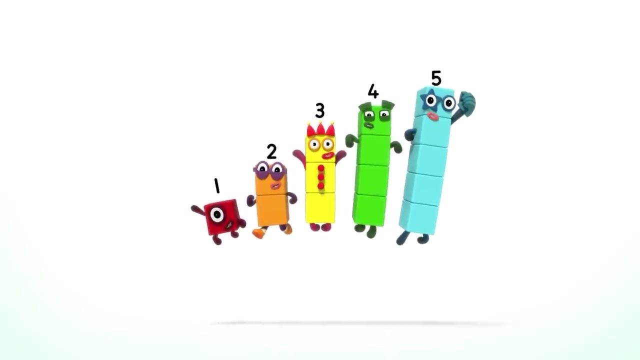 Step five: we're going to overtime, As we give you a straw, Thanks, And vanish away. Yum yum, Octoblock. ouch, I've got an octo-boo-boo. This is a job for step squad. The super special secret step squad is here. 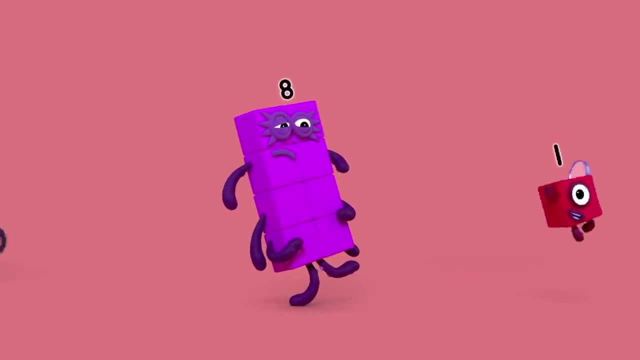 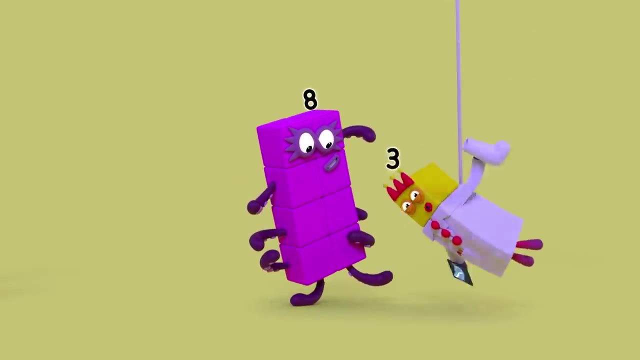 Step one: check the boo-boo, That'll get you started. Step two: nee-no, nee-no, And now we're on our way. Step three: see the doctor, Don't be downhearted. Step four: bandage boo-boo. We're gonna save the day. 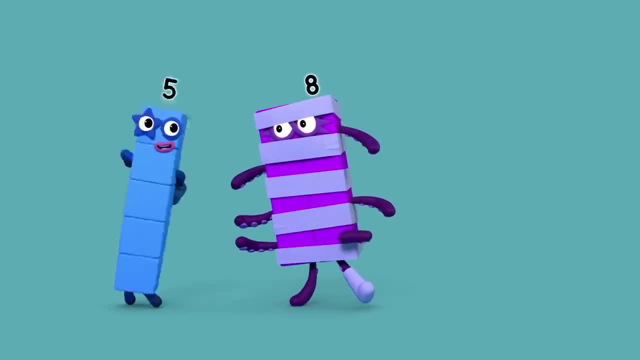 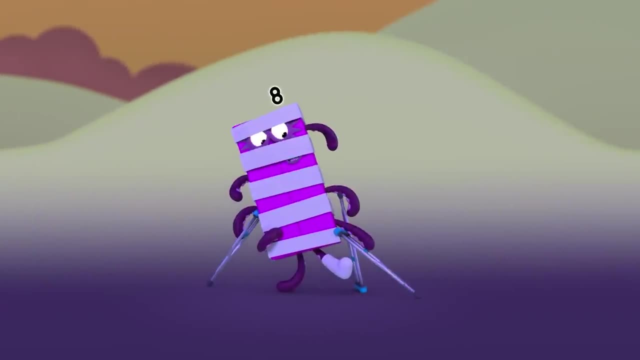 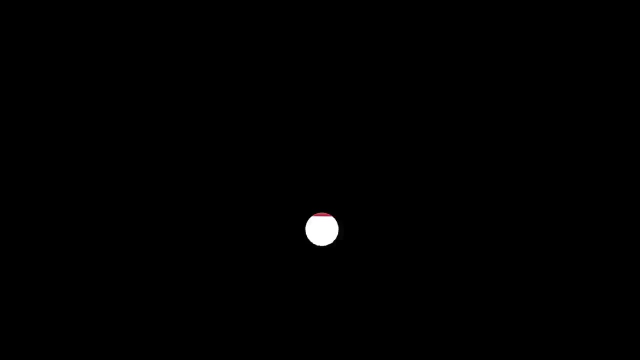 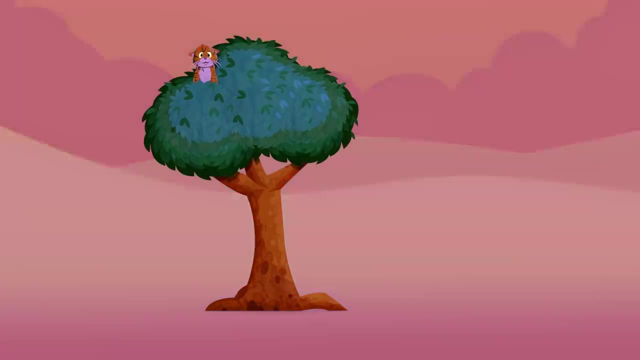 Step five: we're going to overdrive As we make it all better And vanish away All better. now, Meow, Meow-meow-meow-meow-meow, Meow-meow, The super special secret step squad is here. Meow, Step one: get a ladder. 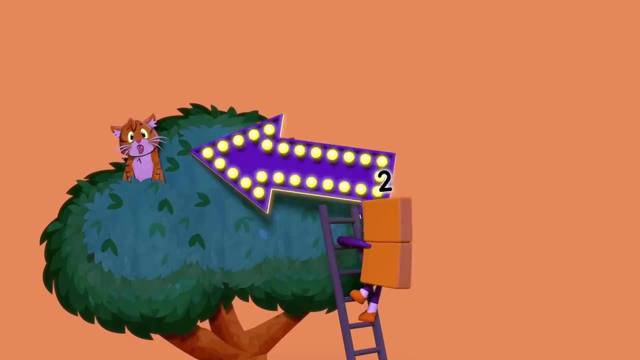 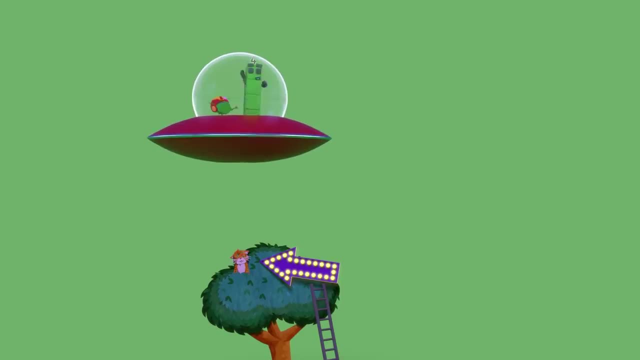 That'll get you started. Step two: light up the tree, And now we're on our way. Step three: call an alien, Don't be downhearted. Step four: beam up the cops, We're gonna save the day. Step five: we're going to overdrive. 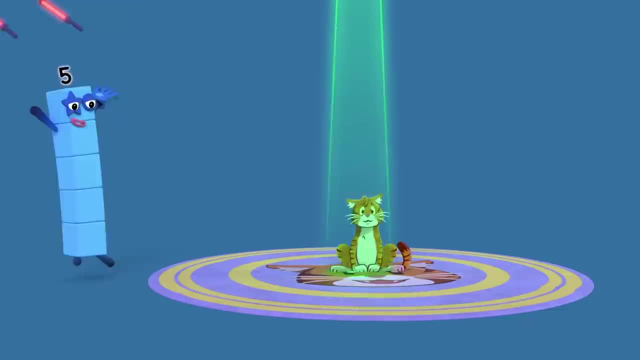 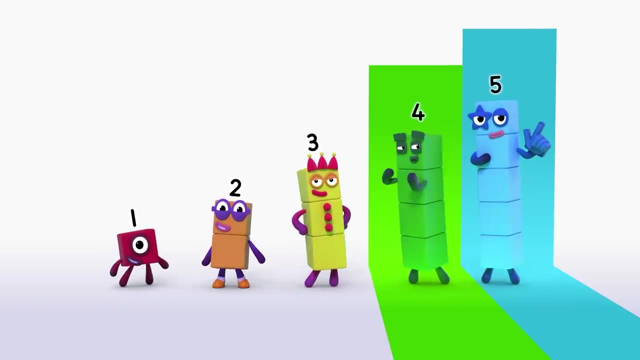 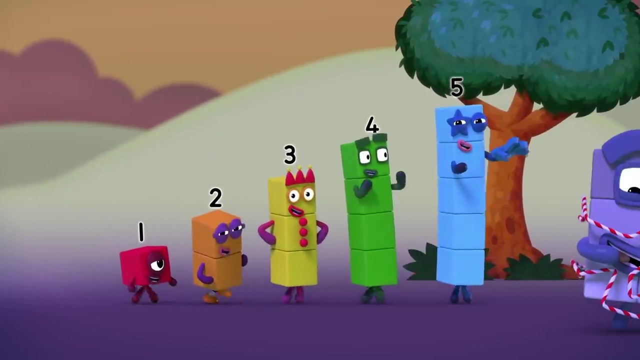 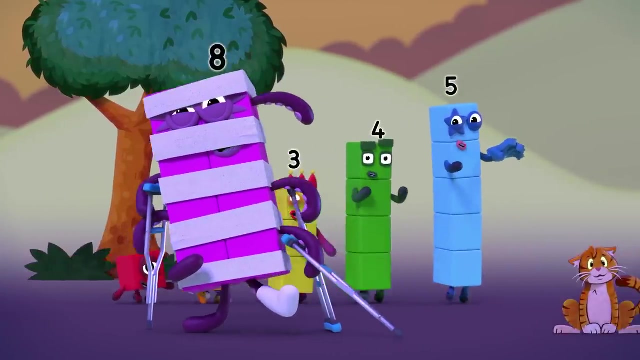 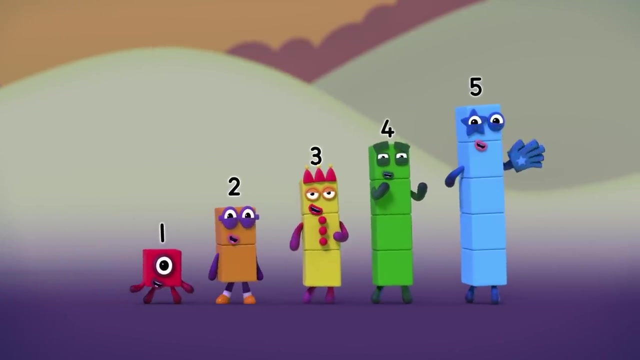 As we beam it back down And vanish away. Five, Four, Three, Two, One Step squad. We're the super special secret step squad. We can make your problem disappear. We're the super special secret step squad. We're gonna make it better And you'll never even know we were here. 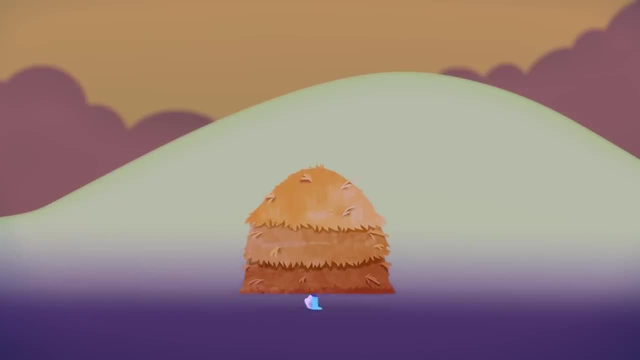 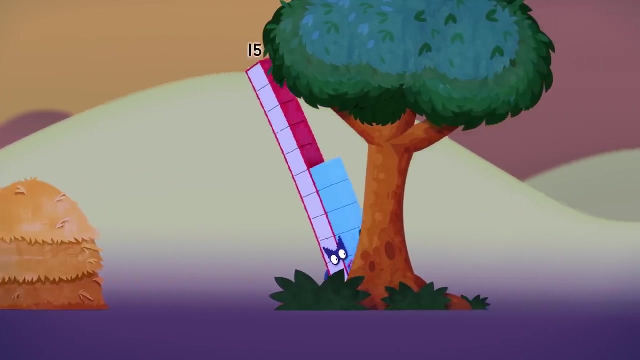 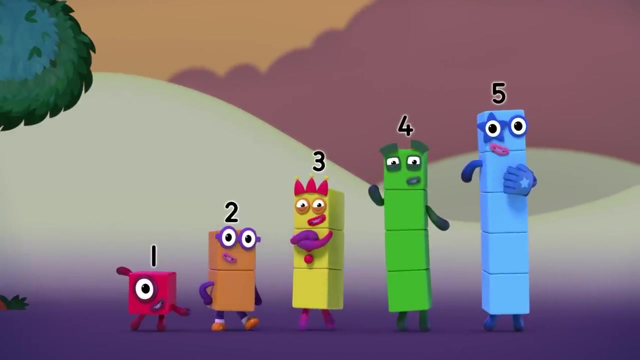 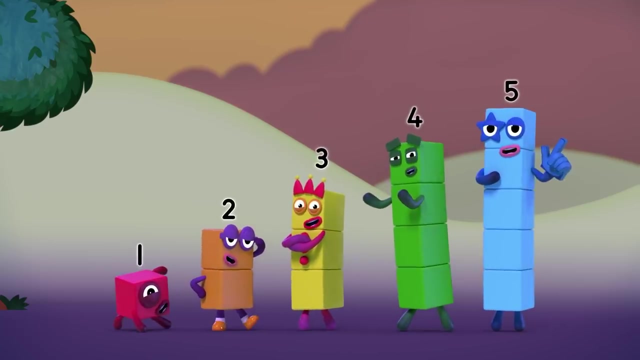 I'm a number with ambition. I'm a number on a mission With a talent that you won't believe, Despite my size. I'm a master of disguise And I've got five friends Who will come and solve your problem. Then we'll leave, Cause we're the super special secret step squad. 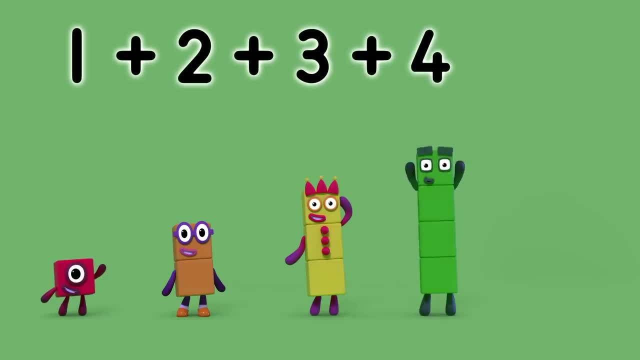 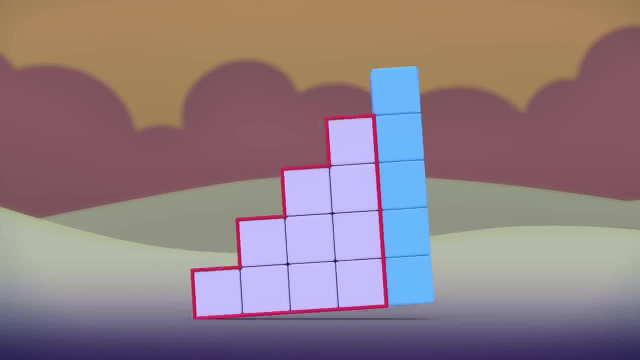 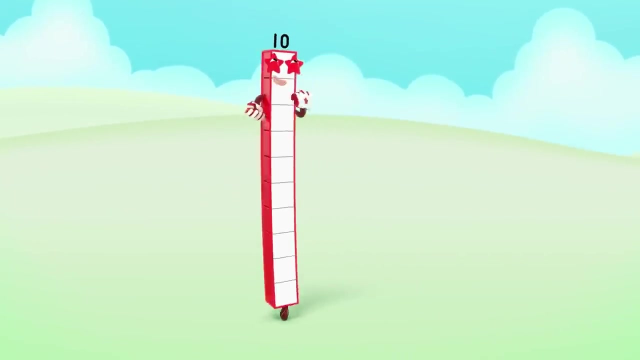 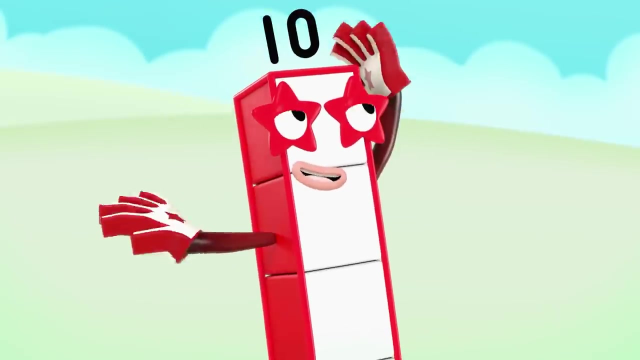 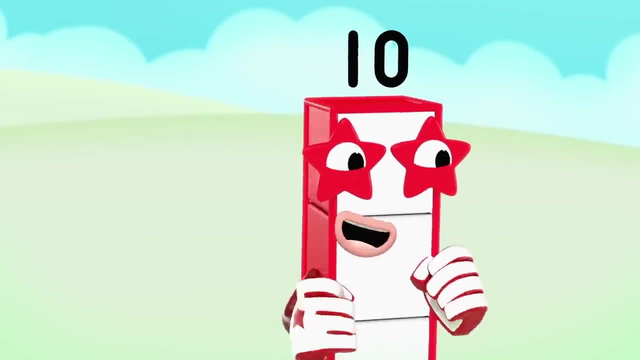 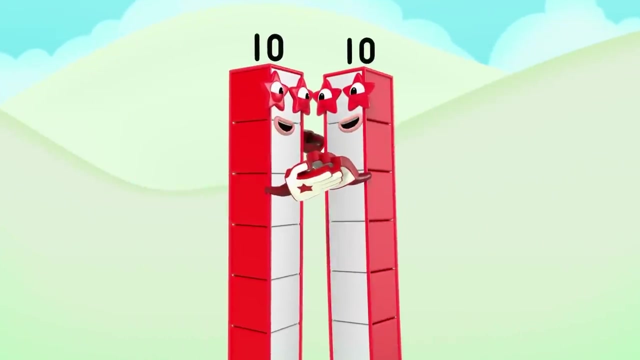 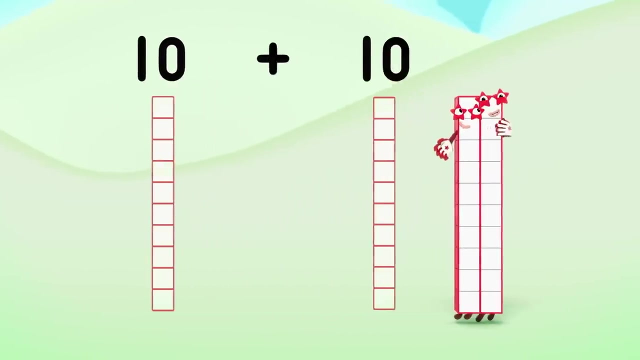 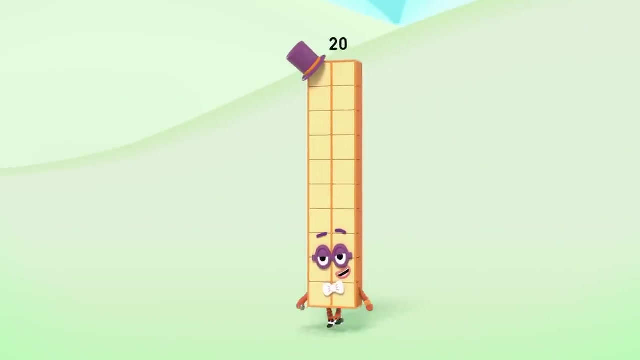 One Plus two Plus three Plus four Plus five Equals fifteen. Hush, hush. Who wants to dance with me? I know someone who wants to dance Me. Shall we dance. Ten plus ten equals Twenty. Hello, hello. Did somebody say Dance? I've got the shoes. 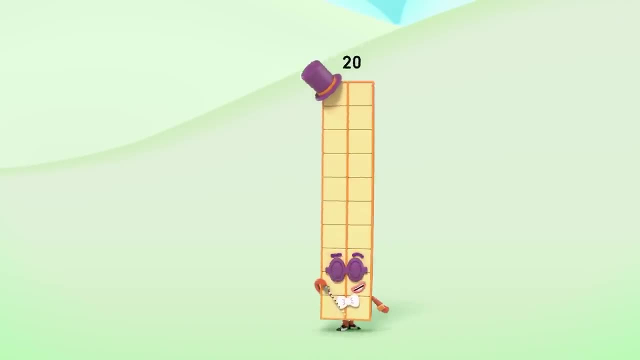 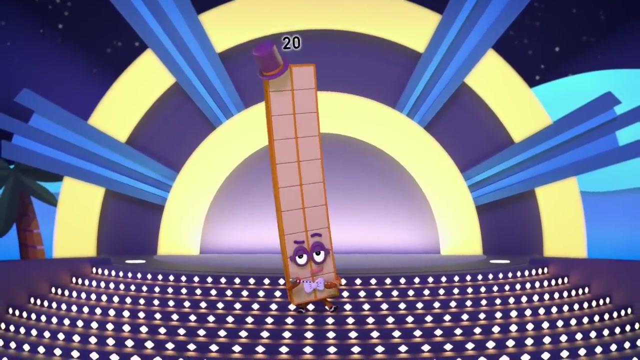 Tap, I've got the cane. Tap, I've got the tip Top, Top, hat, Tap, tap, tap. Are you ready for the big dance number? That's me, I am twenty And I love to dance With plenty of moves to my name. I'm tall and I'm slender. 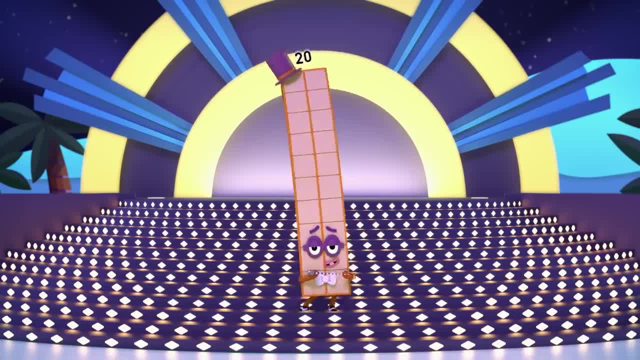 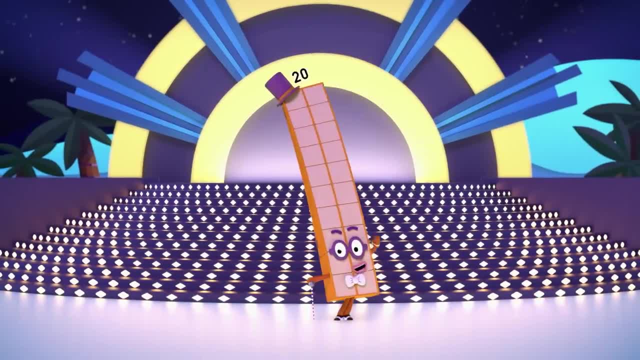 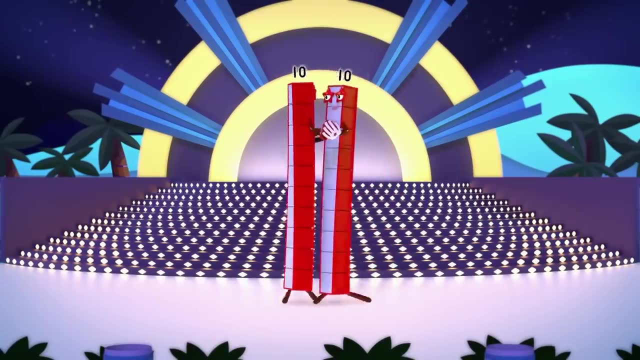 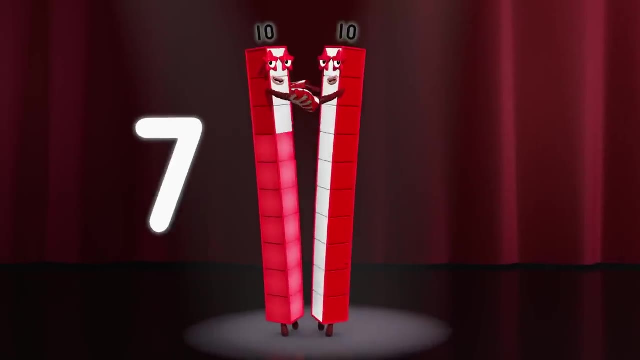 I'm graceful and tender. I sway as I do the fandango Two tens, nothing more, As I take to the floor And dance to the two tens: tango One, two, three, four, five, six, seven, eight, nine, ten. 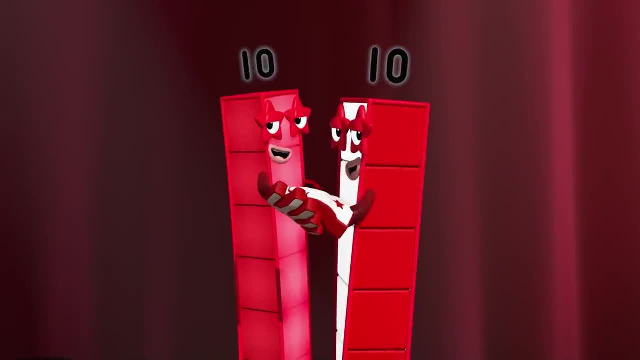 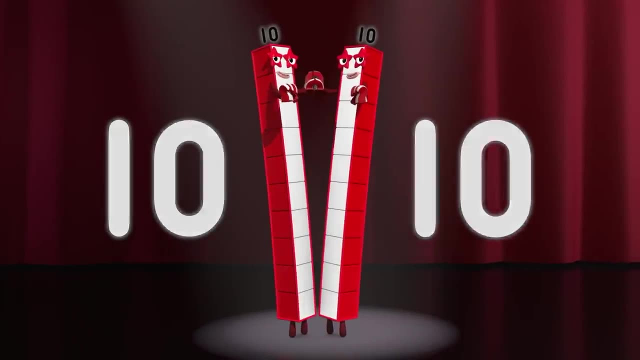 Drop to the floor and go round again. One, two, three, four, five, six, seven, eight, nine, ten. Two friends, two tens make twenty. One, two, three, four, five, six, seven, eight, nine, ten. 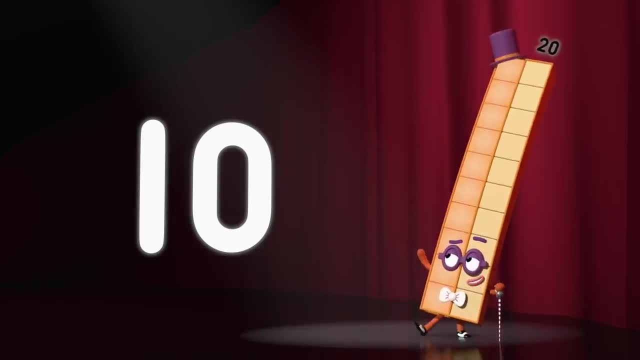 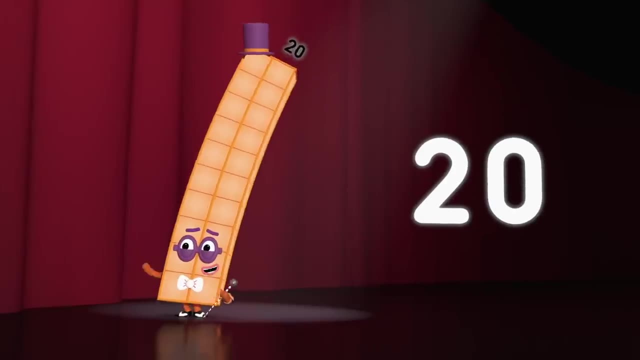 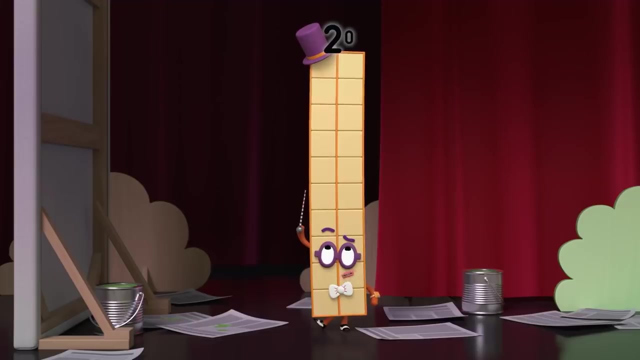 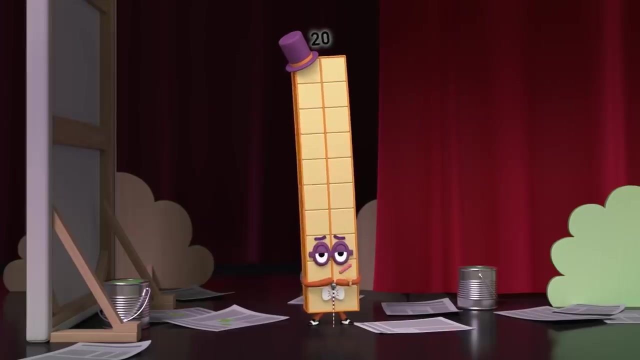 Halfway to twenty. Go round again. Eleven, twelve, thirteen, fourteen, fifteen, then Sixteen, seventeen, eighteen, nineteen, twenty, My two says I'm made of two tens, And who says I need any more? I say no more. That's how I'm created. 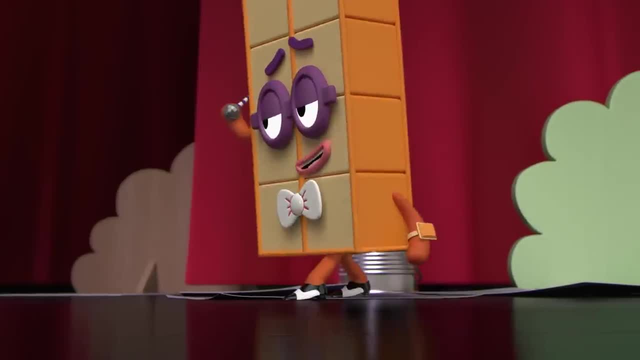 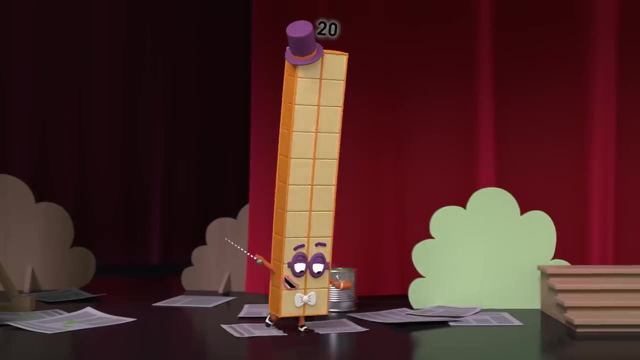 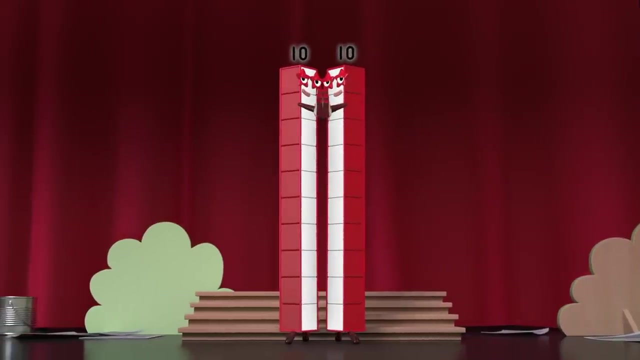 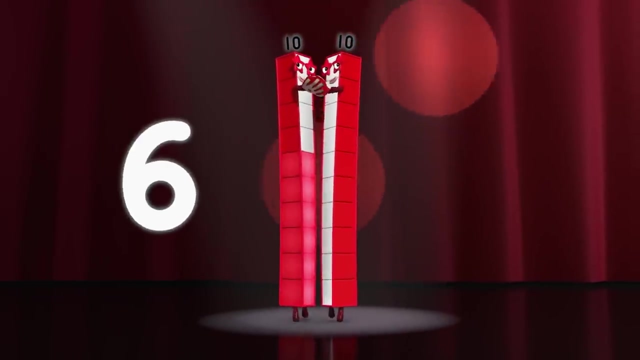 I'm perfectly weighted To move to the beat of a mambo, And then right on cue I can split into two And dance to the two tens tango One, two, three, four, five, six, seven, eight, nine, ten, Drop to the floor and go round again. 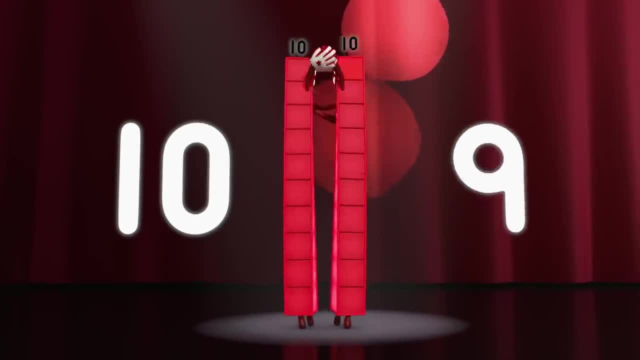 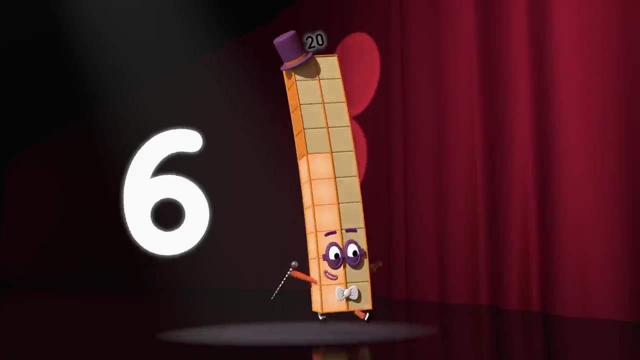 One, two, three, four, five, six, seven, eight, nine, ten. Two friends, two tens make twenty. One, two, three, four, five, six, seven, eight, nine, ten, Halfway to twenty. Go round again. 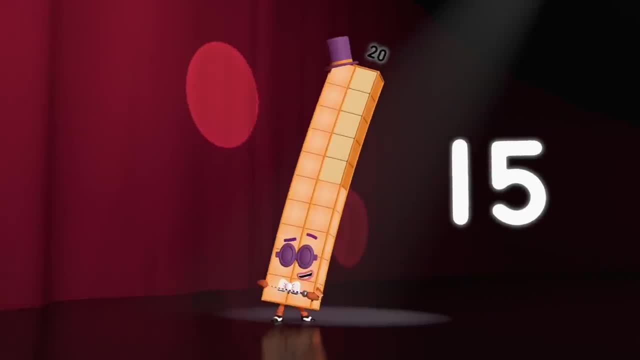 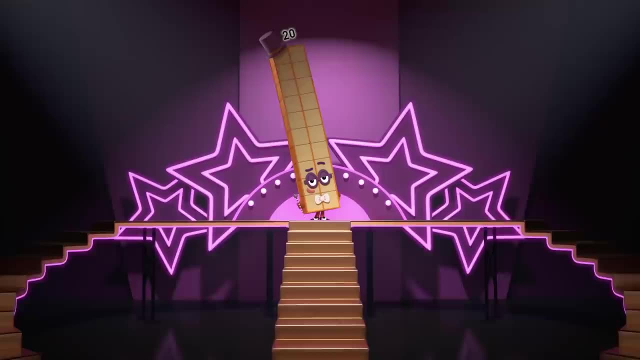 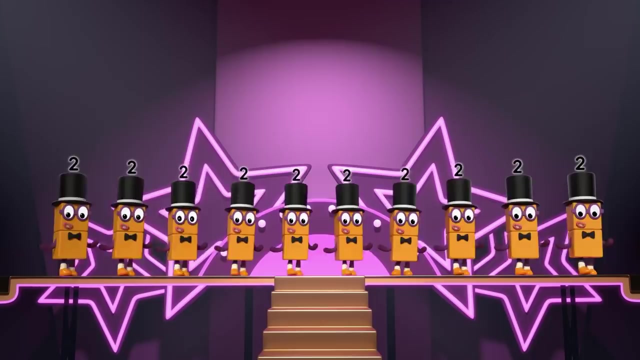 Eleven, twelve, thirteen, Fourteen, fifteen, then Sixteen, seventeen, eighteen, nineteen, twenty. I have some more friends I'd like you to meet. It's the ten twos hot shoe shuffle. Ten of us twos in a row. It's the ten twos hot shoe shuffle. 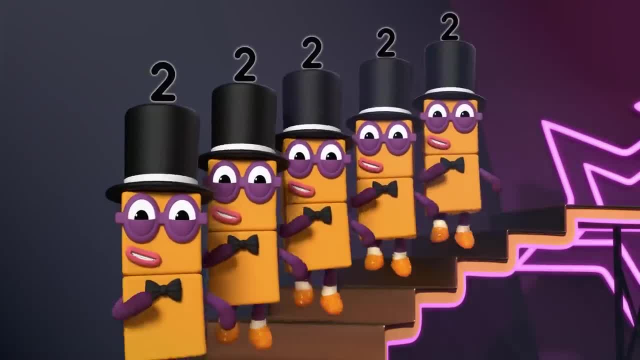 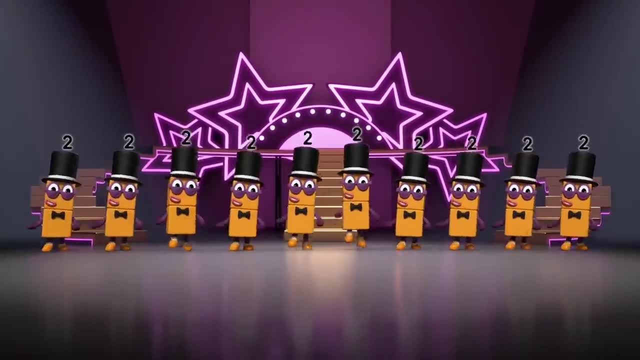 Welcome to the ten twos hot shoe show. We can shuffle to the beat, maybe shuffle our feet. People say your shuffling sure looks sweet. It's the ten twos hot shoe shuffle. Ten of us twos in a row. It's the ten twos hot shoe shuffle. 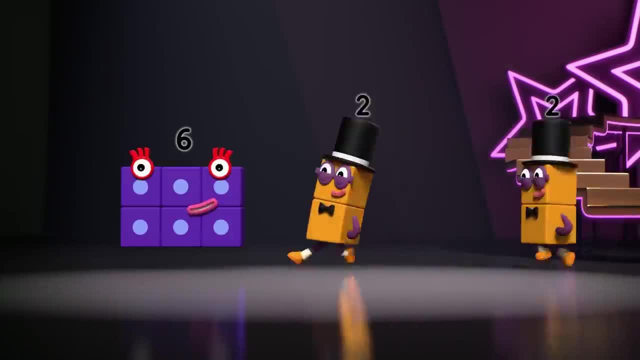 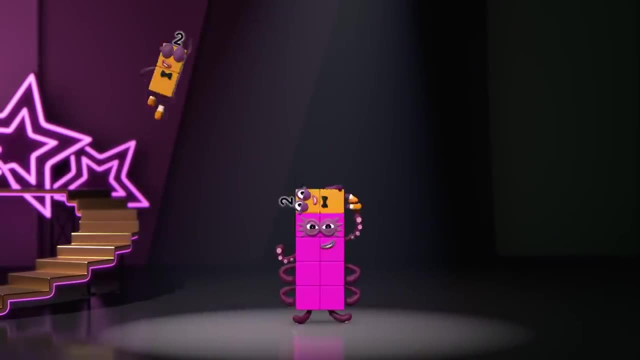 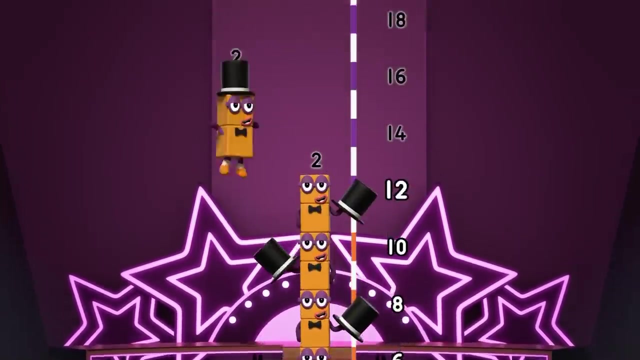 Wild words, but now it's time to go. Two, four, six, eight, ten, twelve, fourteen, sixteen, eighteen, twenty. Two, four, six, eight, ten, twelve, fourteen, sixteen, eighteen, Twenty. Two, four, six, eight, ten, twelve, fourteen, sixteen, eighteen, twenty. 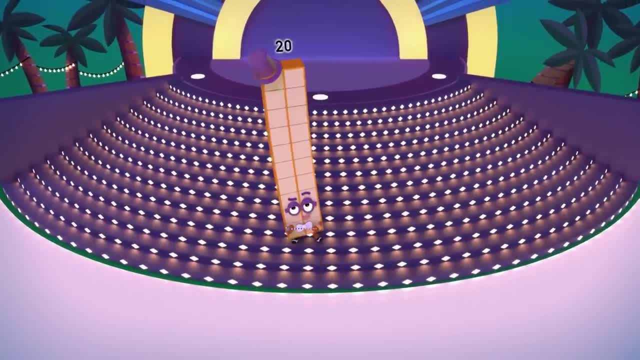 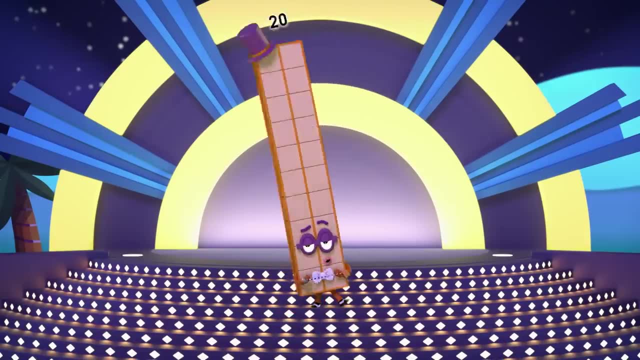 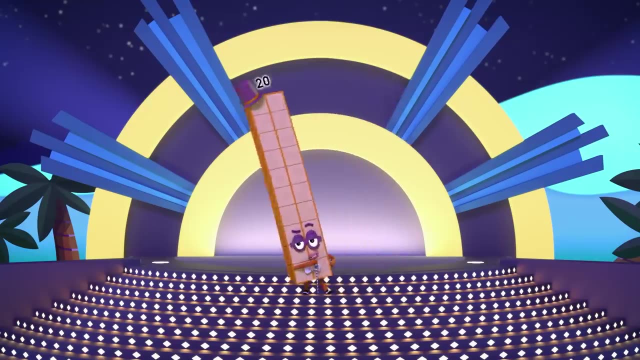 I'm 20 and I love to dance plenty of moves to my name. I'm tall and I'm slender. I'm graceful and tender. I sway as I do the fandango- Two tens, nothing more- as I take to the floor and dance to the two tens tango. 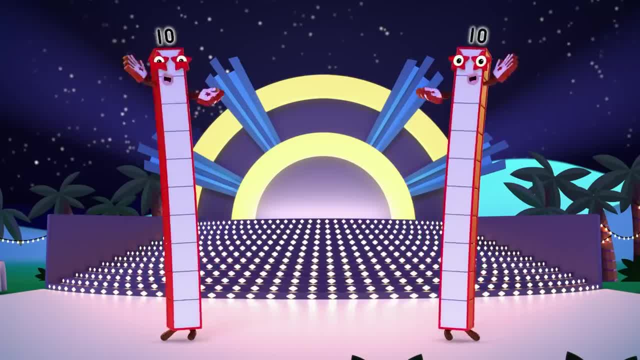 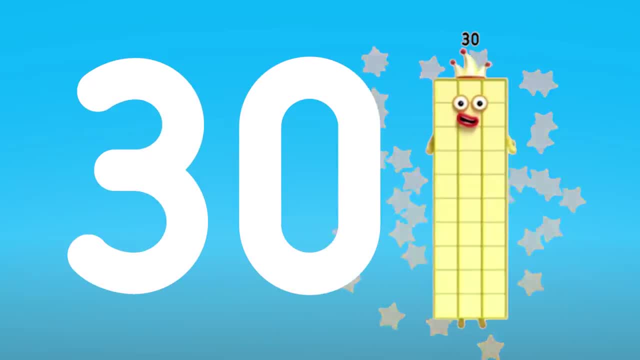 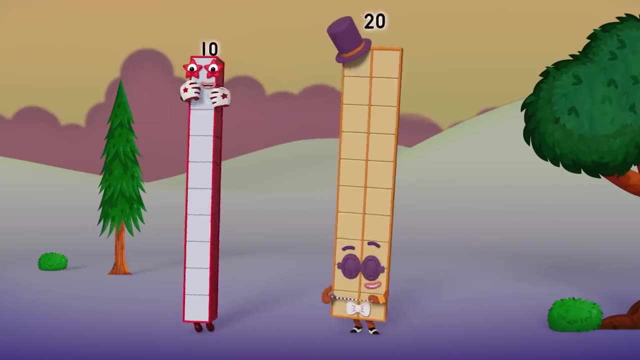 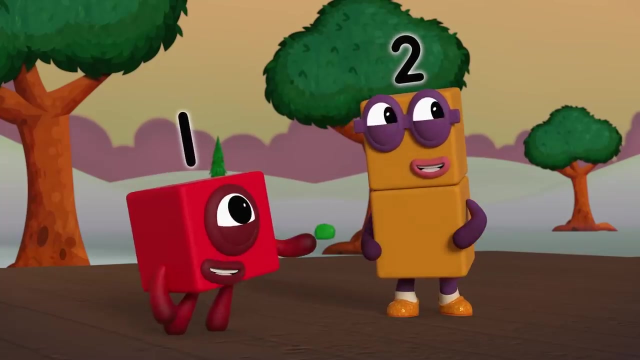 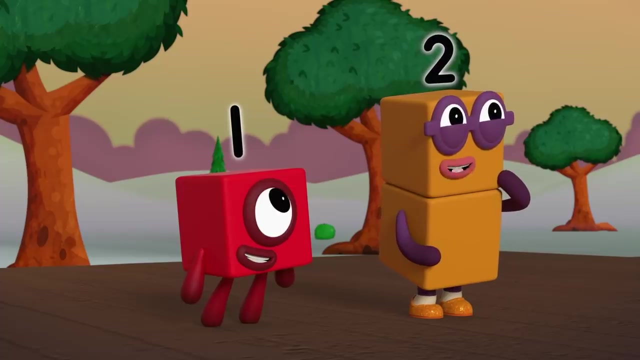 Two tens, nothing more, as we take to the floor and dance to the two tens tango. If I were bigger, maybe I'd be able to leap as high as you Ten. If I were bigger, maybe I'd be able to dance as well as you Twenty. 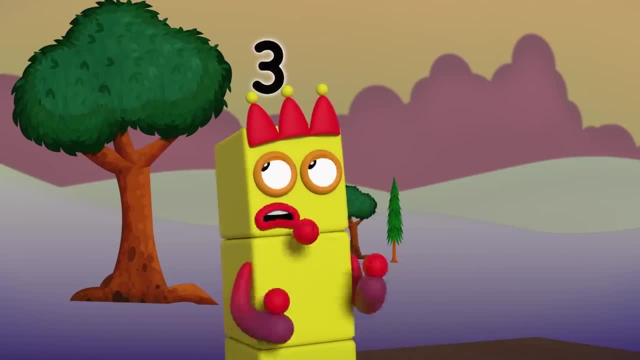 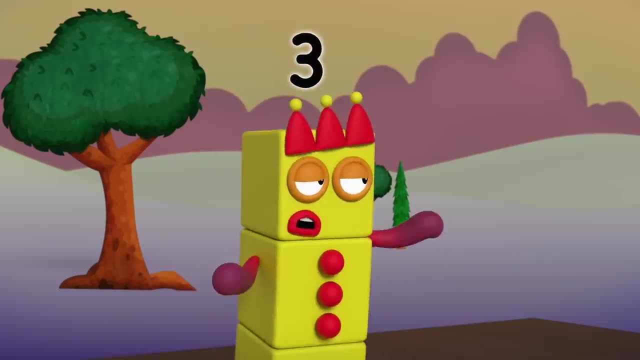 I don't want to be bigger. There's nobody in the world who's a better juggler than me. You know Three. there's someone you should meet, Huh, Who? Well, I'm one ten, And I'm Twenty. I'm 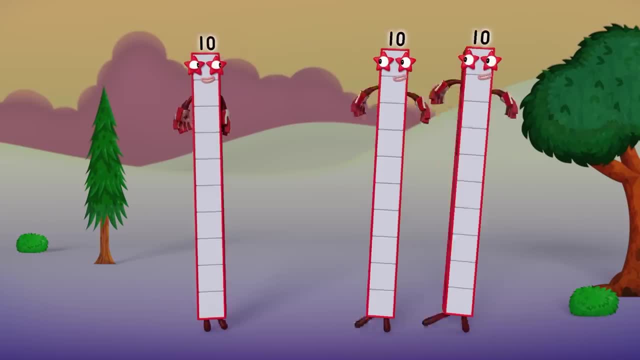 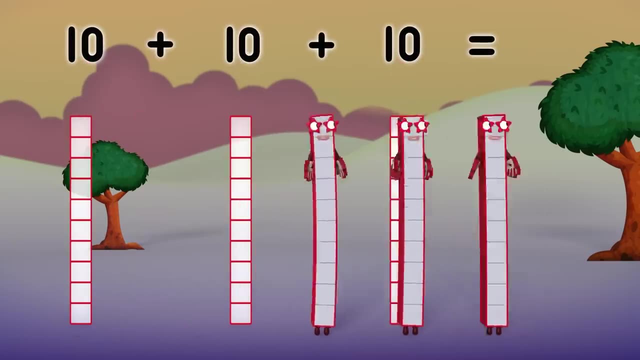 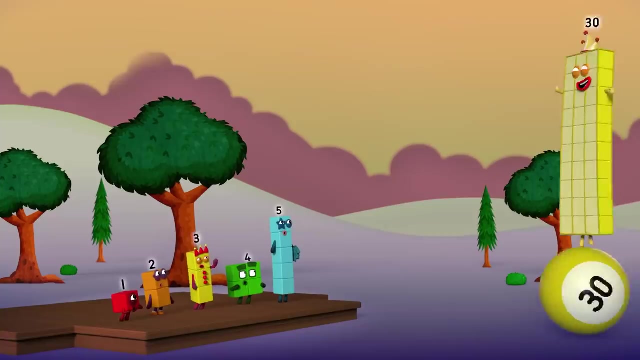 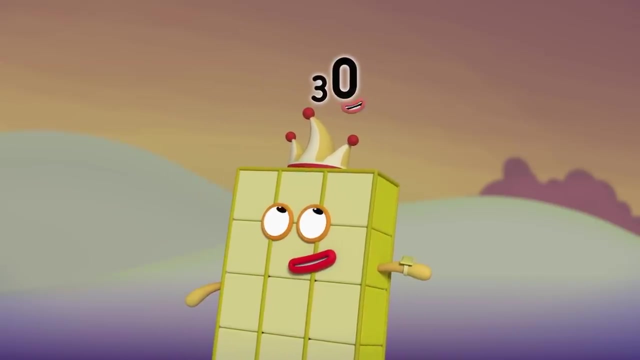 Two tens. Put us together, and what have you got? Three tens. Ten plus ten plus ten equals thirty. I am Thirty, the big entertainer. This Three stands for Three tens And nothing more. Oh, If you'd like to see more, then come to the circus. 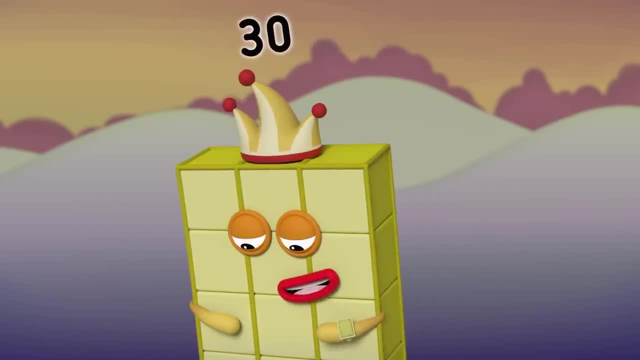 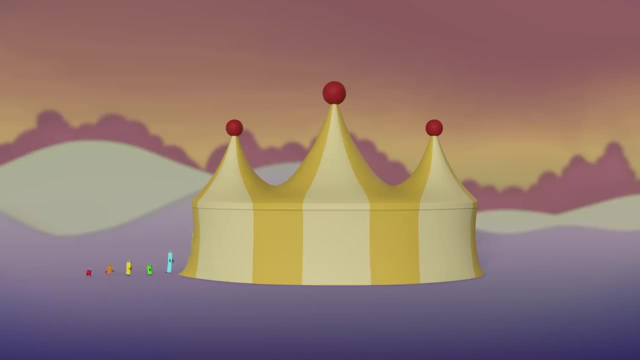 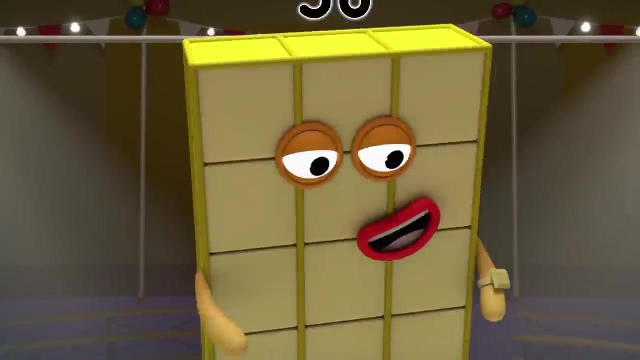 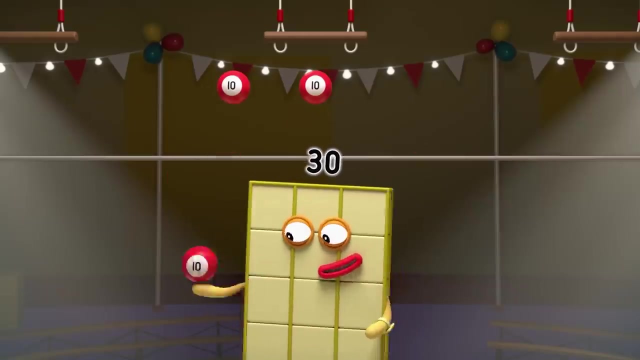 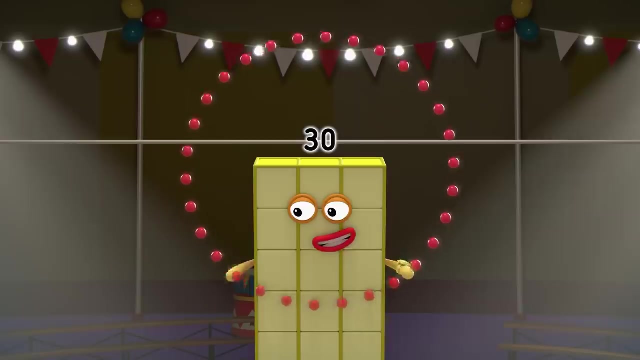 What circus. I like to keep it under my hat. Welcome to the big, big, Big big shop. Oh, Three tens are ten, twenty, thirty, Thirty balls. That's big. Wait, there's more. I'm three tens, Which means I'm also. 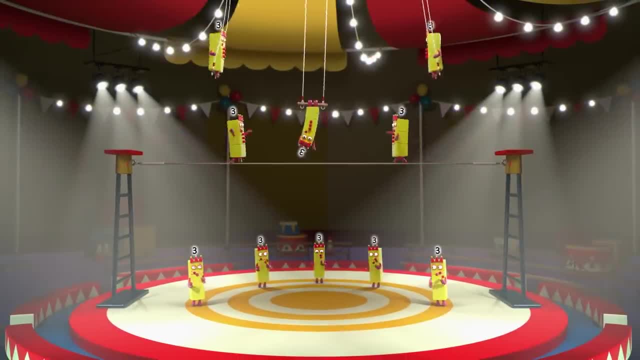 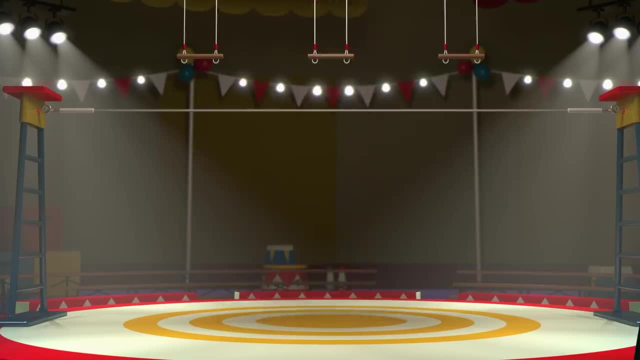 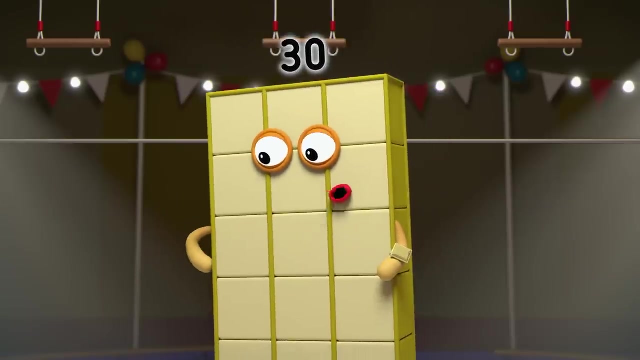 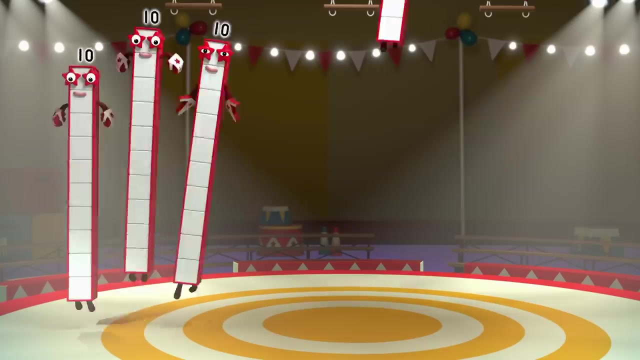 Ten, threes, four, Wow, Jus, Wow, If you like that, you're going to love this next act, for which we need another ten, Woo-hoo, Four tens. Put it together and what have you got? 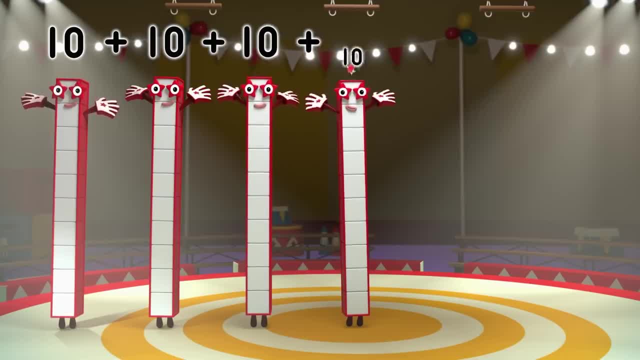 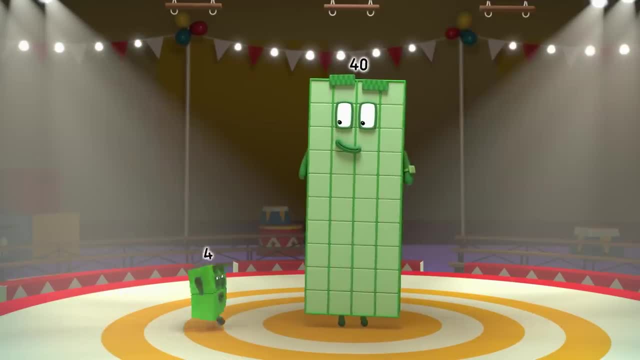 Ten plus ten plus ten plus ten equals Forty. I am forty and I'm a big squirrel. Oh, you're not a square. Oh, no, I am not, I'm a rectangle. I love rectangles. Would you like to see my collection? 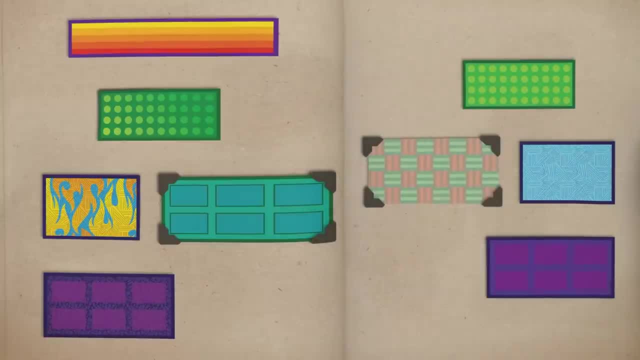 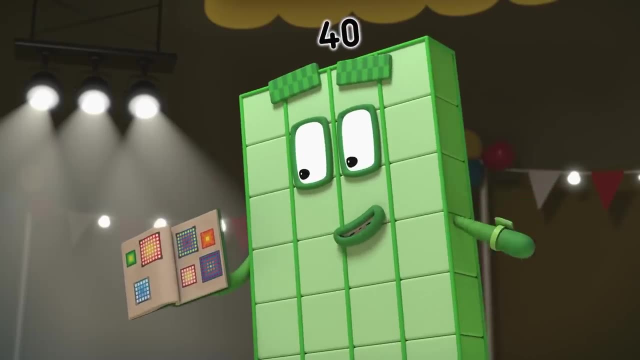 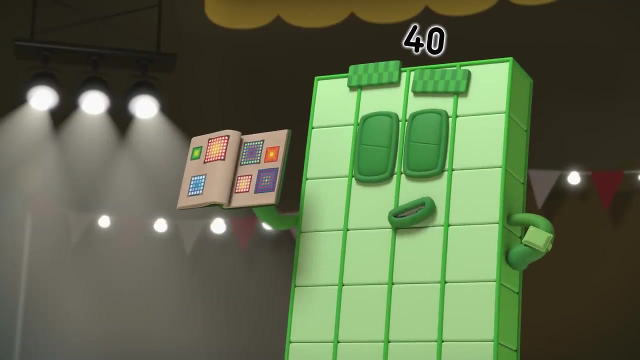 I've got loads of different ones: Tall ones, wide ones, I've even got square ones. Huh, Squares are a special kind of rectangle, you see, where all four sides are the same length, And a rectangle that's not a square is called an oblong. 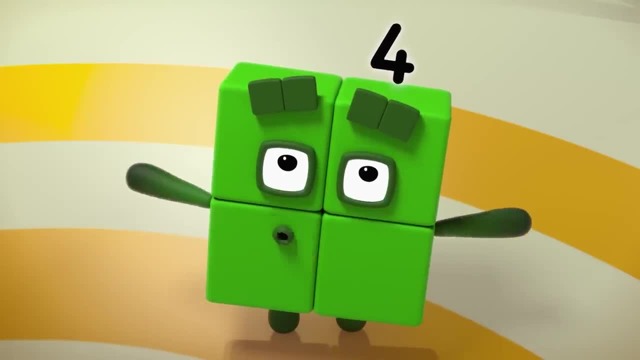 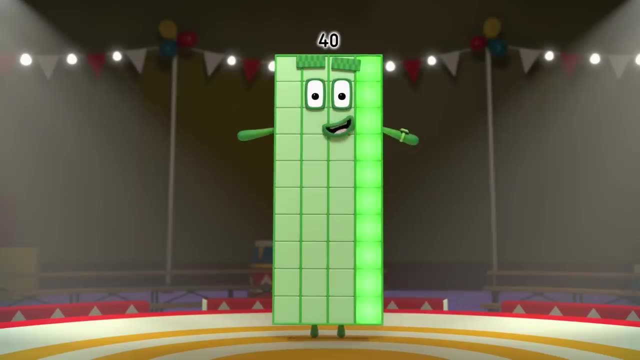 Ooh, I'm a special rectangle, But if it's squares, you want it's squares, you're going to get. I'm forty, I'm four tens, Which means I'm also Ten fours. Yay, With ten strong squares, you can really 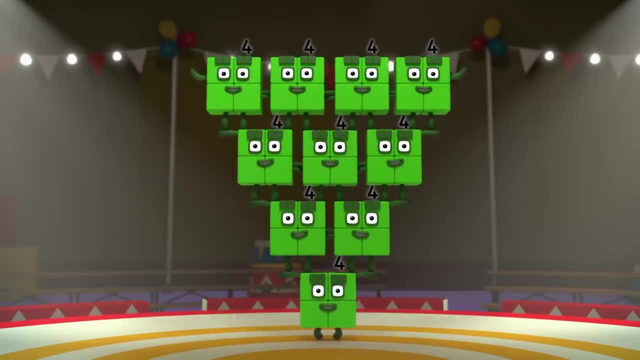 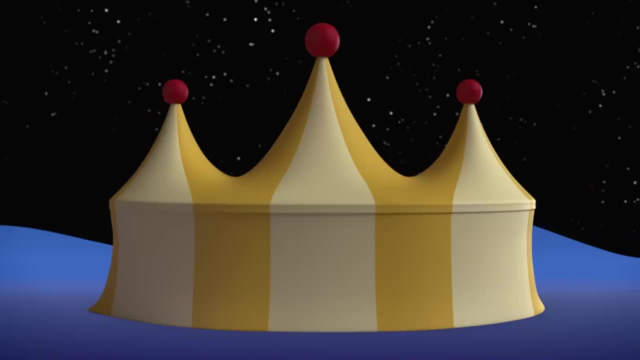 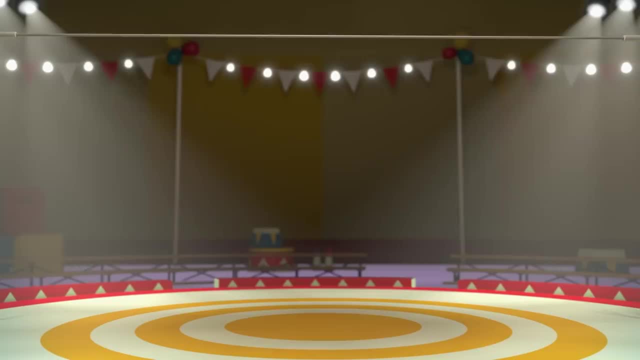 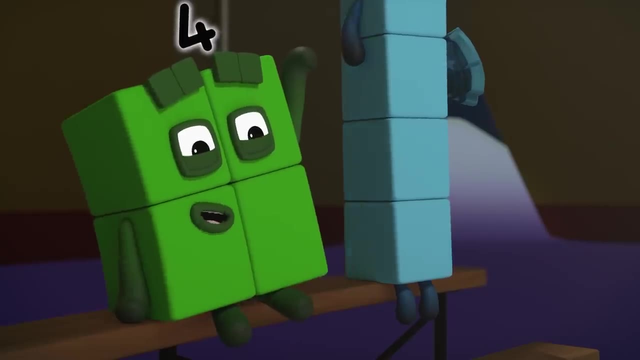 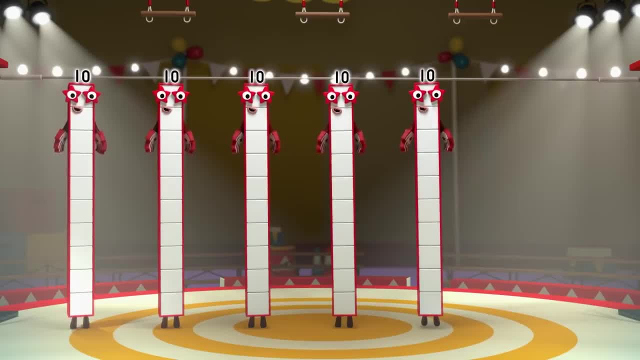 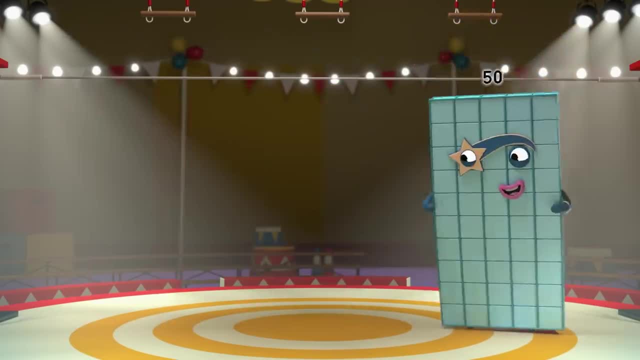 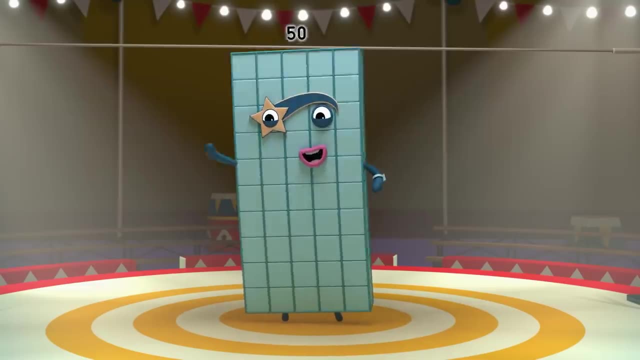 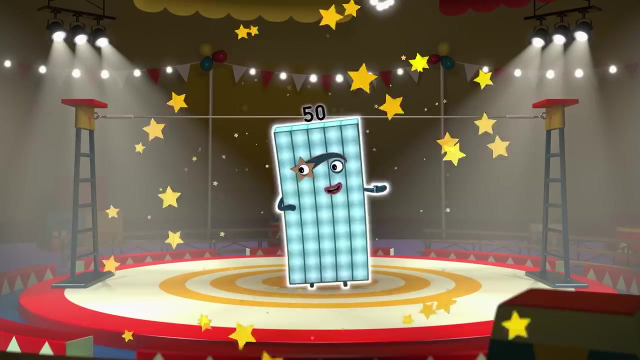 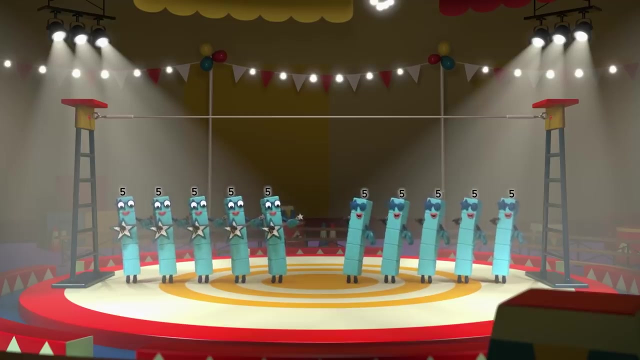 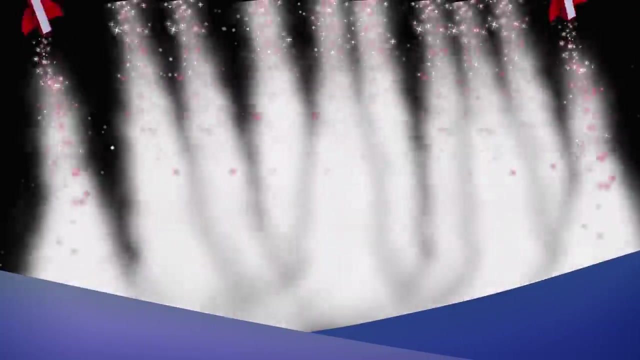 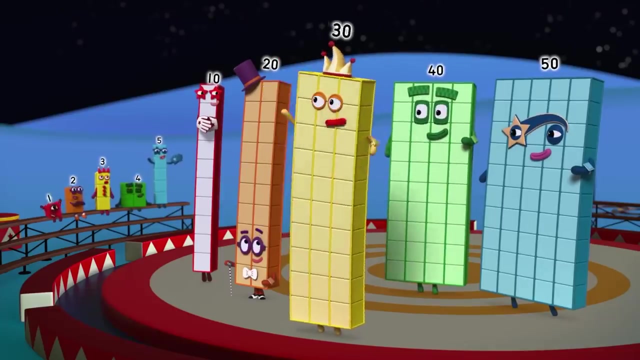 Wow Για Hi-five, Hi-five, Hi-five, Hi-five, Hi-five, Hi-bye. Wow, Hi-bye. All right, I'm 510, which means I'm Now. that's what I call a showstopper. 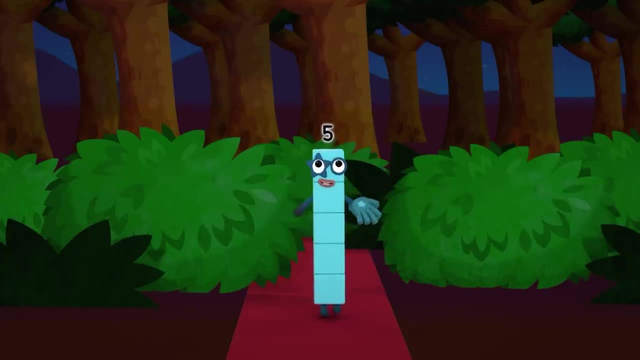 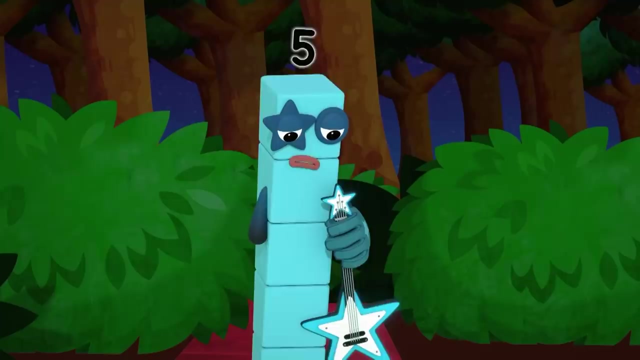 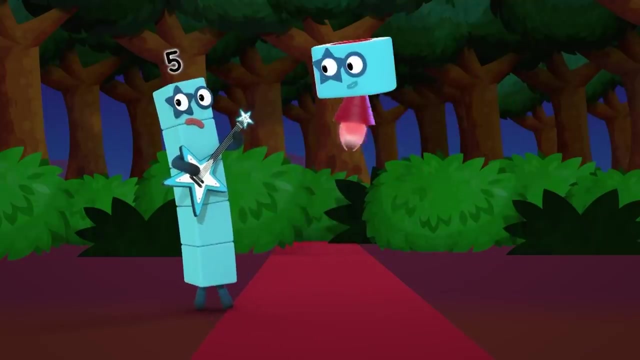 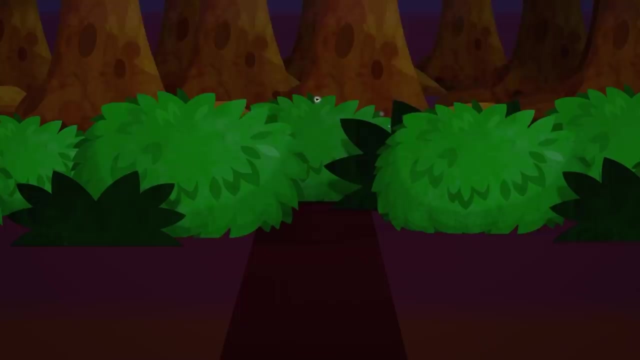 Wow, that's here. That's a real, the Tower of Rock. Yeah, but am I good enough? Yes, of course you are. You've got talent, You've got drive and you never give up. It runs in the family, the family Five Rock. 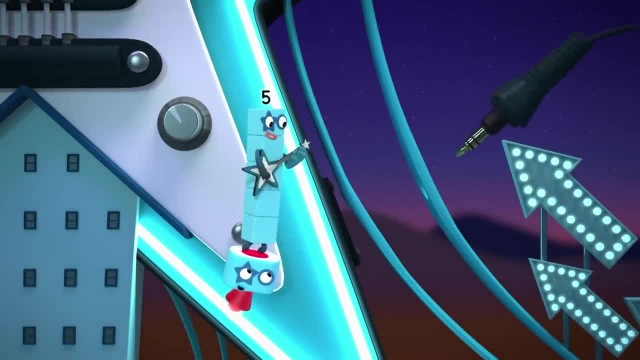 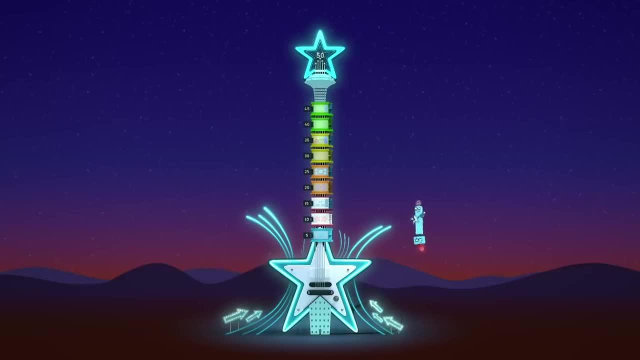 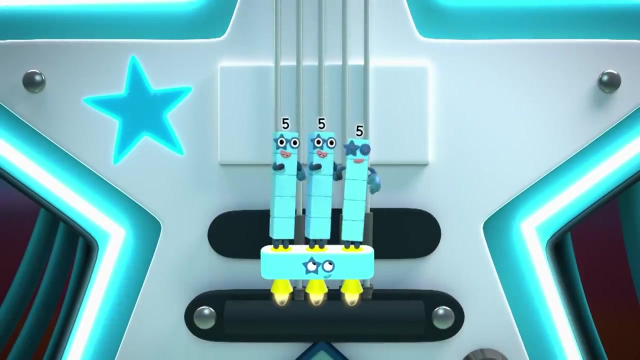 Crack it up, Plug in the cable. I'm the one and only five times table. It's time to come alive and meet your heroes, Some of them and in five and some and in zero. One five is five, two fives are ten. three fives are fifteen. 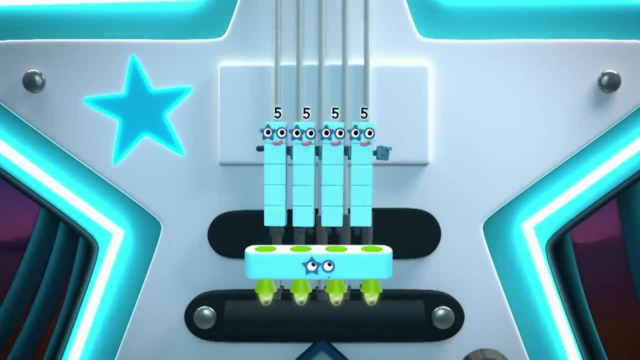 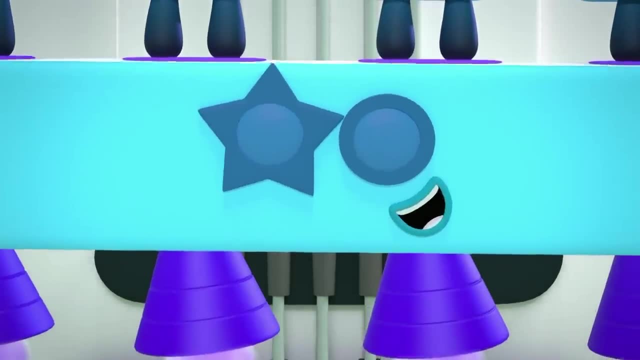 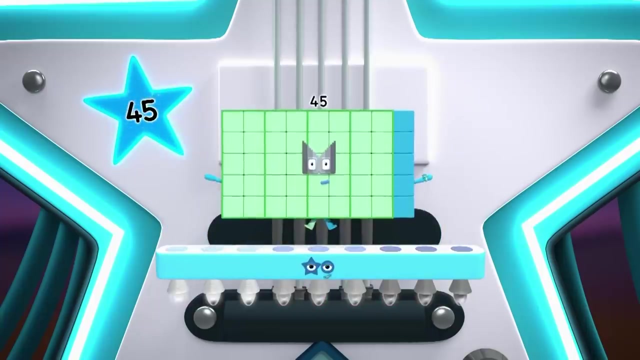 Trust me, You'll go far. Four fives are twenty. five fives are twenty-five. six fives are thirty. You know who you are. seven fives are thirty-five. eight fives are forty. nine fives are forty-five. And here's the next big superstar: ten fives are fifty. 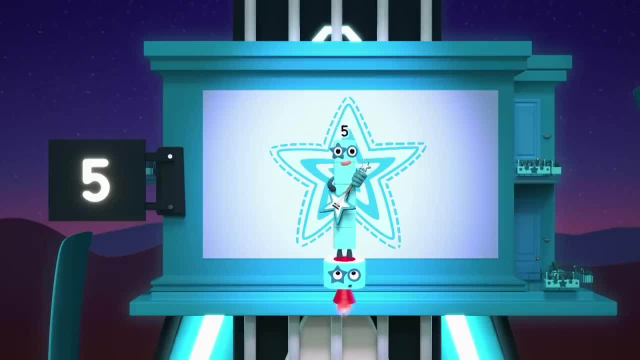 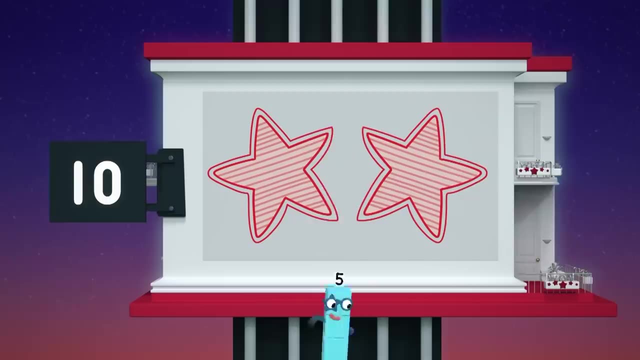 Take it to the top One, five will land her hands. She's the leader of the band. five high five. Two fives can take a trip. They can make a rocket ship. Ten Lost all Cause I'm the five times table. Start me up and we'll go up in fives. 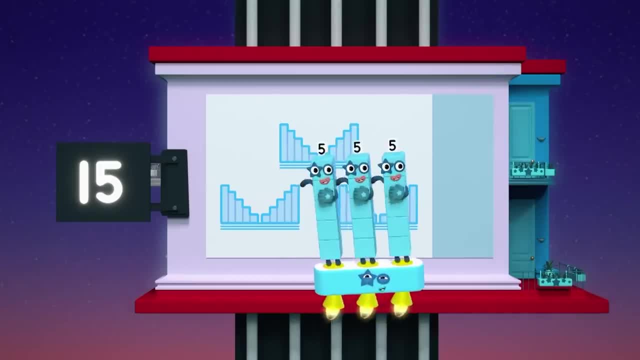 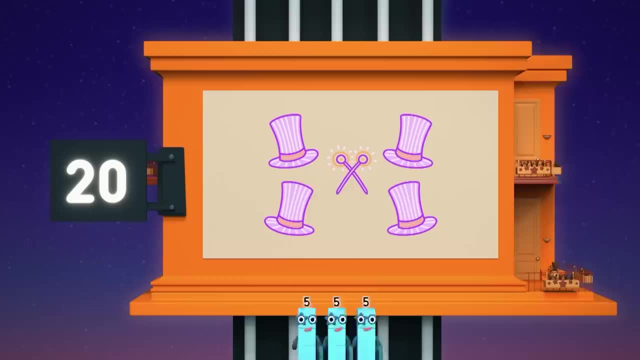 Three fives are slightly odd. They're a secret special squad. Fifteen, Hush, hush, Slightly odd. Four fives make a great quartet, But you ain't seen nothing yet. Twenty Chop, chop, chop, chop, chop, chop, Cause I'm the five times table. 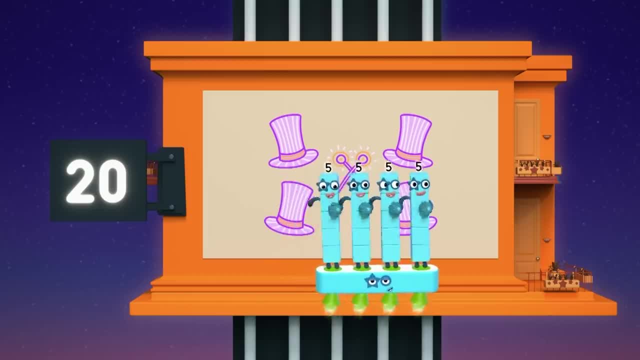 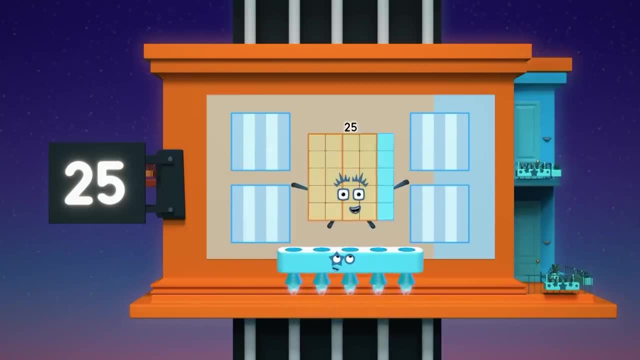 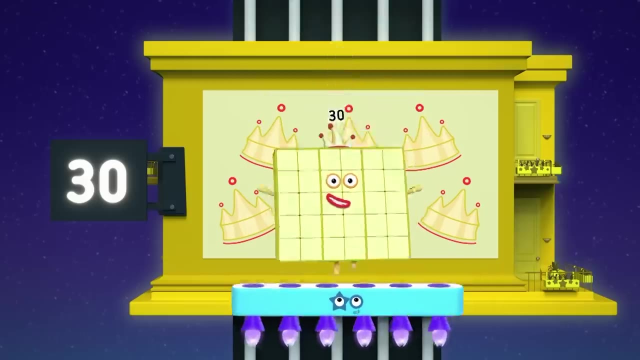 Stab me up and we'll go up in fives. Five fives are half way there. Five fives make a great big square. Twenty-five Square. Six fives are neatly stacked. Six fives are a circus act. Thirty, The greatest show in Numberland. 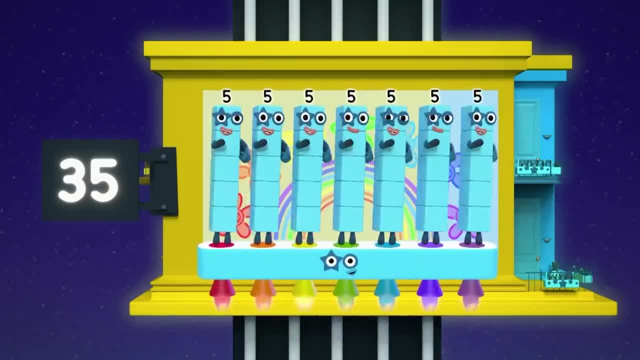 Seven fives never come unstuck. Seven fives have a great show in Numberland. Seven fives never come unstuck. Seven fives have a great show in Numberland Seven fives never come unstuck. Seven fives have sevens left Thirty-five. 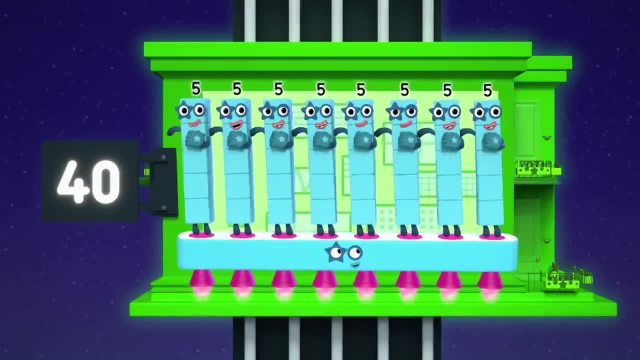 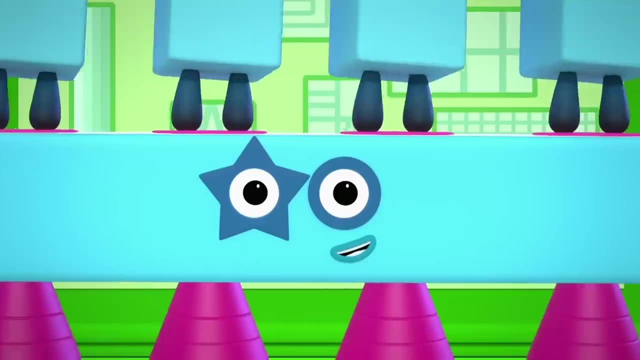 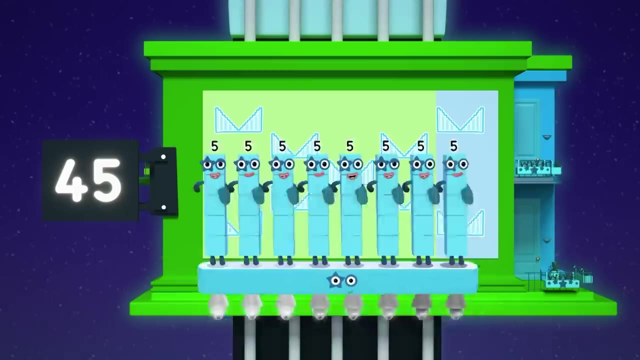 She's the five times table. Eight fives will get them bigger. They make an impressive figure. Forty, She's the five times table. Cause I'm the five times table. Start me up and we'll go up in fives. Nine fives to step up the pace. 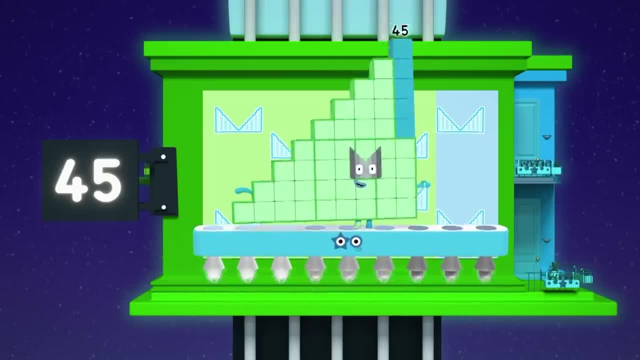 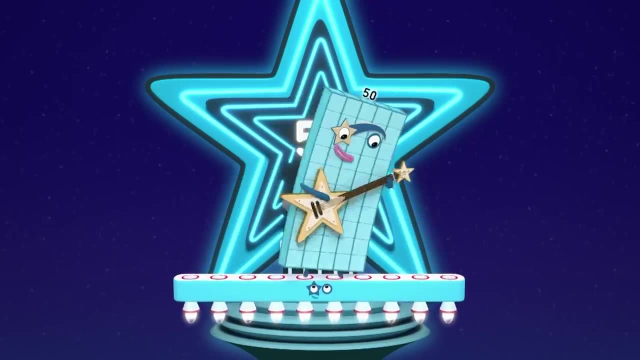 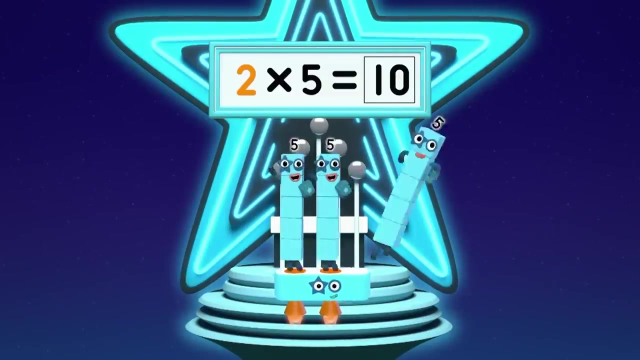 And take you to a higher place. Forty-five, Ten fives with a gold guitar. Ten fives with a gold guitar. Ten fives make a superstar. Fifty High. fifty One five is five. Two fives are ten. Three fives are fifteen. Trust me, you'll go far. 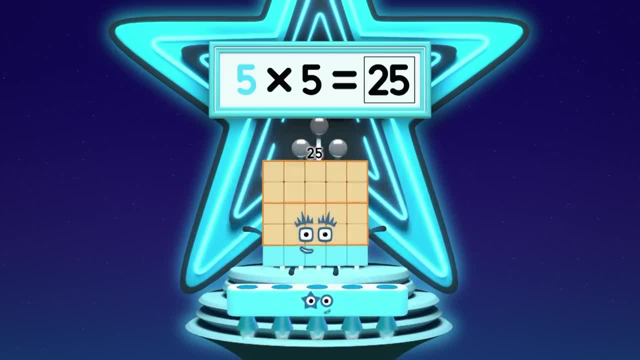 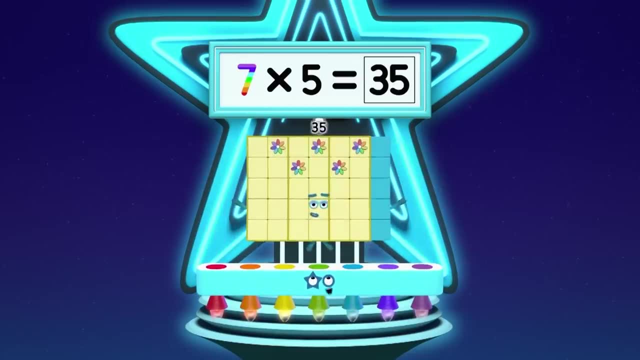 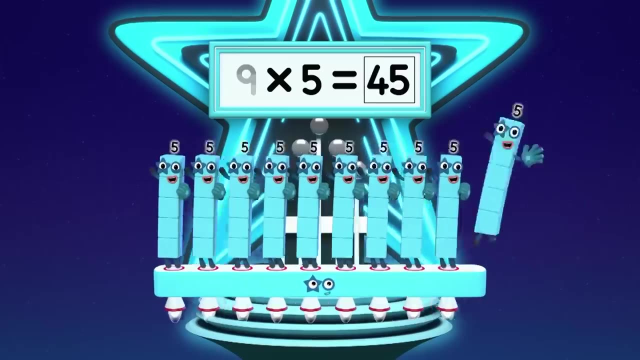 Four fives are twenty. Five fives are twenty-five. Six fives are thirty. You know who we are. Seven fives are thirty-five. Eight fives are forty. Nine fives are forty-five, Forty-five. Here's the next big superstar. Ten fives are fifteen. 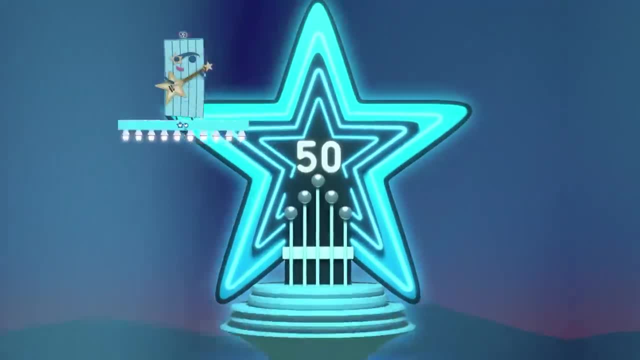 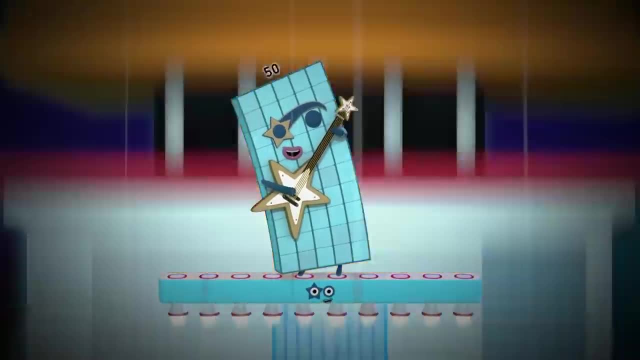 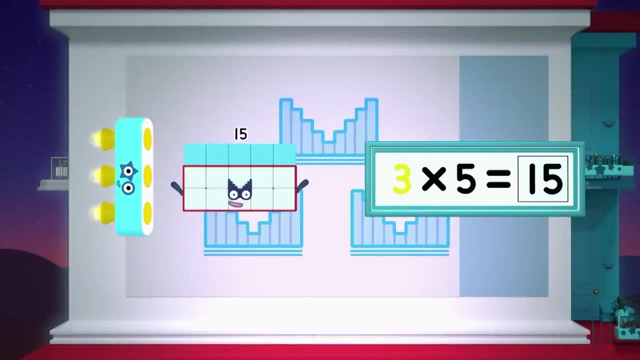 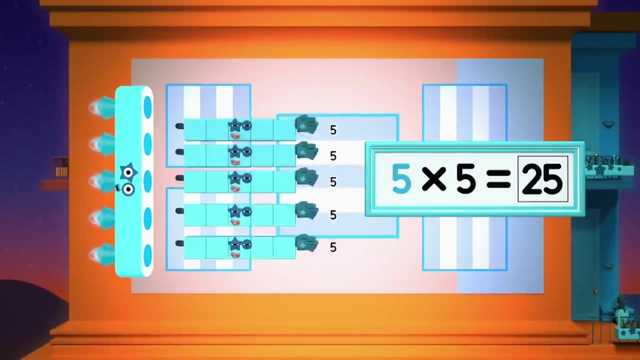 Fifty Guitar solo Sideway: One five is five, Two fives are ten. Three fives are fifteen. Trust me, you'll go far. Four fives are twenty. Five fives are twenty-five, Six fives are thirty. You know who we are. Oh, oh, oh. 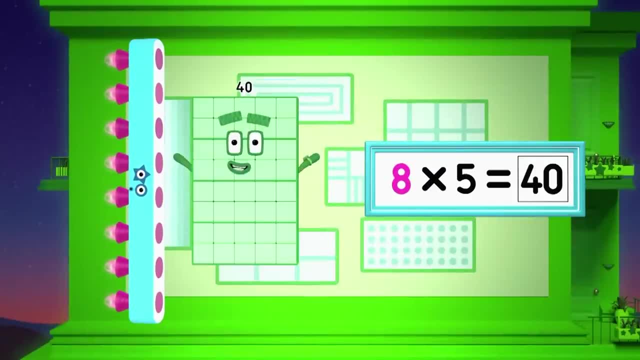 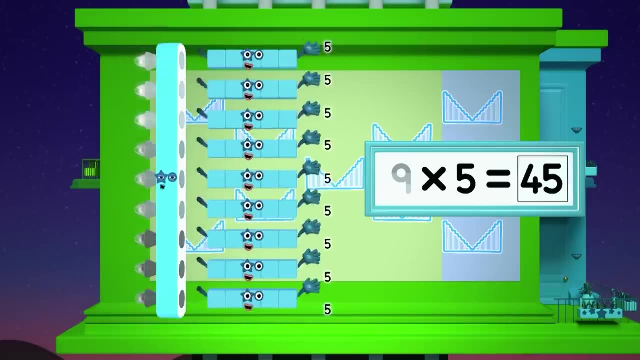 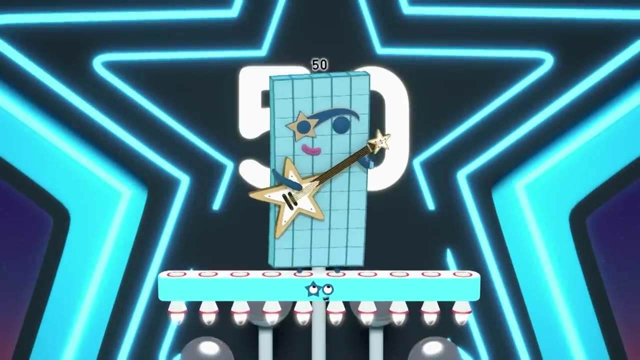 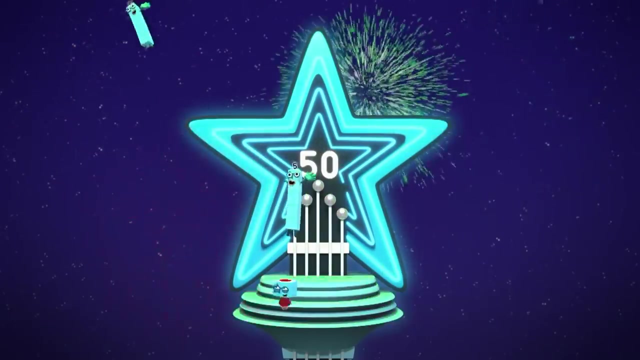 Seven fives are thirty-five. Eight fives are forty. Nine fives are forty-five. One more time, let's take it to the top. He's the star of the show. Ten fives are fifty. Rock and roll Guitar solo. Oh yes, high-five. 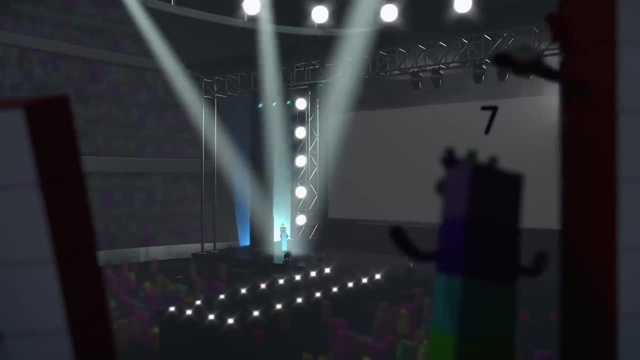 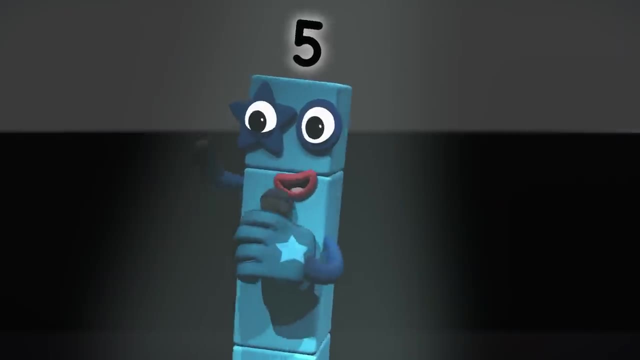 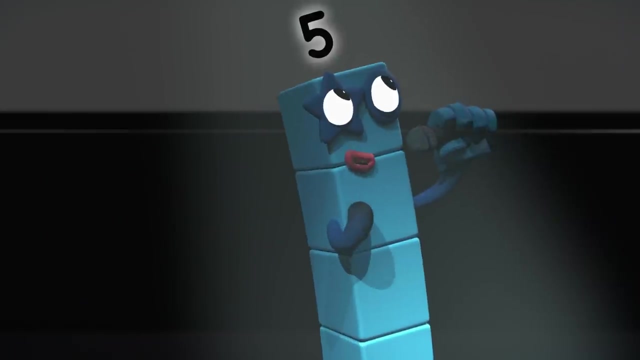 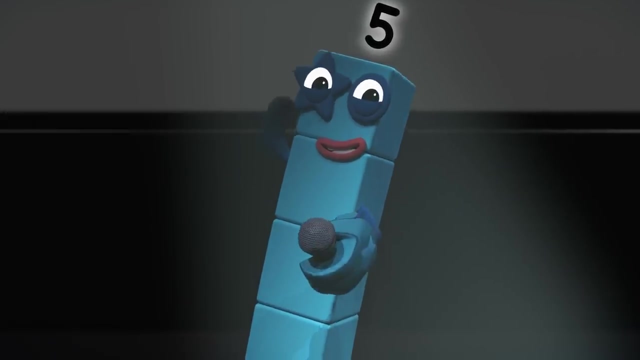 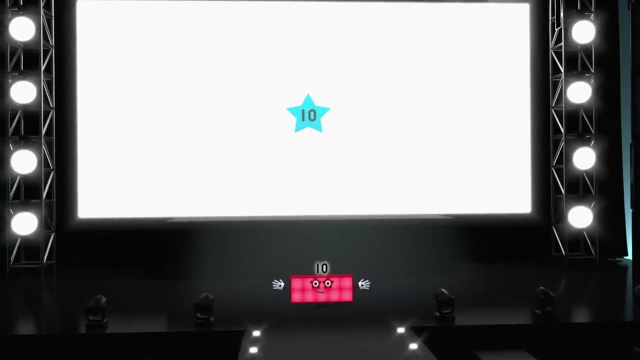 Yay, Testing, testing One, two, three, four, five. Hello Numberland, I'm a rock star, But are you ready to meet a super star With a little help from my friends? Five, Ten, Fifteen. 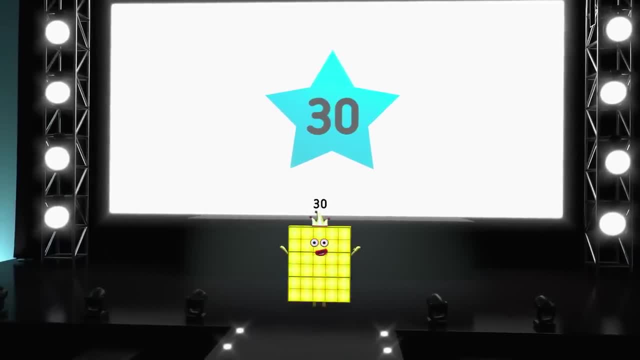 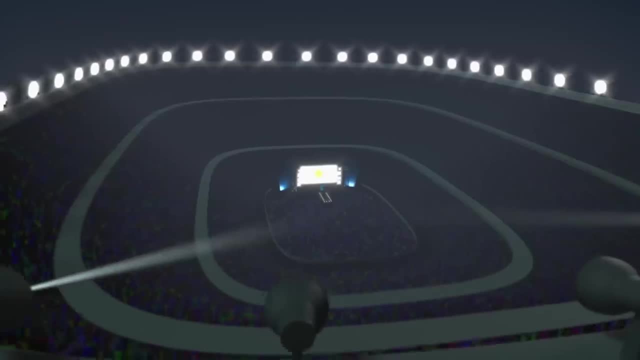 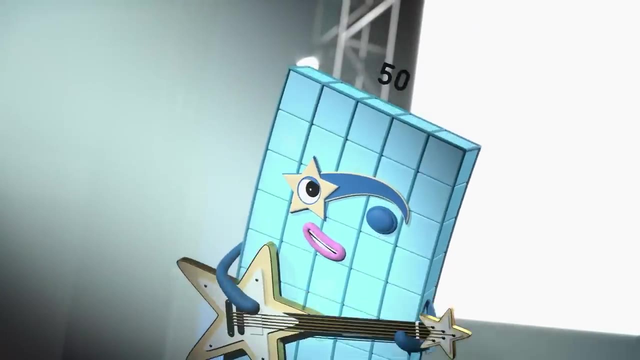 Twenty, Twenty-five, Thirty, Thirty-five, Forty, Forty-five And fifty, Let's rock. My name is Phyllis. I'm a rock and roll superstar. I'm all the rage when I take the stage with my shining gold guitar. 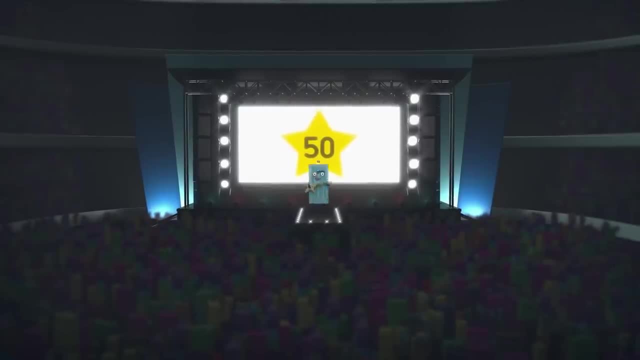 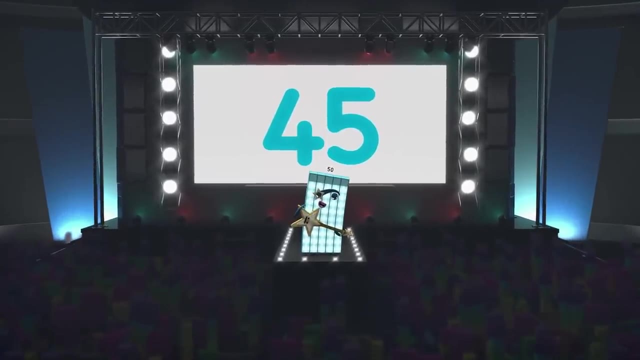 And so you don't forget my name. I play this counting game in five, Five, ten, fifteen, twenty, twenty-five, thirty, thirty-five, forty, forty-five And fifty- I'm fifty. Ten hands, Ten big hands. 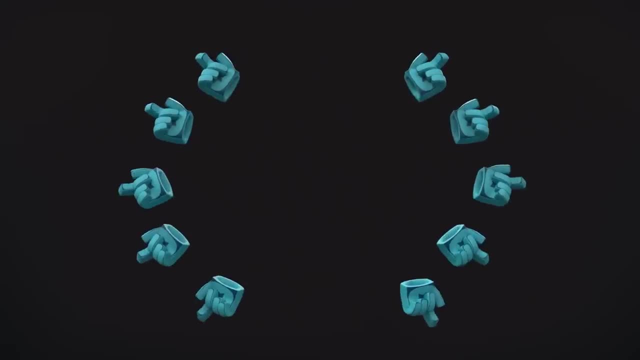 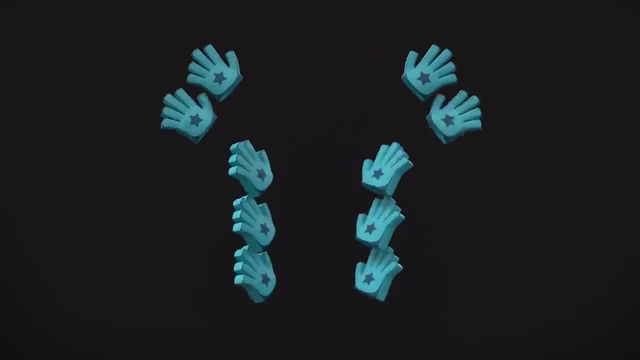 Flying through the air. Count the fingers super quick. A little bit of flair. Five fingers on each hand, High five, Five, ten, fifteen, twenty, twenty-five, thirty, thirty-five, forty, forty-five And fifty, Fifty fingers. 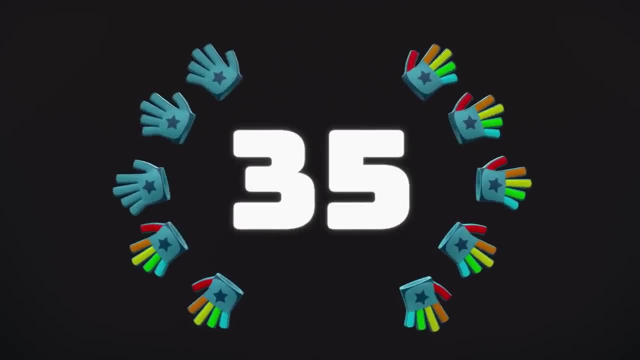 My name is Fifty. I'm a rock and roll superstar. I'm all the rage when I take the stage with my shining gold guitar, And so you don't forget my name. I play this counting game in five. Five, ten, fifteen, twenty, twenty-five, thirty, thirty-five, forty, forty-five. And so you don't forget my name. I play this counting game in five. Five, ten, fifteen, twenty, twenty, twenty-five, thirty-five, thirty-five, forty-five. And so you don't forget my name. I play this counting game in five. 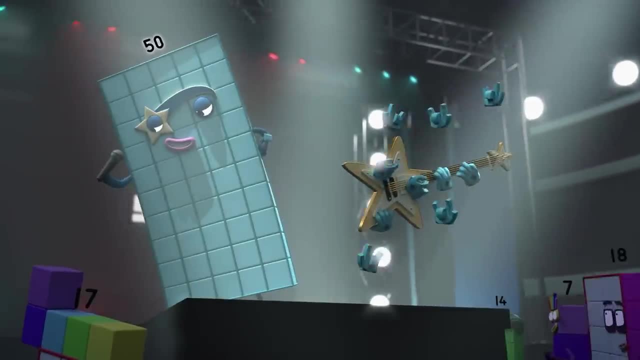 Five, ten, fourteen, fifteen, twenty-five, thirty-five, forty, forty-five And fifty. I'm fifty. Fifty fingers. My name is Fifty. I'm a rock and roll superstar. I'm all the rage when I take the stage with my shining gold guitar. 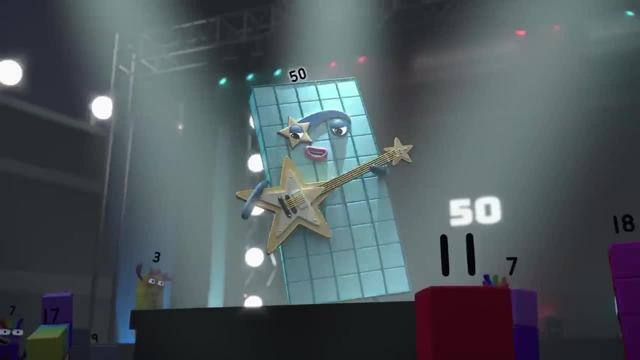 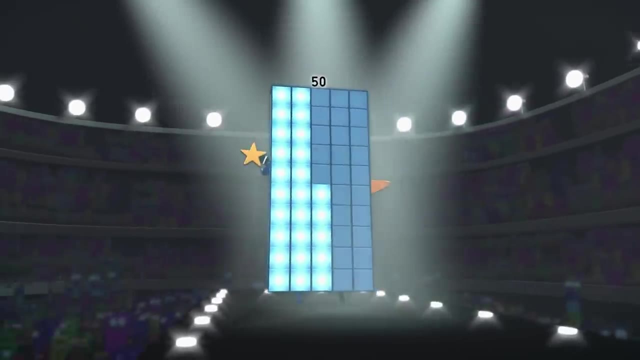 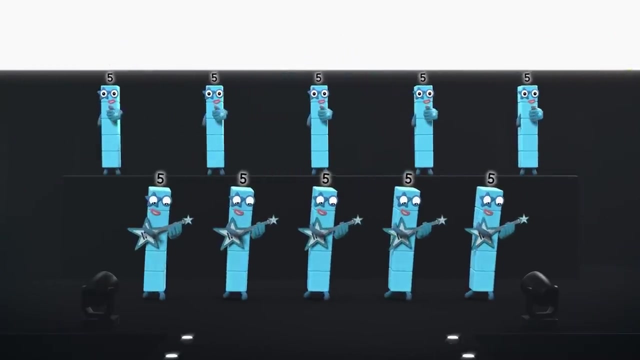 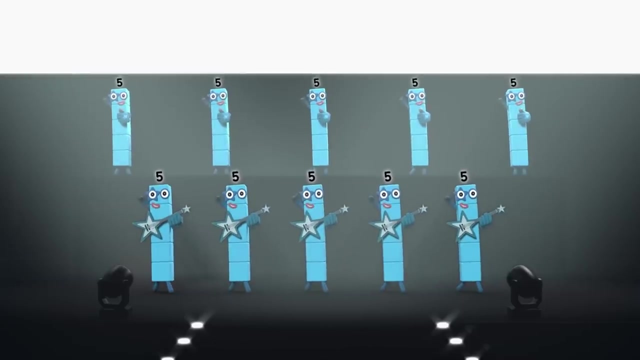 And so you don't forget my name. I play this counting game in five, Five, ten, fifteen, twenty, twenty-five, thirty, thirty-five, forty, forty-five And fifty. I'm Fifty, Ten, five, ooh. 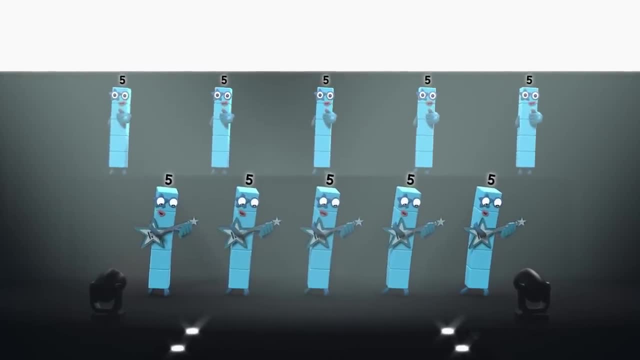 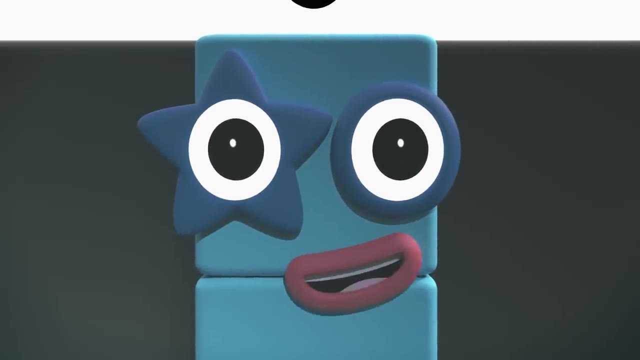 Ten, five, ten rockers rocking out in style, Five blocks on each of us jumping in a pile. Sea dive Five: 10, 15,, 20,, 25,, 30,, 35,, 40,, 45.. 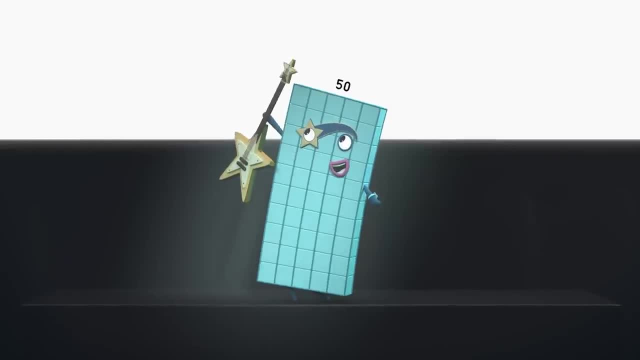 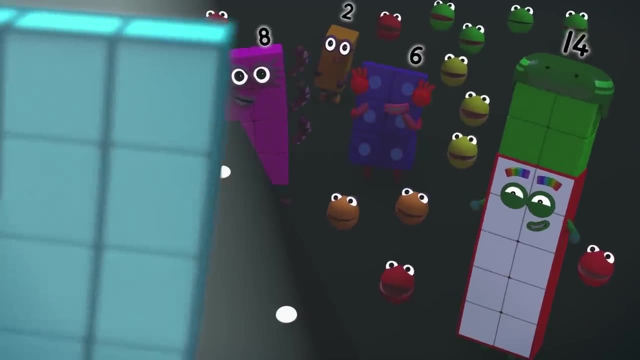 And 50,, 50 blocks. My name is 50.. I'm a rock and roll superstar. I'm all the rage when I take the stage with my shining gold guitar, And so you don't forget my name. I play this counting game. 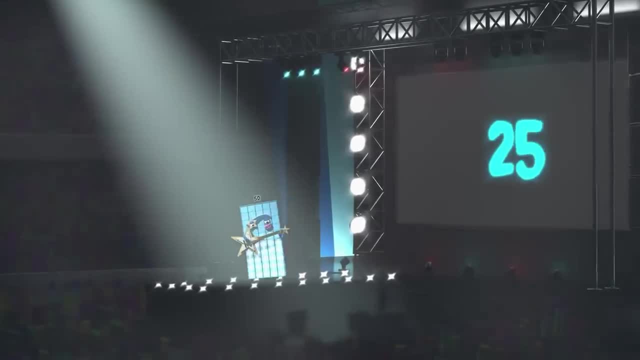 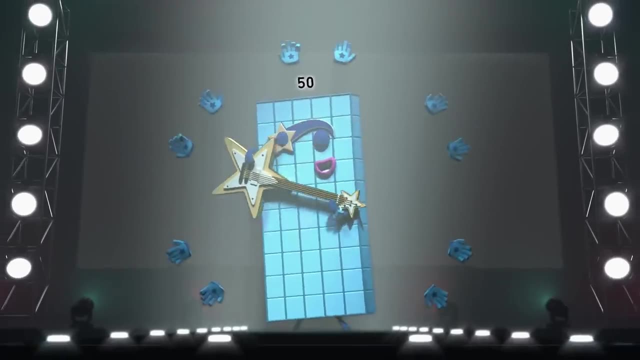 Come on Five: 10,, 15,, 20,, 25,, 30,, 35,, 40,, 45. And 50. I'm 50, everybody, Ten, five, 50. I feel alive. 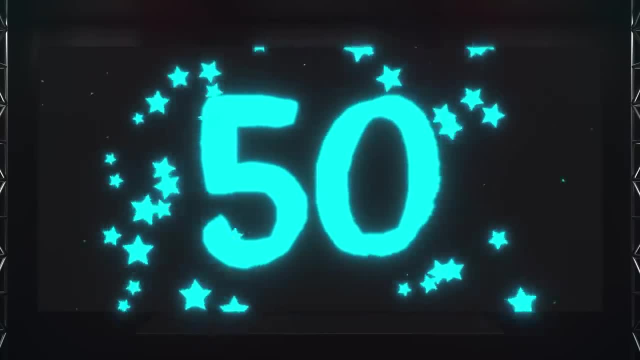 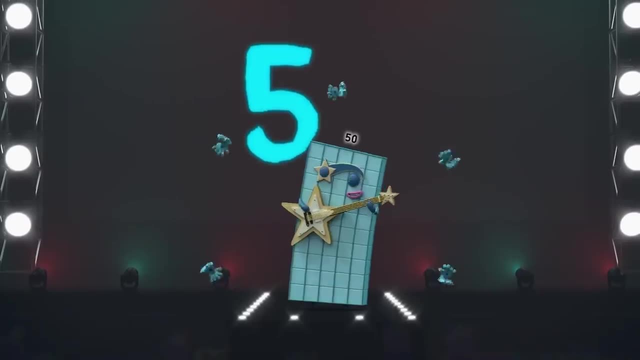 50.. A five and a zero 50.. Who's your hero? 50.. Five, 10.. 50.. Say it again: 50.. A five and a zero 50.. Who's your hero? 50.. 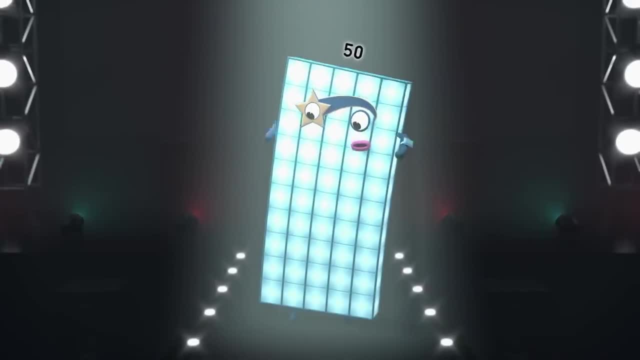 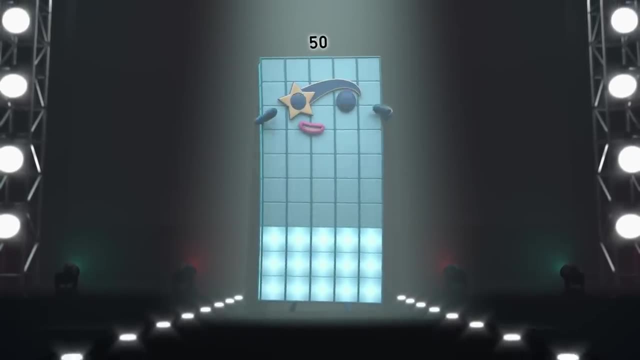 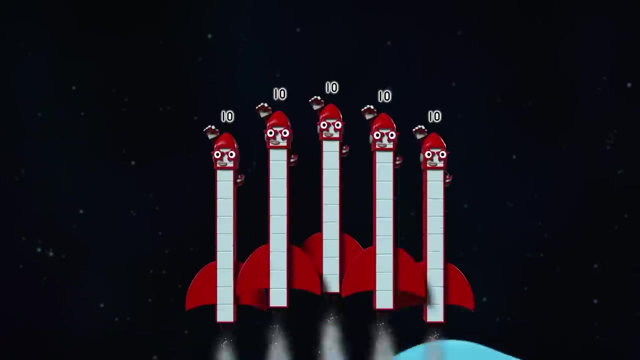 50,, 50,, 50.. 50,, 45,, 40,, 35,, 30,, 25,, 20,, 15,, 10,, 5.. Last shot: Five: 10, five rockets shooting into space. 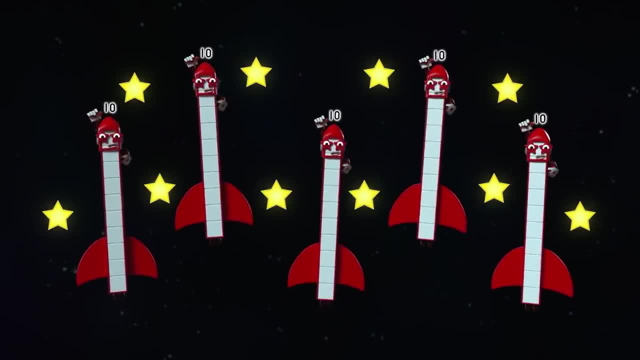 We can count the points on all the stars before heading: 5, 10,, 15,, 20,, 25,, 30,, 35, 40,, 45. And 50.. 50 shining points: 5, 10,, 15,, 20,, 25,, 30,, 35,, 40, 45. 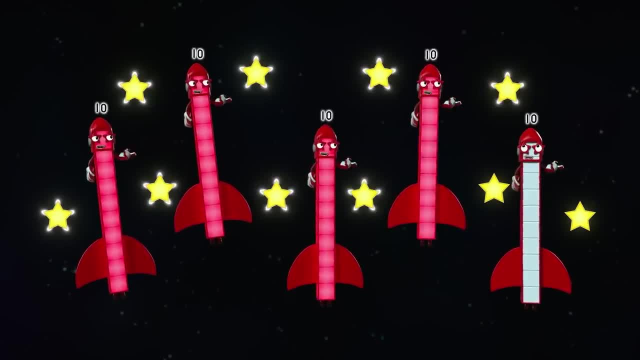 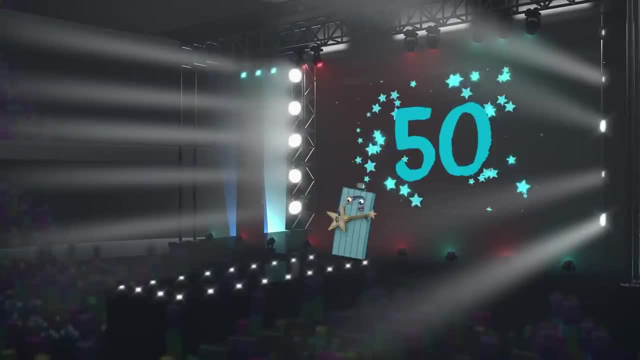 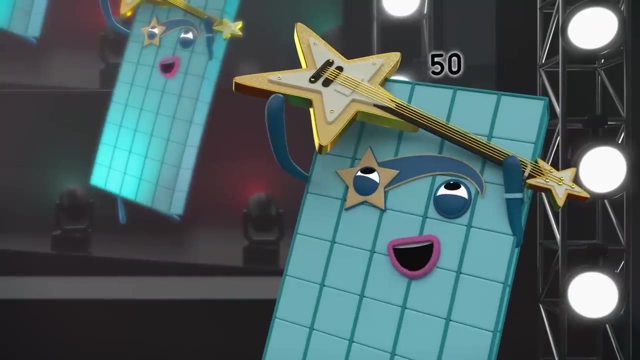 And 50.. 50 shining points. My name is 50.. I'm a rock and roll superstar. I'm all the rage when I take the stage with my shining gold guitar, And so you don't forget my name. I play this counting game. 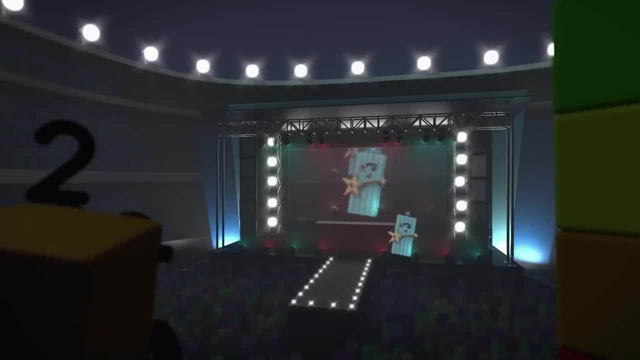 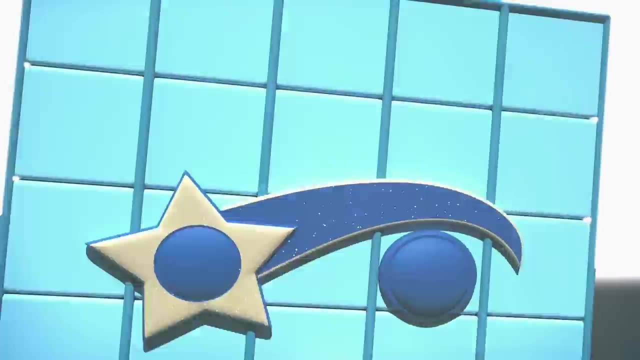 Let me hear you: 5, 10.. 15,, 20,, 25,, 30,, 35,, 40,, 45,, 40. And 50.. 20,, 25,, 30,, 25,, 40,, 45,, 50.. 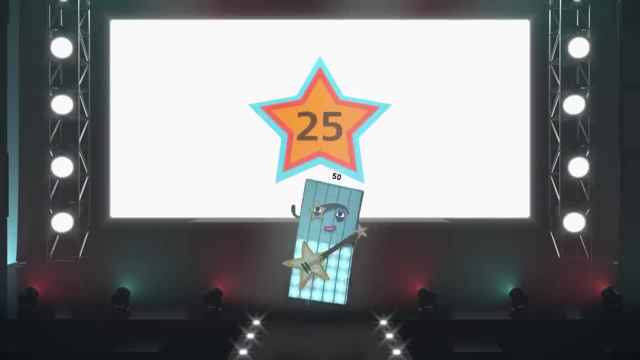 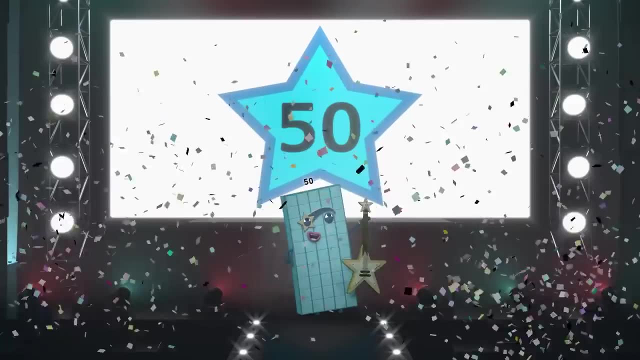 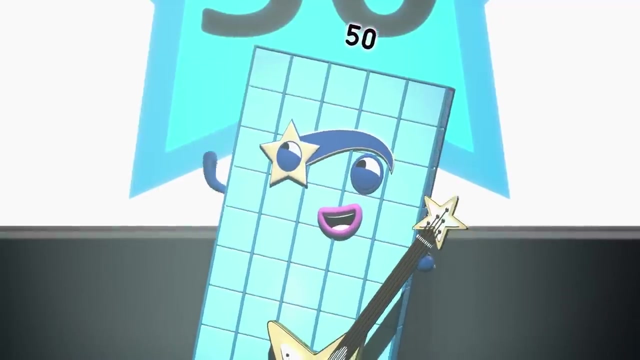 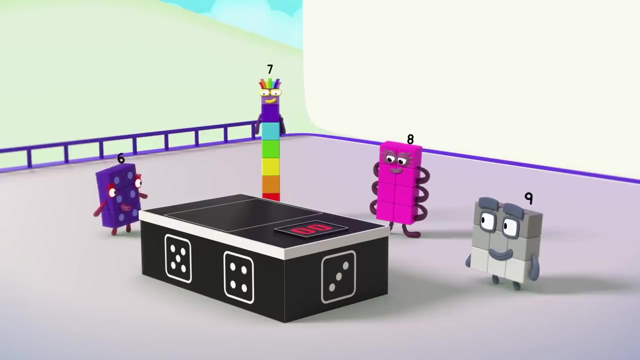 Who am I? 5,, 10,, 50,, 20,, 25,, 30,, 25,, 40,, 45.. I'm 50.. I'm 50.. Yeah, Thank you for coming to play my big new game. 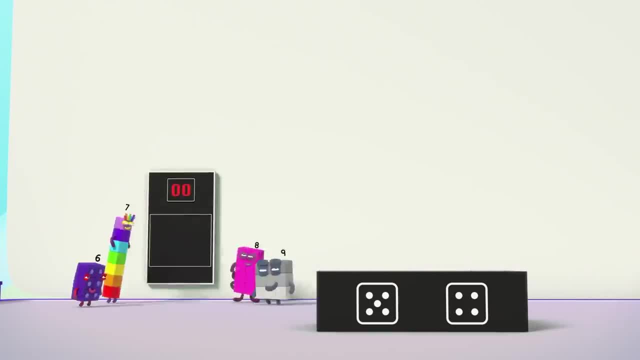 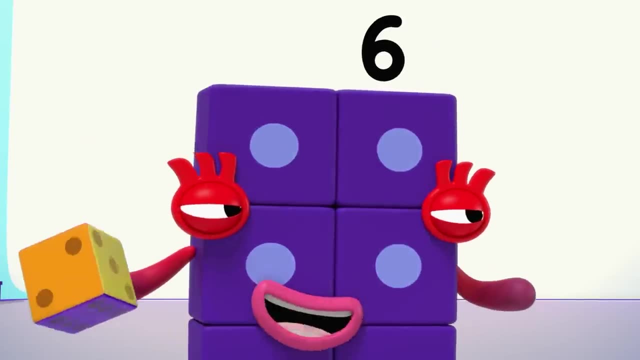 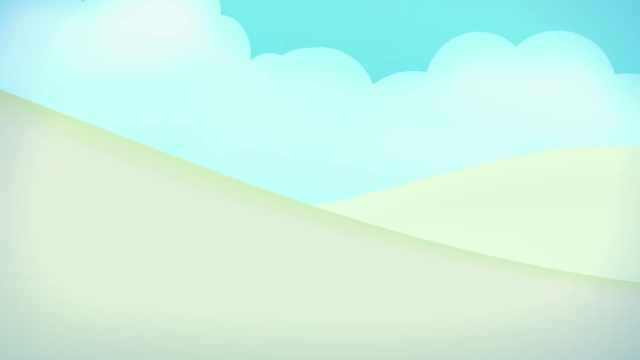 I'll roll the dice to start my friends. This game is called How Many Tens? Hmm, Six Six times 10 equals 60.. I am 60 here to play with 60 spots. hip, hip hooray. 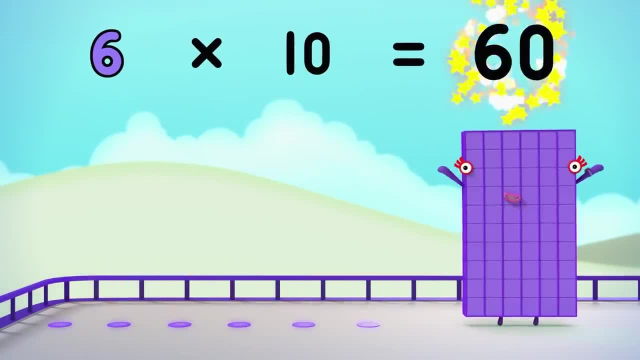 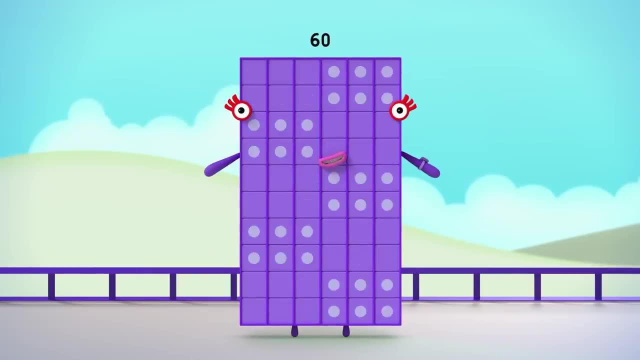 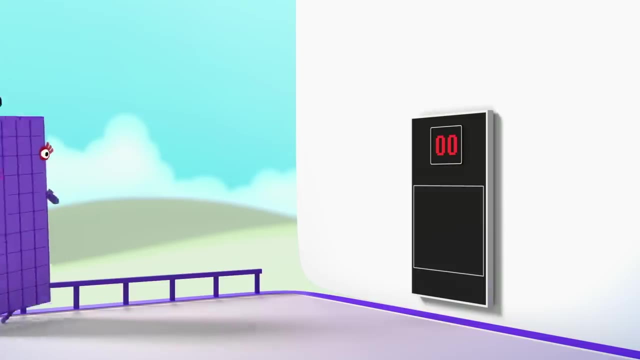 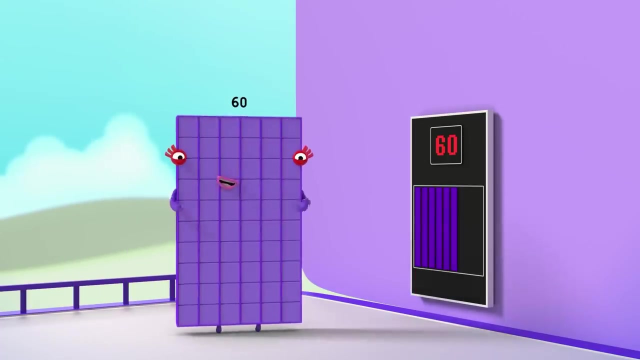 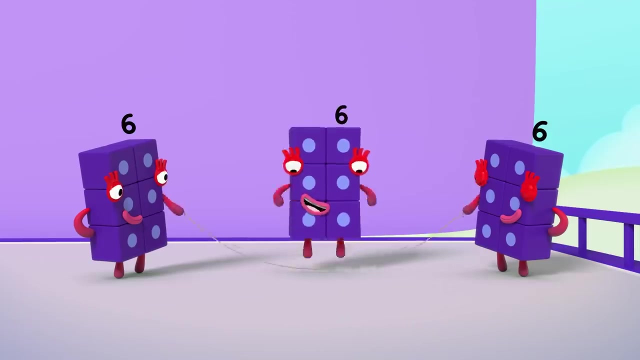 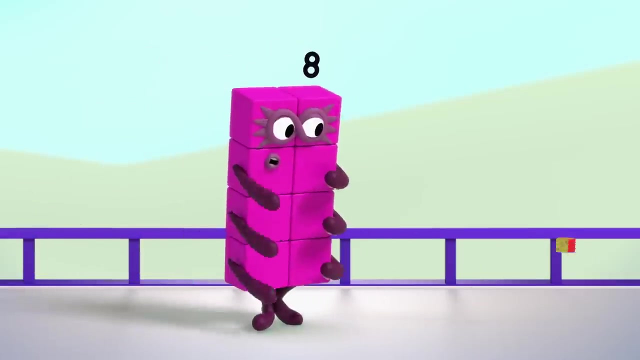 Wow, 60.. Six lots of ten is a new high score. I'm six, tens or Ten sixes. Game on. Yeah, Come on Nine, we can. Whoa, Oh, Uh-oh, Oh, no, The special game dice. 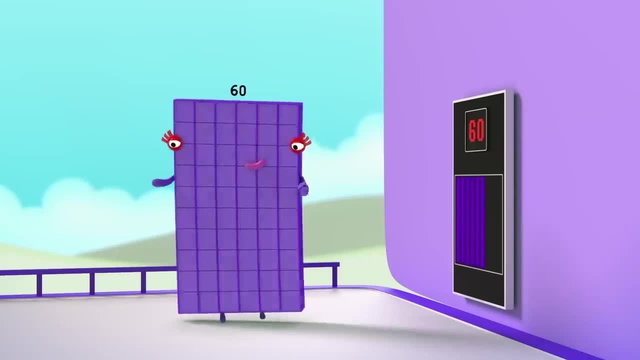 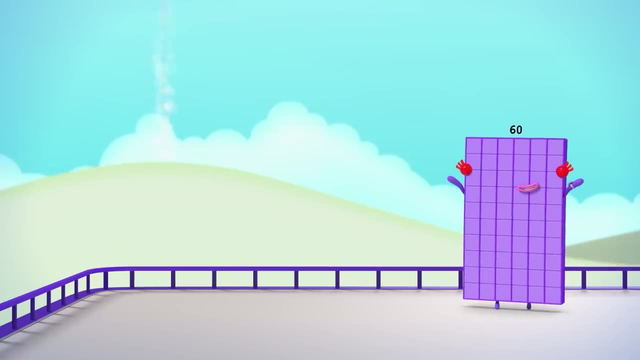 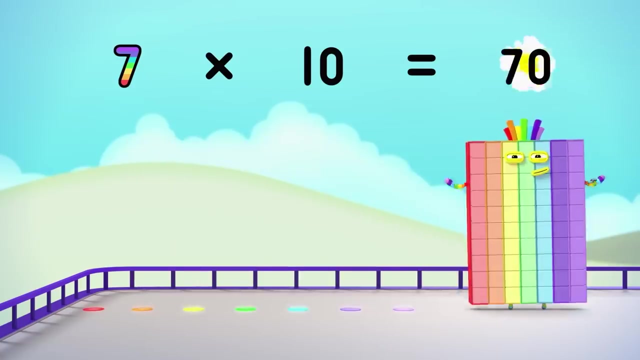 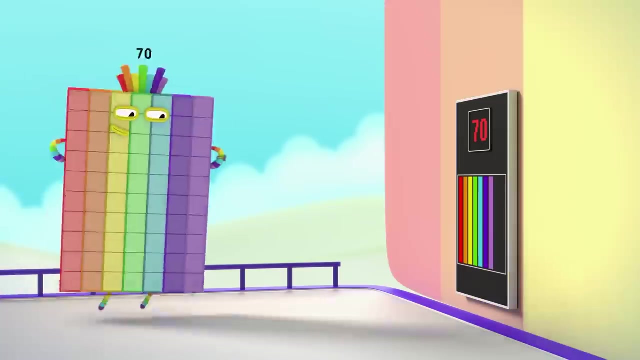 I'm sure you'll see that dice again. This calls for A normal dice. This calls for another ten. Seven times ten equals Seventy. I am 70.. You lucky numbers, As luck would have it, I'm seven tens. 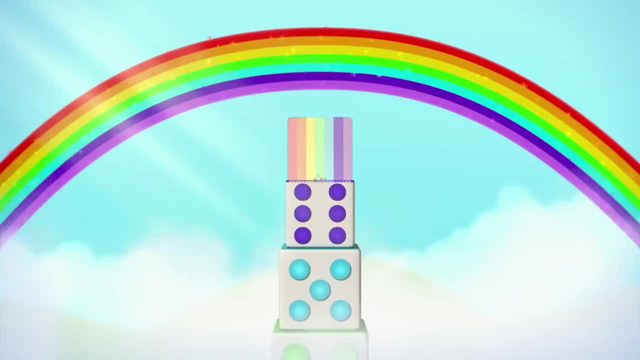 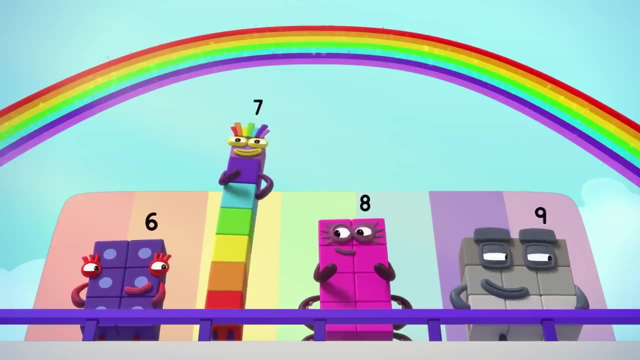 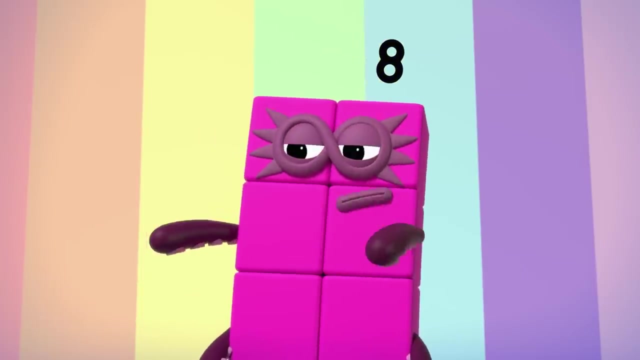 So I'm also Ten. sevens, The Rainbow Collection. Ooh, Whoa, Ooh. I see it. It's way over there, But how can we get it back again? Luck is in the air tonight. Here comes another ten. 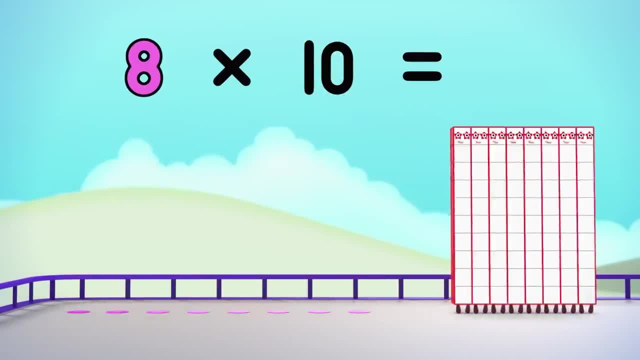 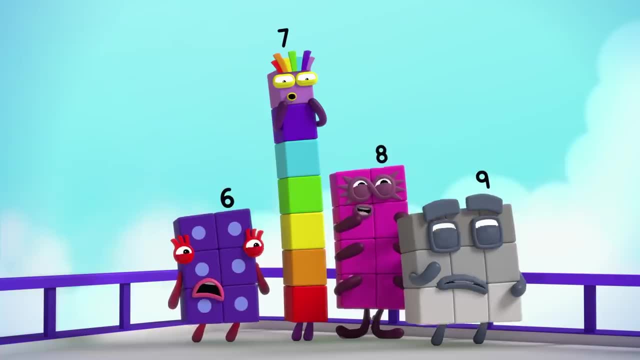 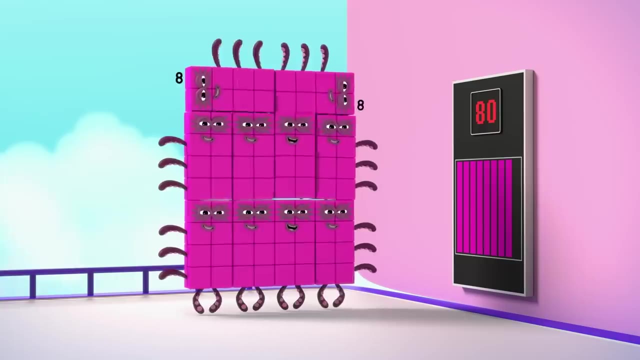 Eight times ten equals Eighty. I am 80!. Super Octoblock to the rescue. Whoa, Oh, Secretly, I'm eight tens. But this is a job for Ten, eights, Octoblocks assemble. 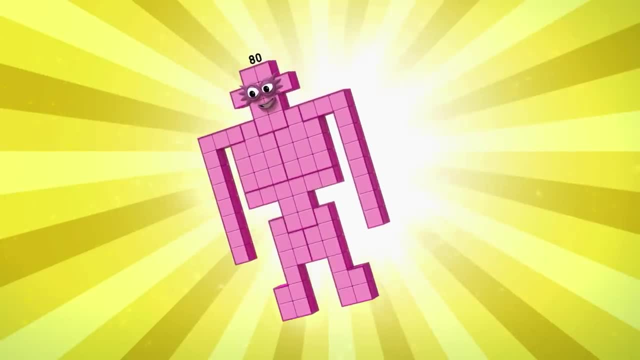 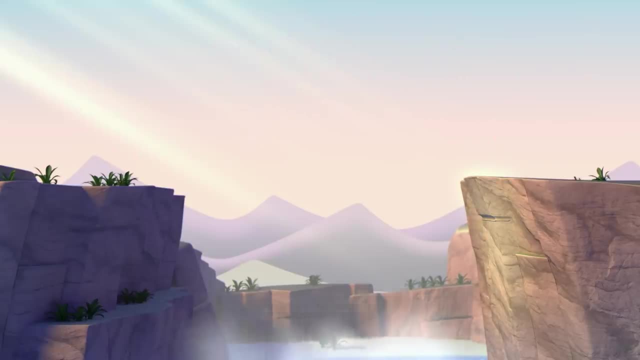 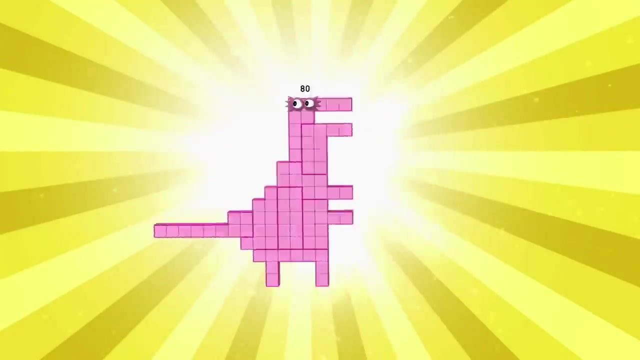 Roboctoblock forward. Whoa, Ha-ha, Ha-ha, Ha-ha, Ha-ha, Ha, Mmm. Ha-ha, Ha-ha, Hmm, Ha-ha, Ha-ha, Ha-ha. 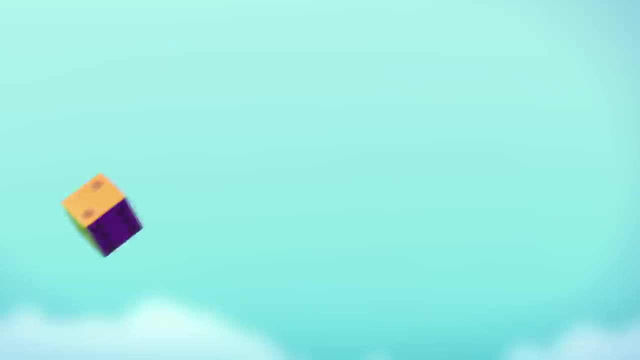 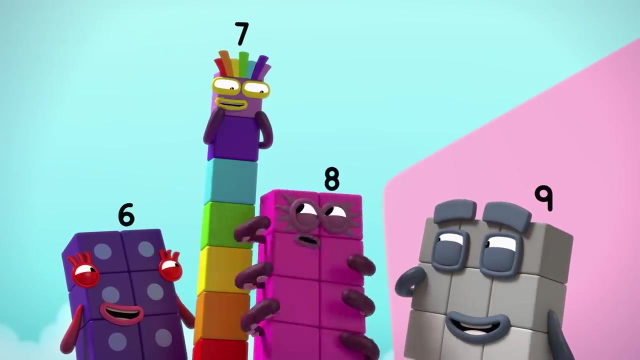 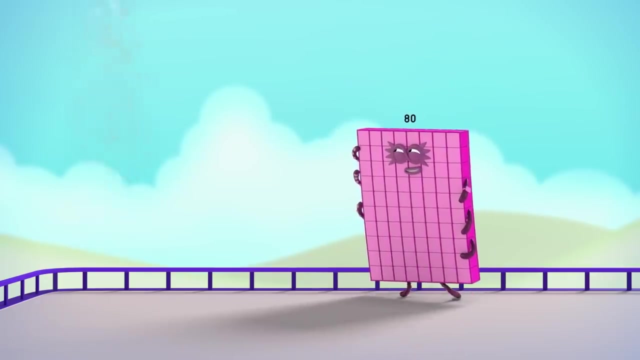 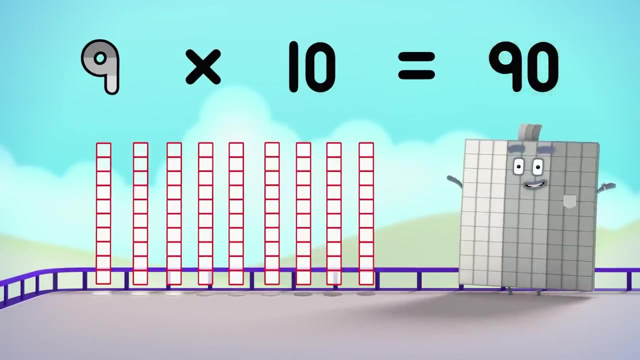 Dinoctoblocks, Rock smash, Huh, Whoa. Eighty's the biggest hero of all. Oh, There's always someone bigger. Look Up in the sky. Its Another ten. Nine times ten equals 90!. 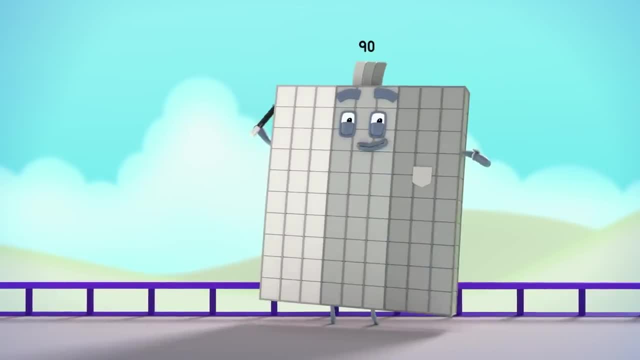 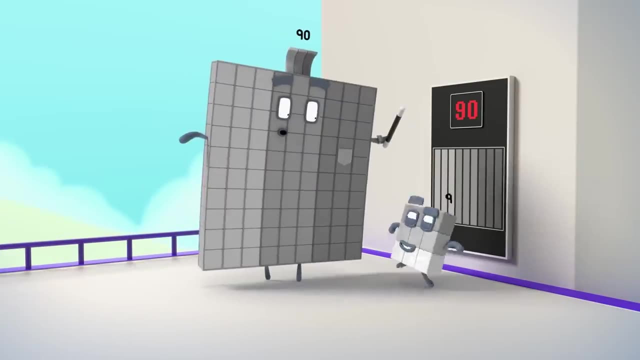 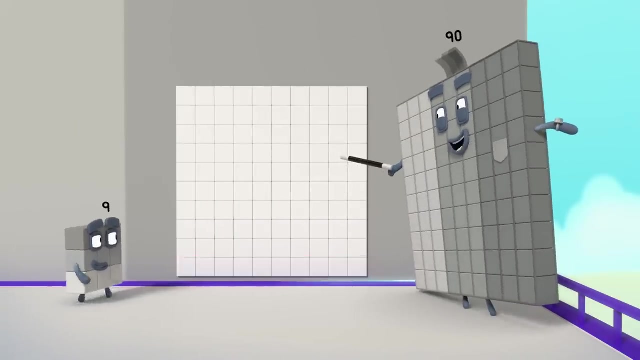 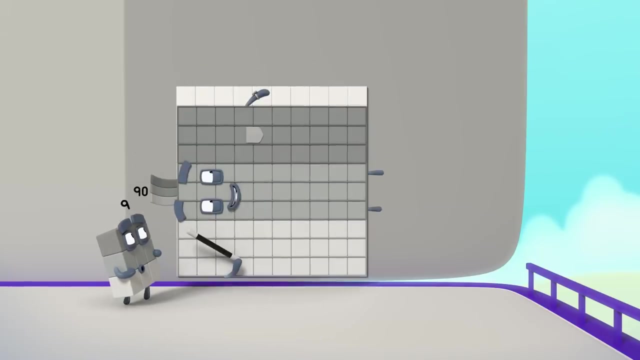 I am 90!. You won't believe your eyes. Are you a square or not? I can't tell. This grid is ten blocks by ten blocks, But I am one column short or one row. Either way, I'm not all square. 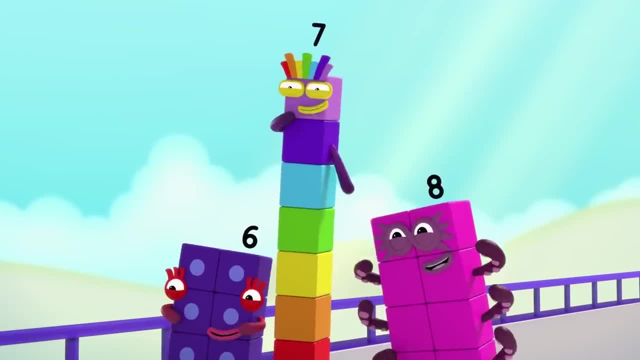 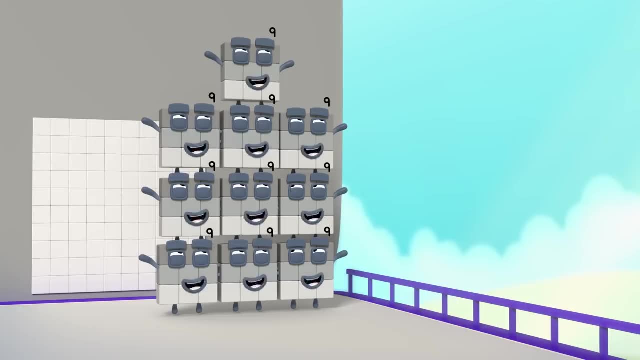 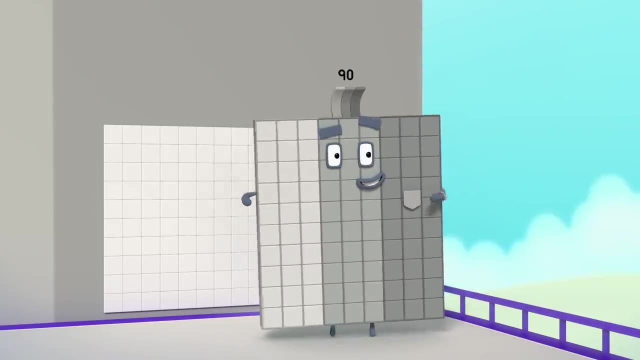 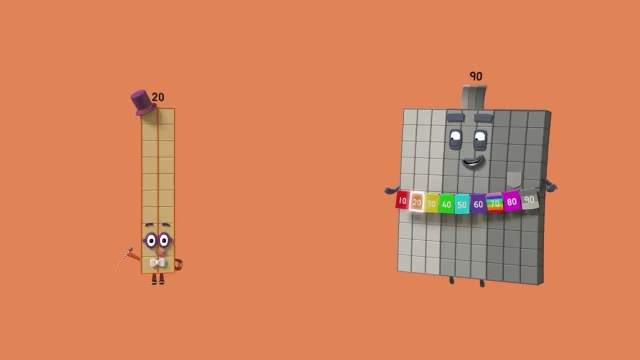 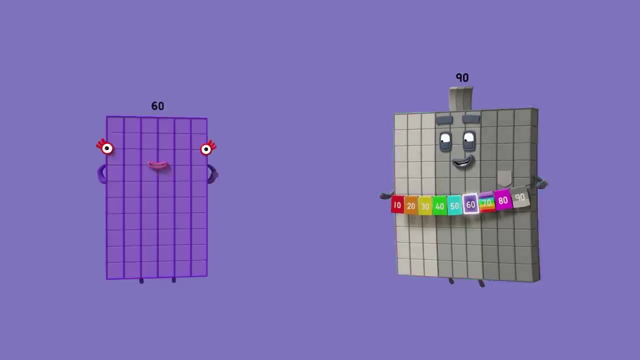 Ah, And now a vanishing trick. Ten lines, Ten lines. Now you see us, Achoo, Now you don't. And what have we got here? Ten, Twenty, Thirty, Forty, Fifty, Sixty, Seventy. 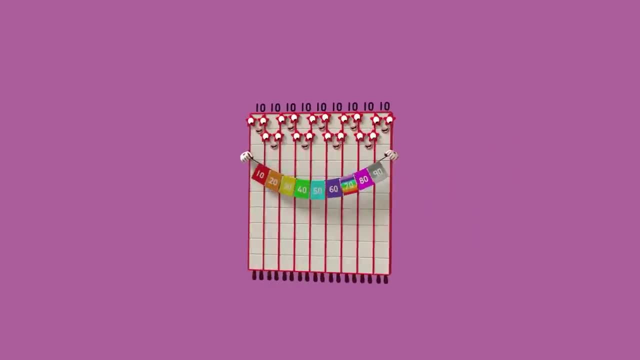 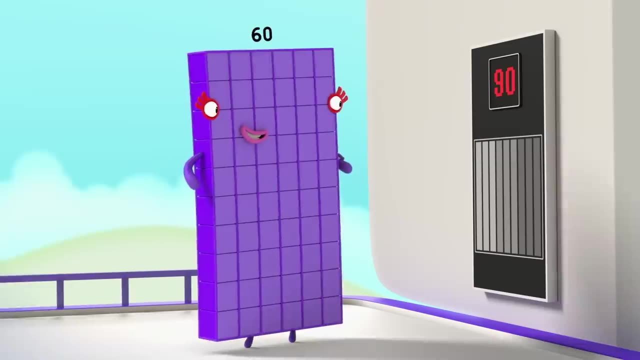 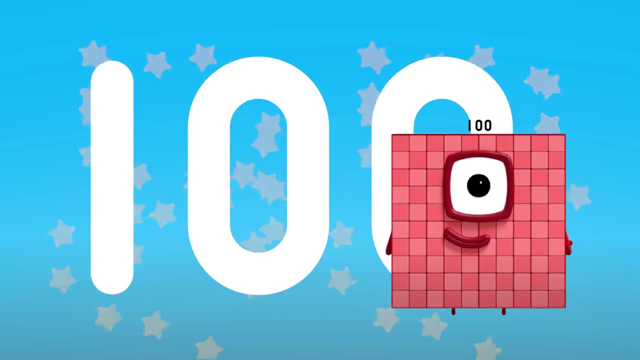 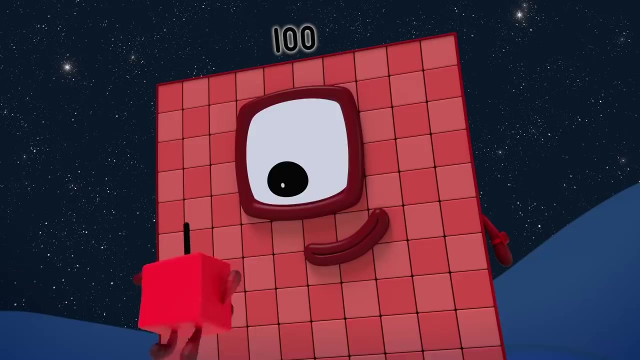 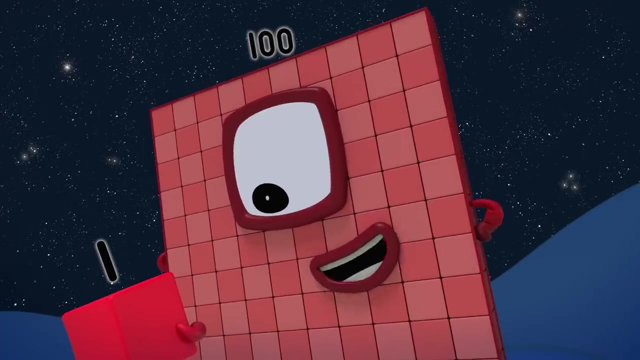 Eighty And Ninety. Ninety's got the highest score, but I wonder how long. four One hundred is here. One One hundred, Hello one, You're so big. Yes, little one, I'm a big one. 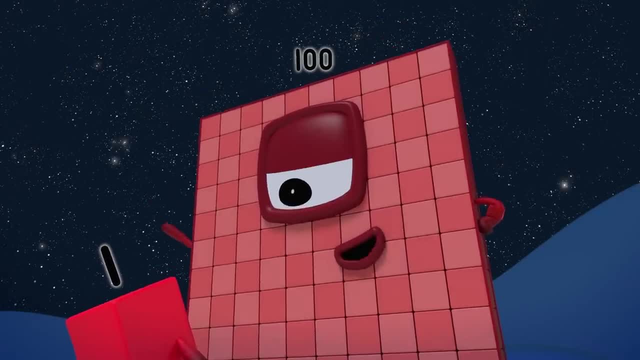 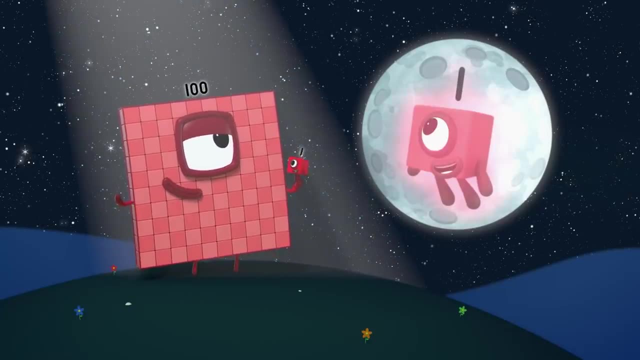 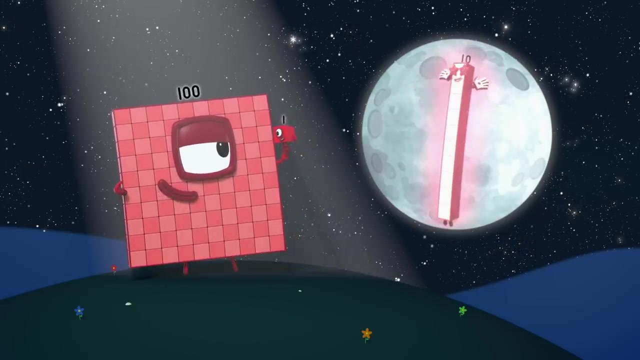 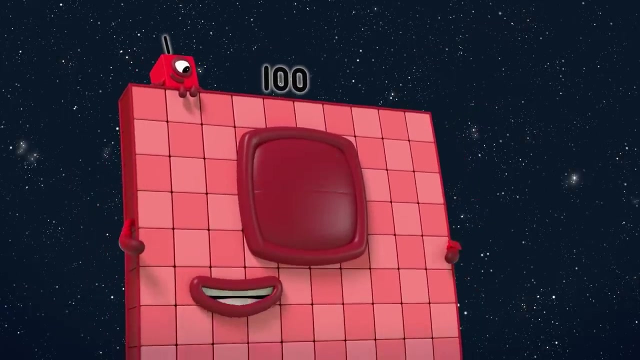 I'm a big number, But I wouldn't be here at all if it weren't for you. Ooh, Look how far we've come. Remember when there was only one? Then ten ones made one ten. We're the one and the zero. Now we've reached a new place. 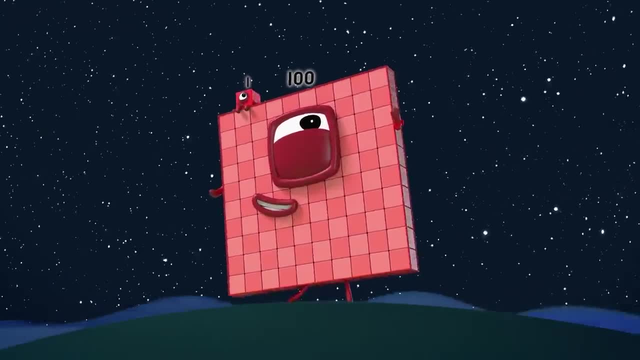 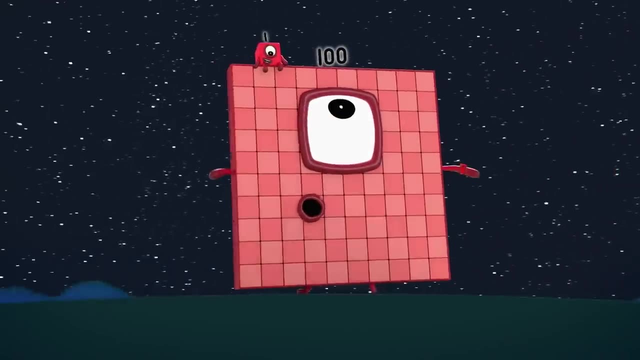 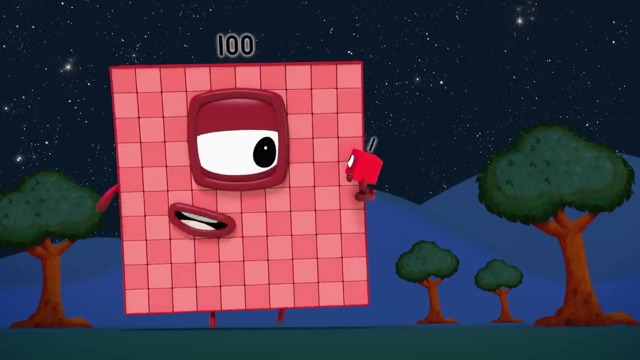 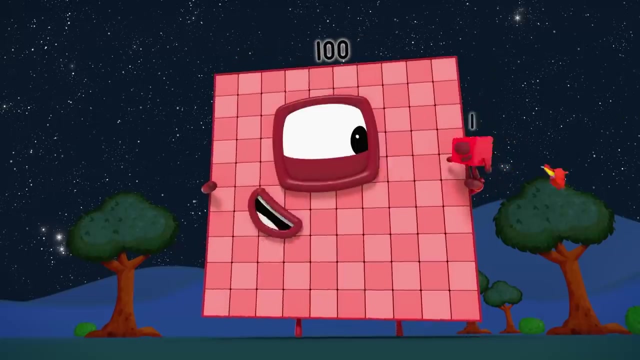 The place of possibilities And new friends And a new face And a brand new kind of hero. I'm big, So big. I'm really really, really big. I am gigantic Gigantic. Did I mention I was big, Mm-hmm, I'm taller than the tallest tree. 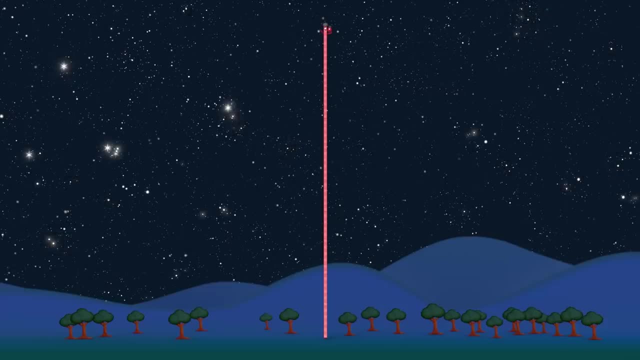 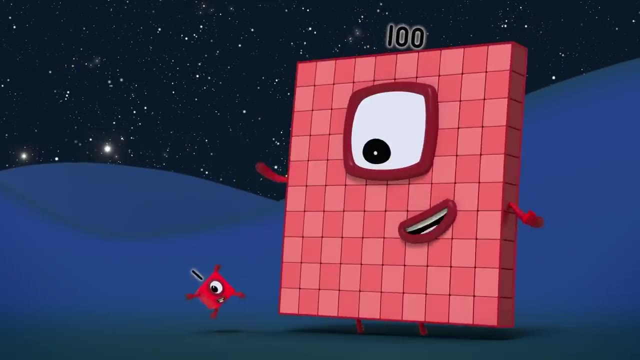 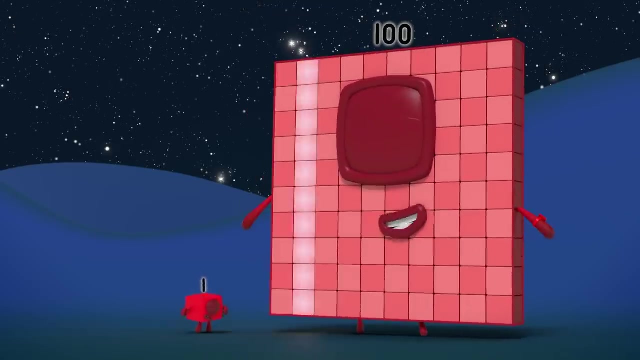 No one here's as tall as me, Because I'm big. I'm really very big. Look: One, two, three, four. I'm so big. you'll need a quicker way to count. If you count ten tens, one ten at a time, You'll reach the right amount. 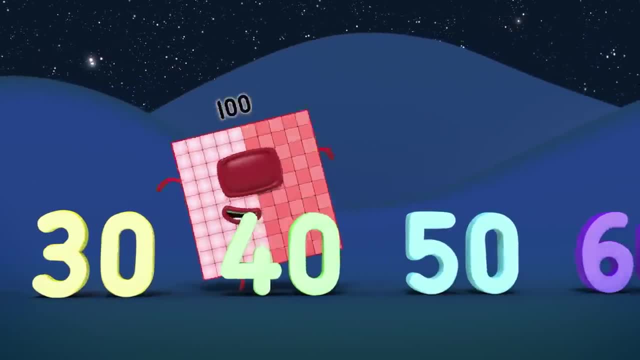 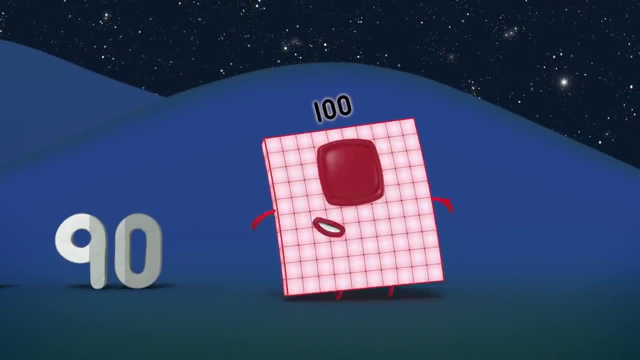 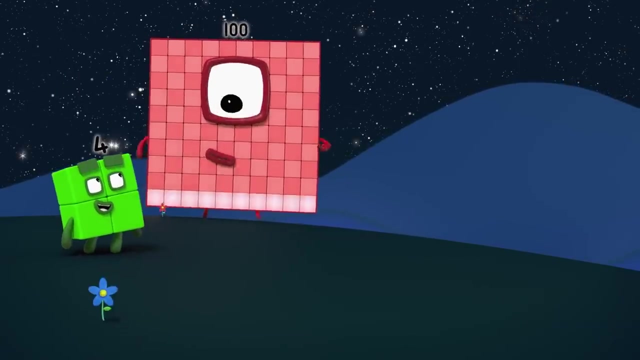 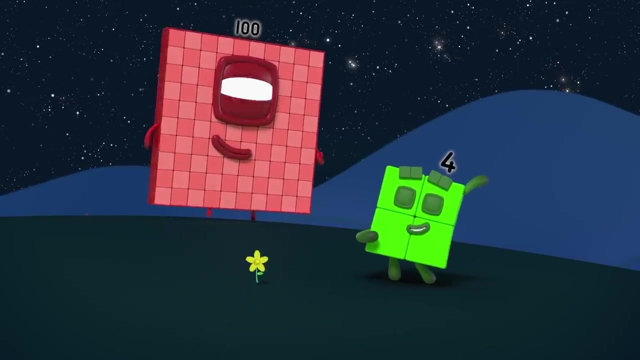 Ten, twenty, thirty, forty, fifty, Sixty, seventy, eighty, Ninety, one hundred. She's square. Oh, I'm ten by ten. That makes me square. She's impressive. Ooh, Now I've noticed that she's square One, four, nine, sixteen, twenty-five. 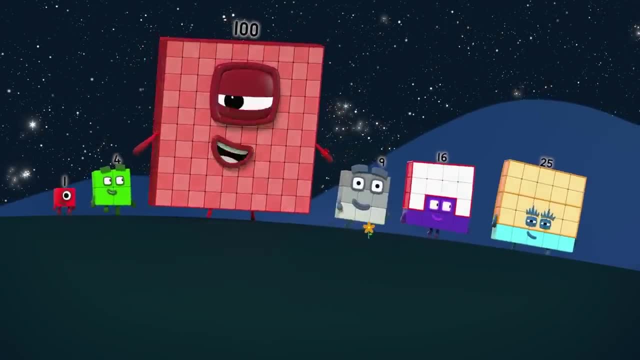 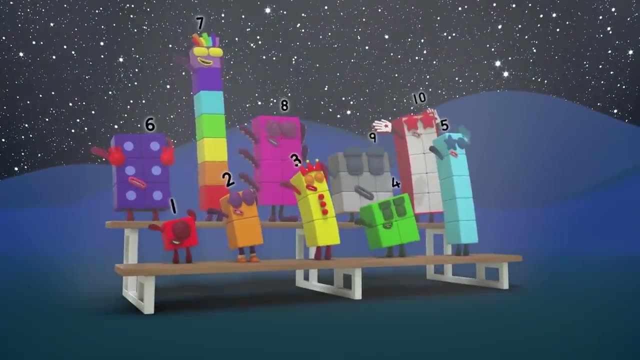 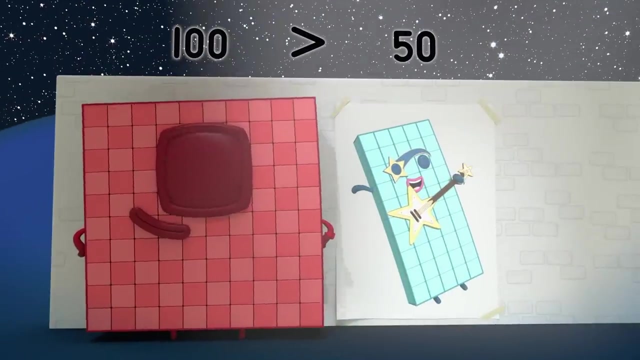 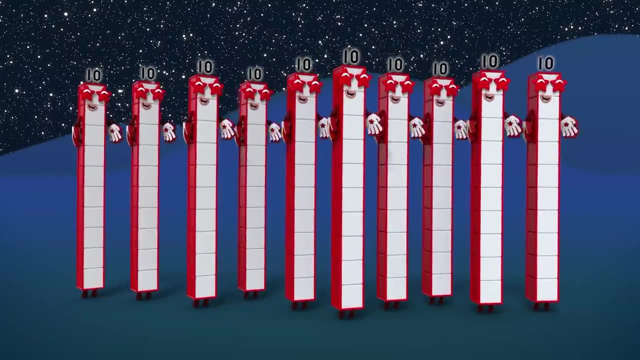 You'll know when all the squares arrive, Cos I'm square, I'm one big matter, I'm a massive square. She's great. You can't help being quite impressed. She's the greatest, She's greater than the rest, She's ten times ten, as you can see. 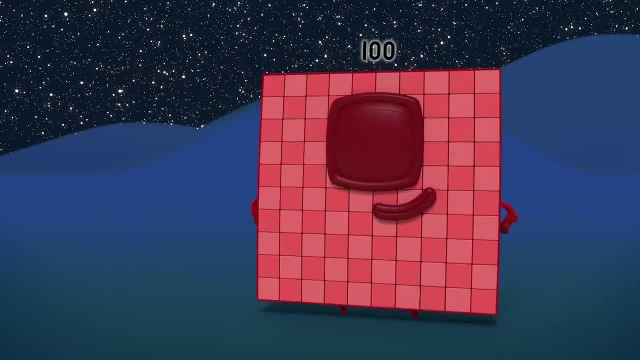 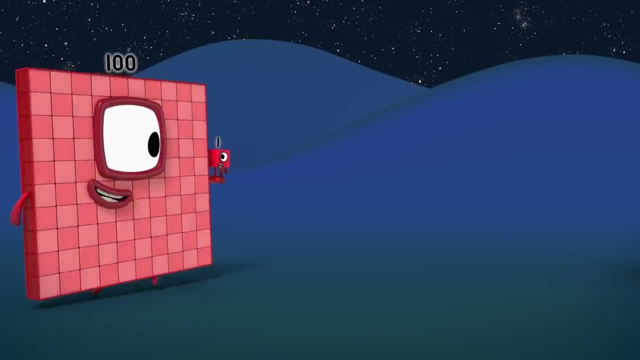 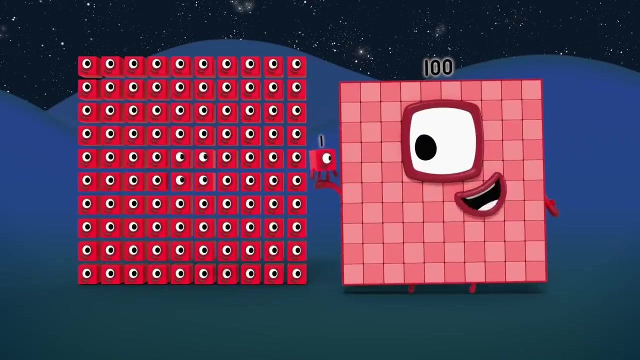 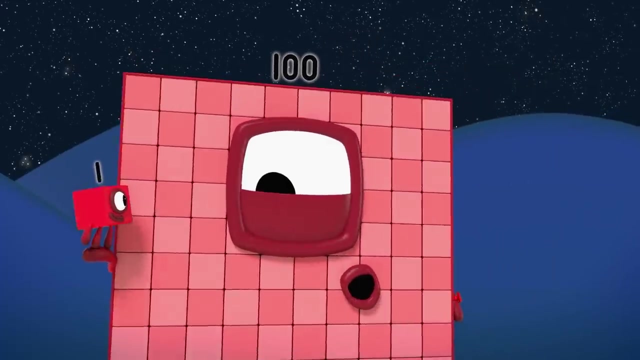 A hundred times the size of me. She's great. We all think she's the best, But I'm still one of you. I'm one with you. It takes a hundred ones to make one me. I won't make fun of you. I'm not done with you. 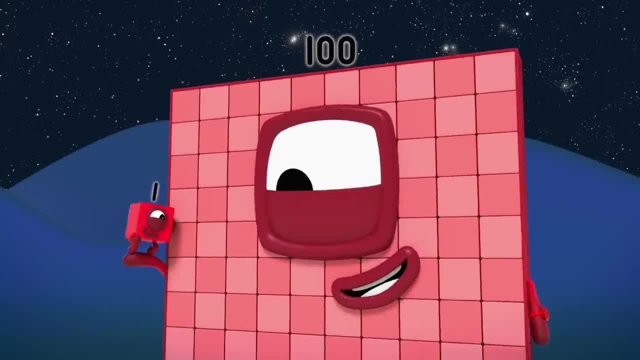 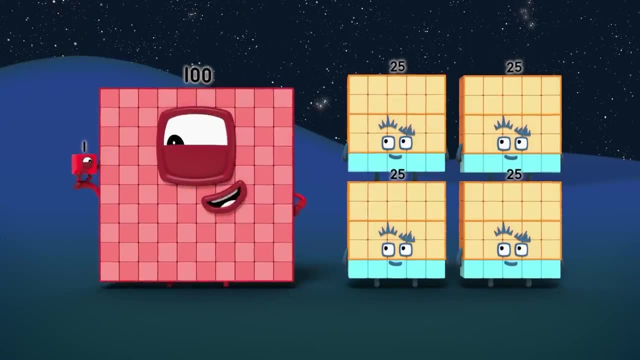 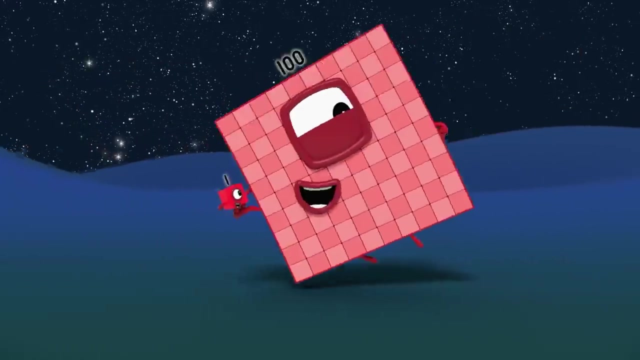 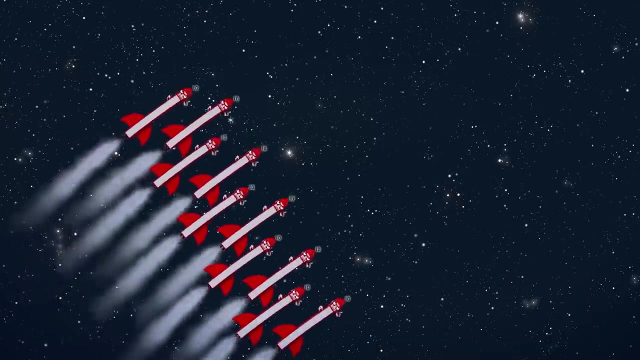 Inside I'm just like anyone you'll see, But I'm big. Well done, I'm really really Somewhat big. I'm tremendous, She's tremendous. I'm proud that I'm so big. You'll see ten tens as we fly by, Ten rockets shooting through the sky. 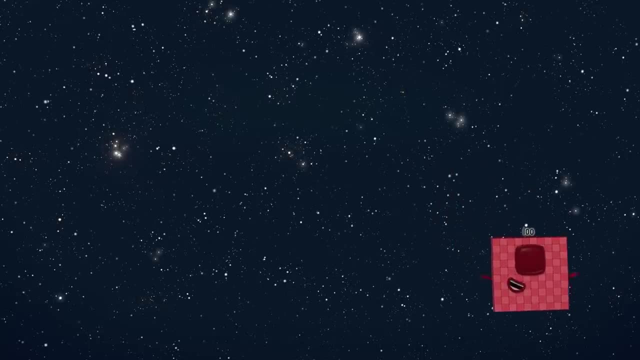 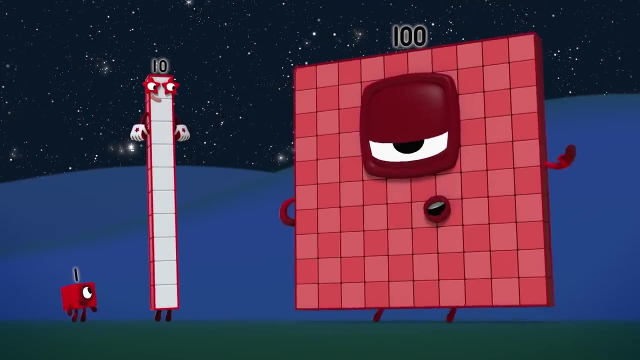 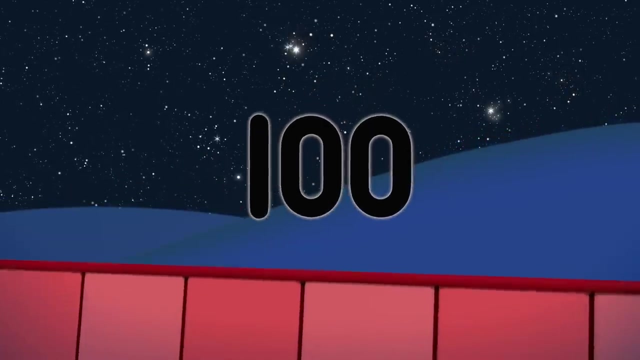 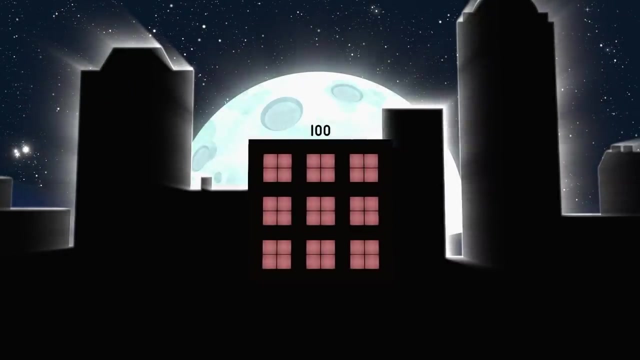 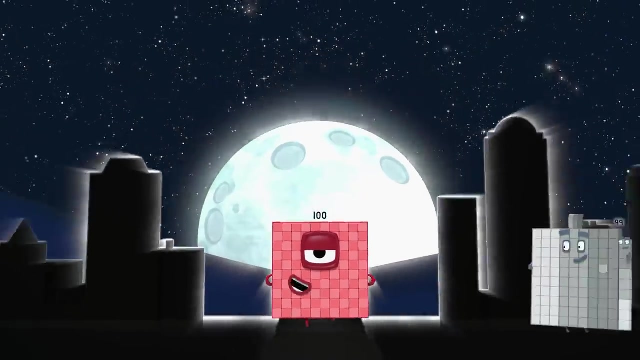 That's big, Unquestionably big. I'm bigger Cos I've got three figures, My zeroes and zeros. My zeroes might give you a clue. Is this the start of something new? I'm big. I'm really really, really big. I'm a landmark. You can't miss me. I'm that big. 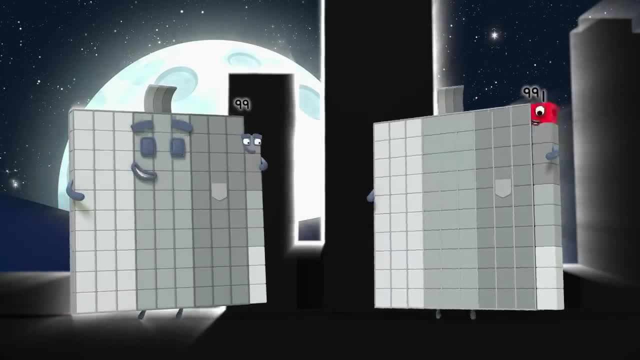 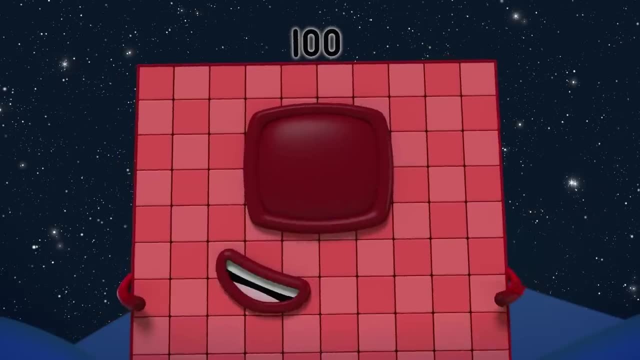 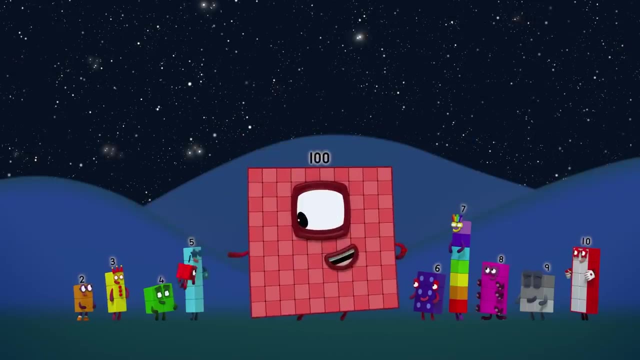 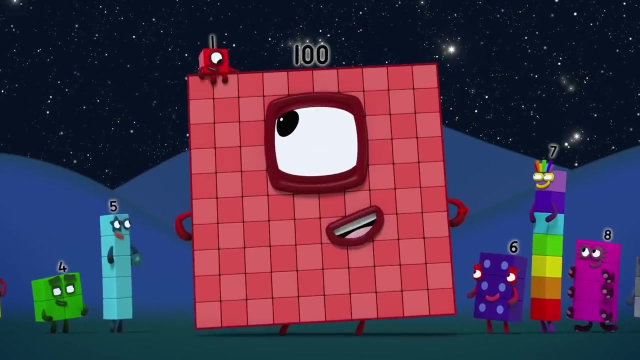 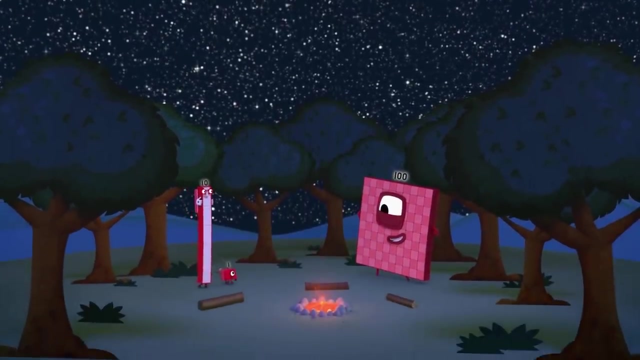 And life's a hundred times more fun When you're ninety-nine plus one. I'm big, She's tremendous. I'm big, She's tremendous, I'm really, really, really, very big. Ah, Hello one, Hello ten, Hello one hundred. 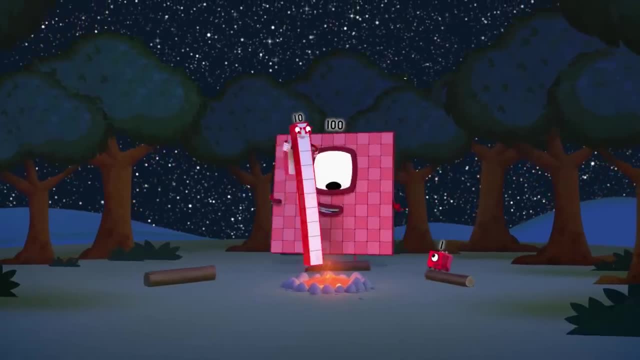 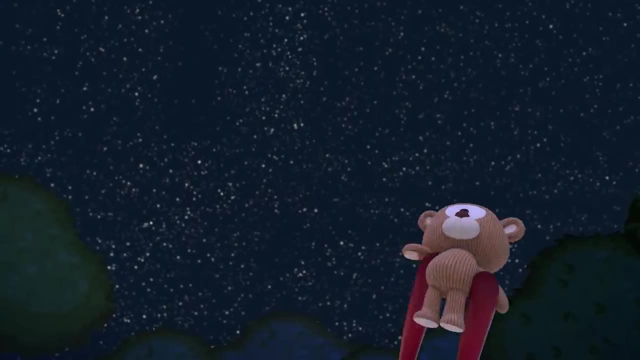 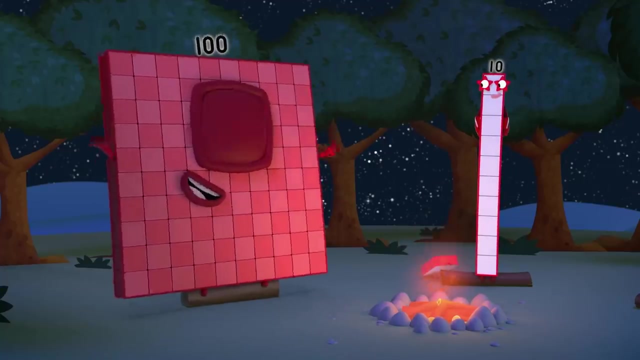 Sit, sit. One's place, ten's place, hundred's place. Look, Teddy, so many stars. There must be a hundred of them. Oh, there are many more than that, More than one hundred, But you're the biggest number I know. 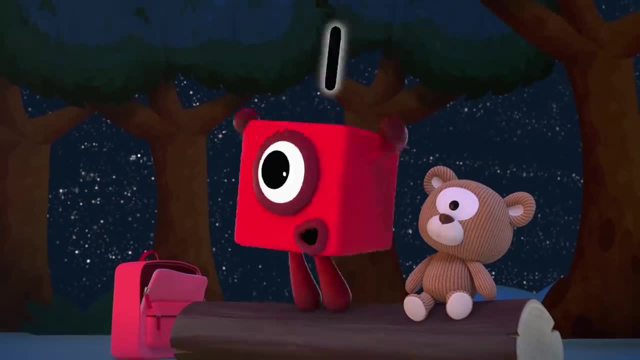 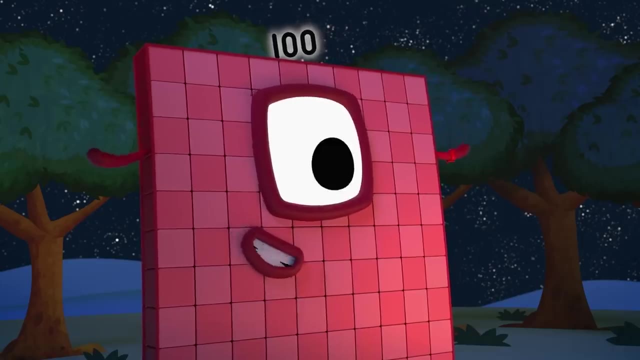 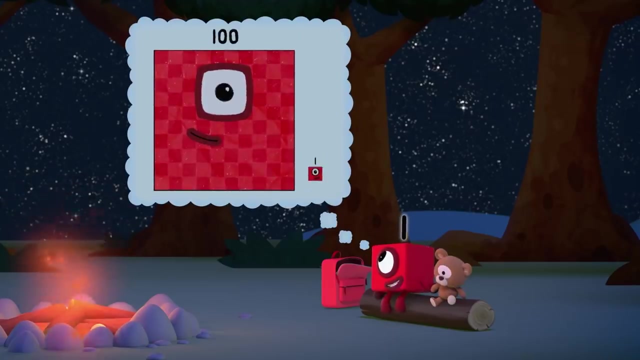 You can always make a bigger number by adding one. And how would that look? Think, think big. This is a good night for big thoughts. Oh, I love thinking about numbers. Look one hundred. if I join up with you, we'll be. 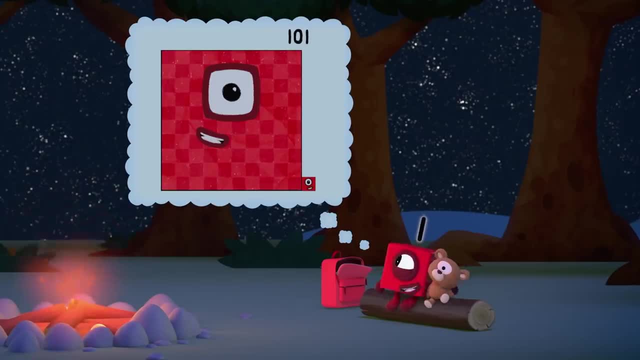 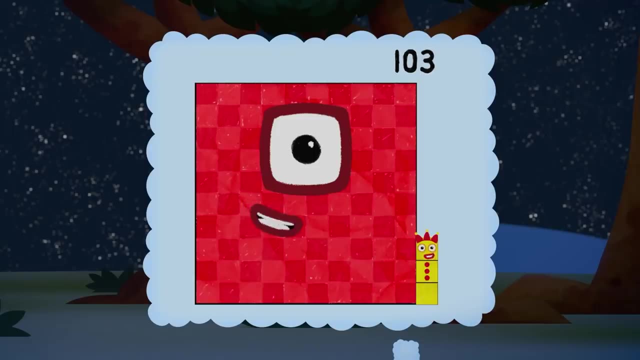 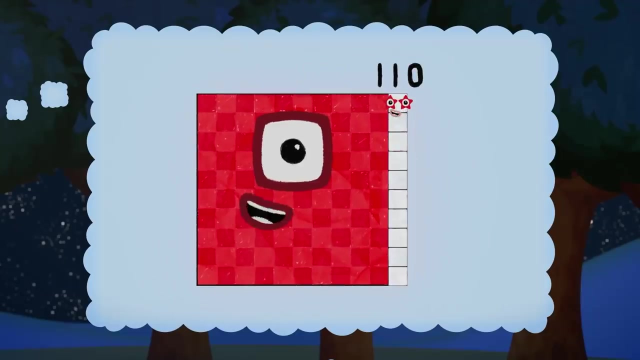 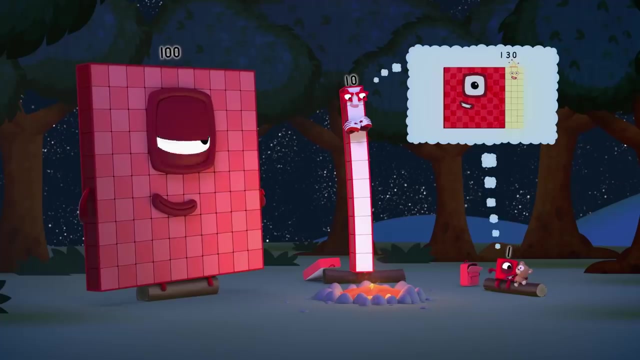 One hundred and one, And we can keep adding one, One hundred and two, One hundred and three, Or we can add tens, One hundred and ten, one hundred and twenty one hundred and thirty. And if we can add ones and tens, we can add hundreds. 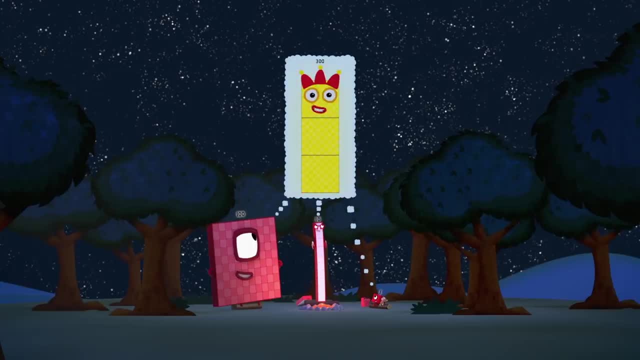 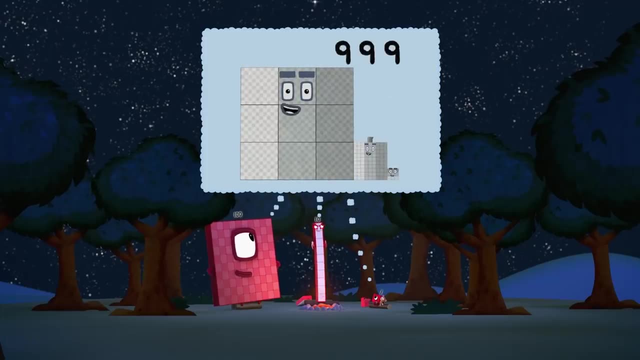 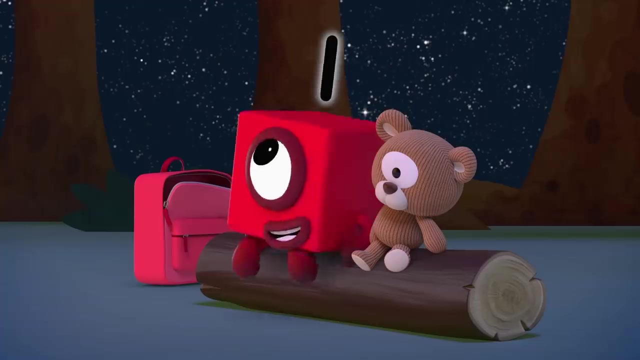 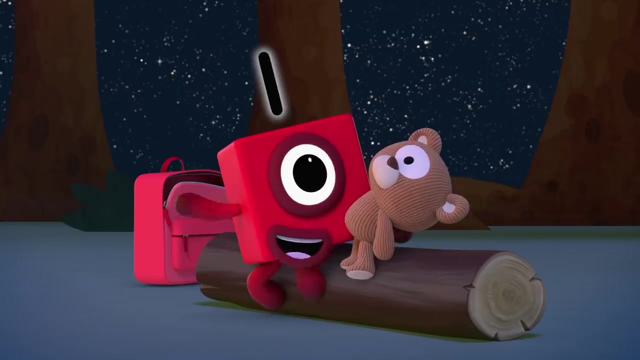 One hundred two hundred three hundred, We could make Nine hundred and ninety-nine. Wow, That's the biggest number I can think of, But there must be bigger numbers because we can always add more blocks. So what's bigger than nine hundred and ninety-nine? 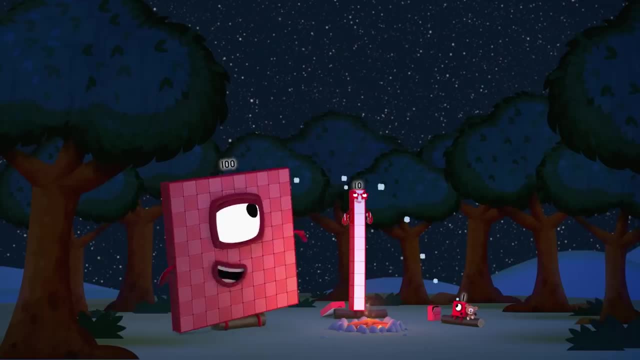 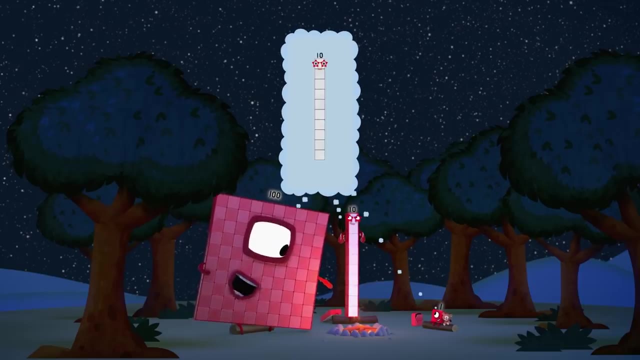 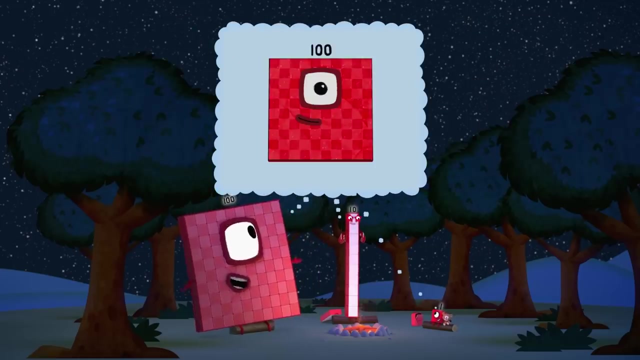 Think about it this way: Let's start with you. One One block, Now ten of you, Ten ones. What's that? Ten? Now let's have ten tens, What's that? One hundred, Now Ten hundreds, What's that? 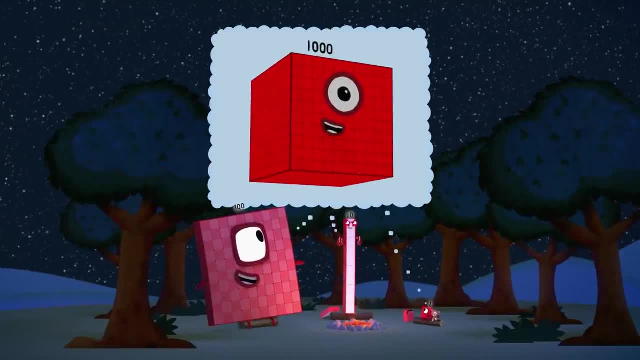 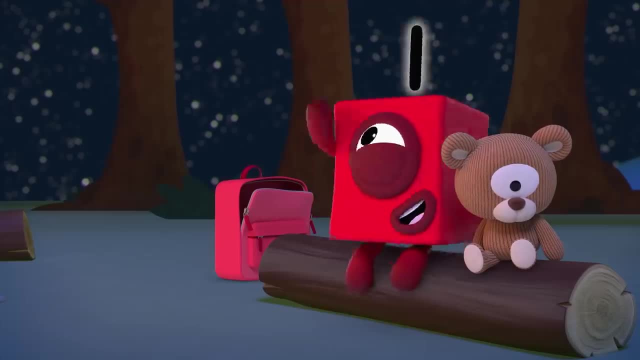 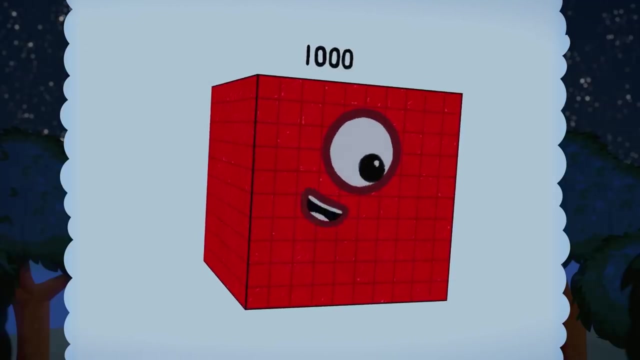 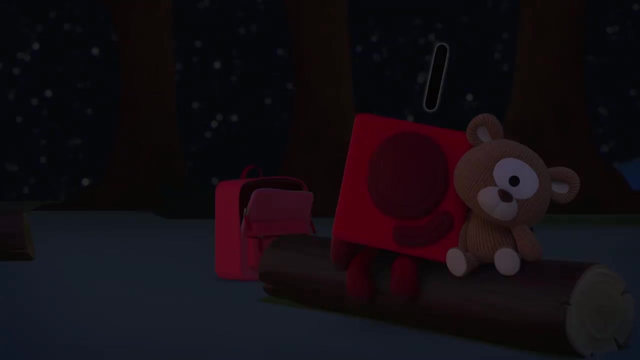 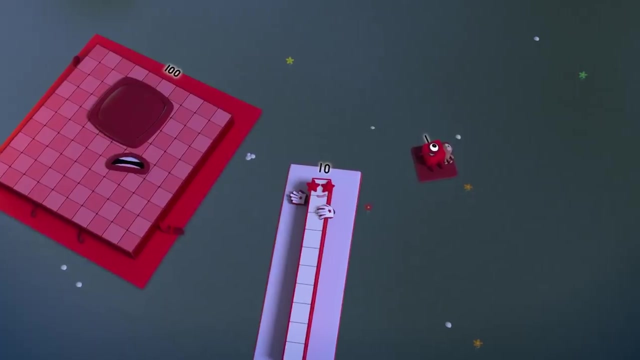 One thousand. You look like a giant, me. I'm a thousand ones. Wow, I can't wait to meet you. Ha ha, Ha, ha ha. Good night little one, Good night one thousand. There are so many big thoughts buzzing in my head. 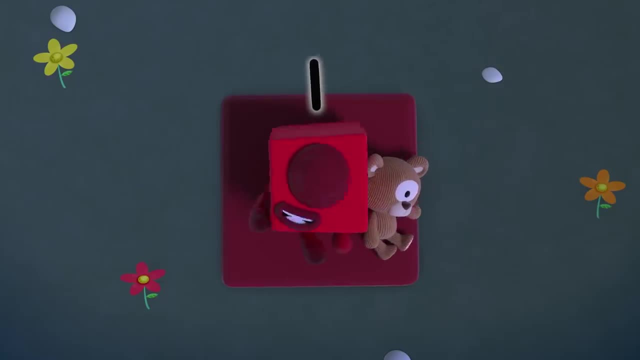 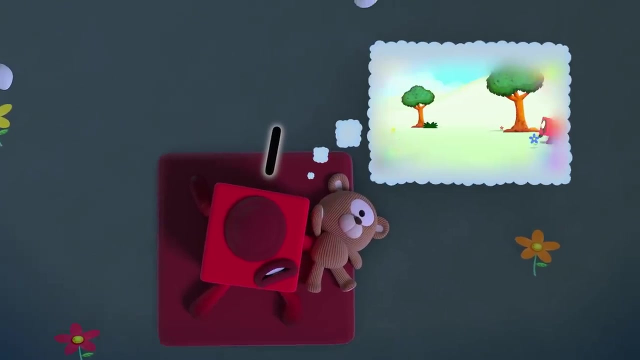 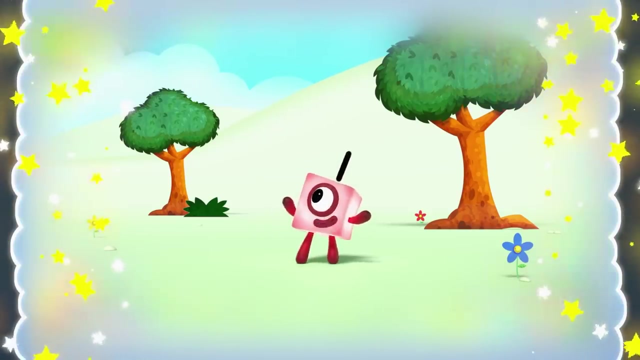 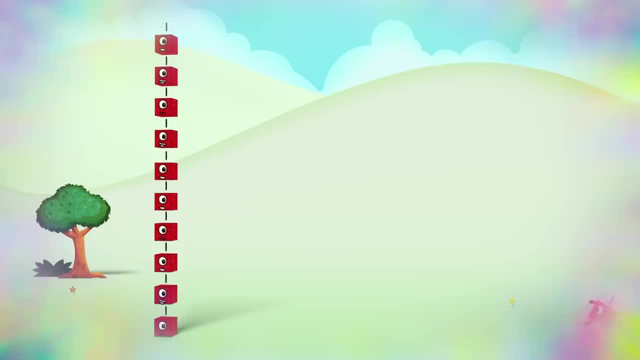 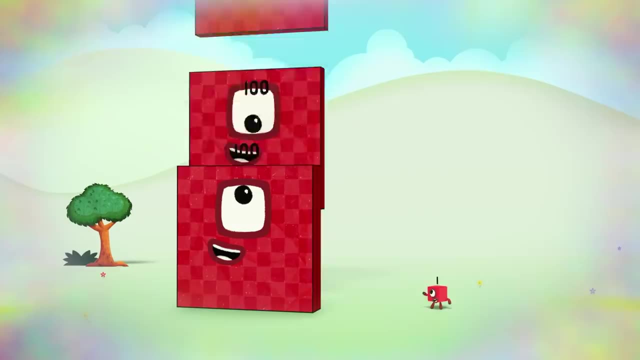 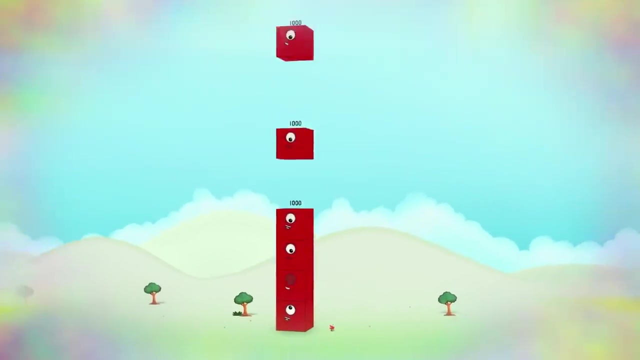 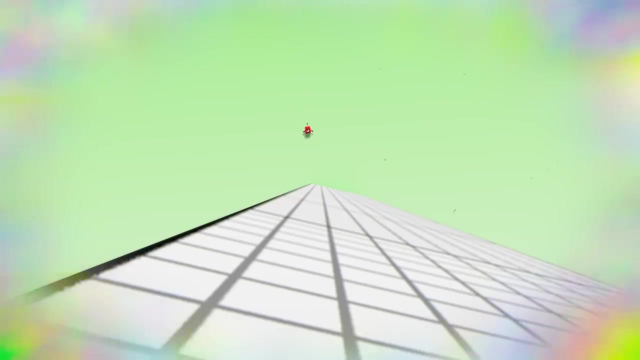 It's a big dream, A big dream, Hello dream. Ten ones are ten, Ten, tens are one hundred, Ten hundreds are one thousand. Ten, lots of one thousand are ten thousand. Ten, lots of ten thousand are one hundred, 100,000!. 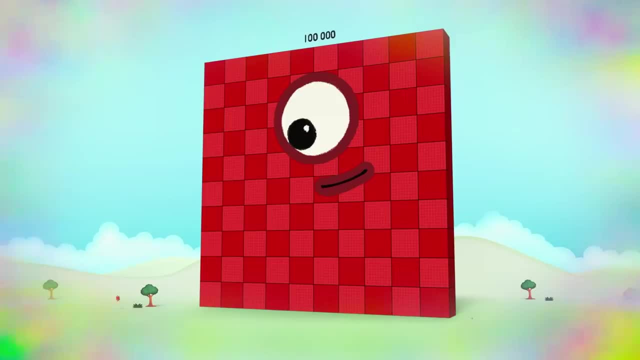 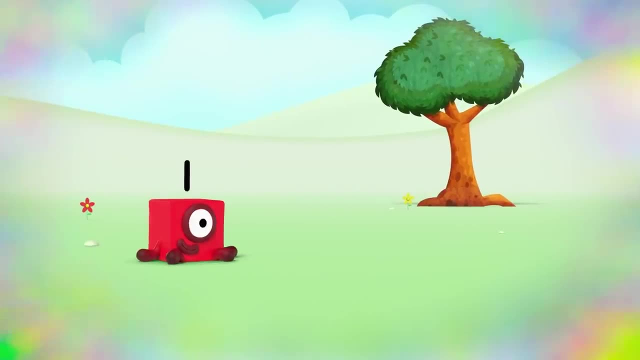 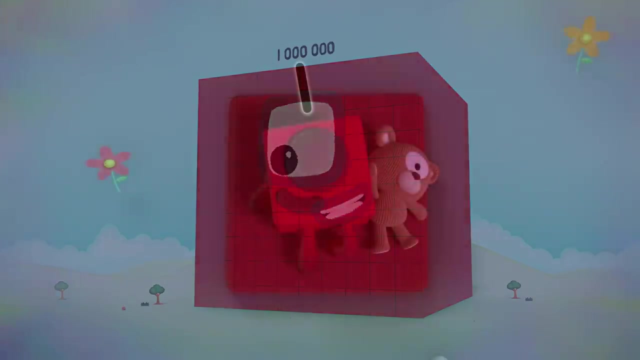 And 10 lots of 100,000 are One million. Hello, Hello, little one. Wow, I never knew there was a number so big And you can always make a number that's bigger, Bigger, Bigger, Bigger. 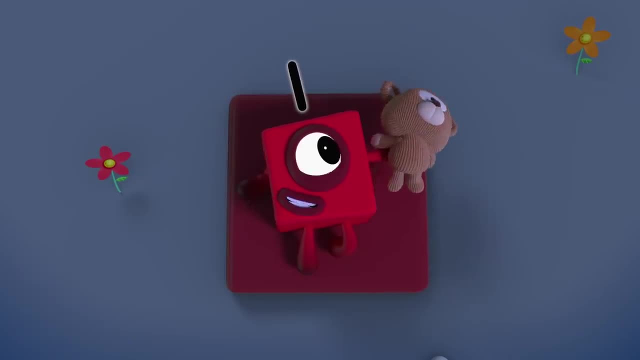 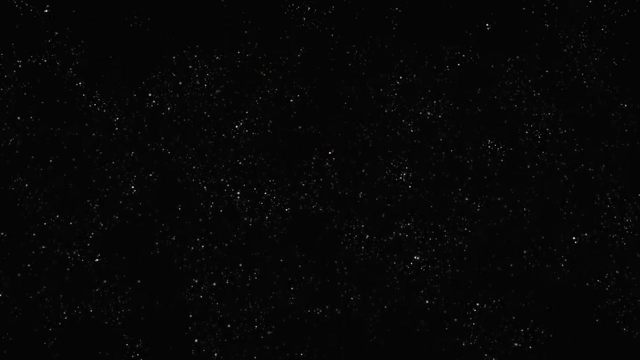 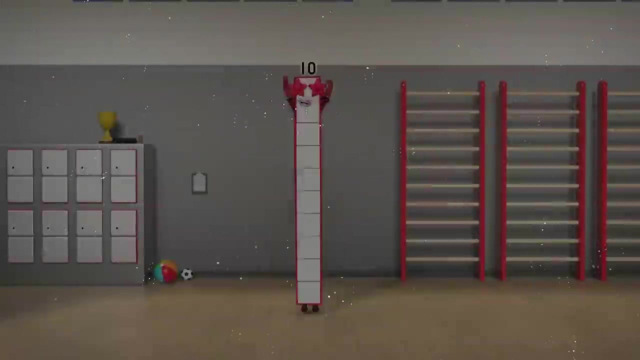 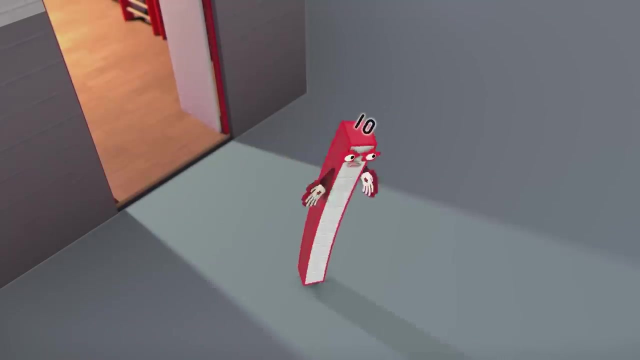 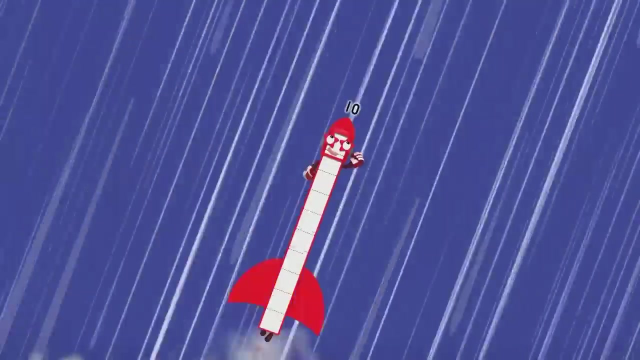 One teddy, One moon, One million stars And more. I can think of bigger and bigger numbers, Because numbers go on forever and ever. Ten, Ten, Ten, ten. ten Heroes with zeroes. this is the Ten Times Table. 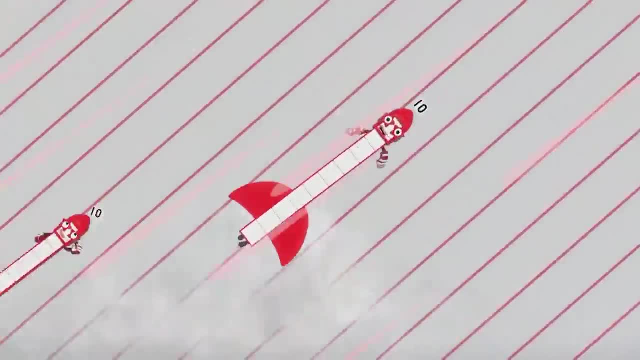 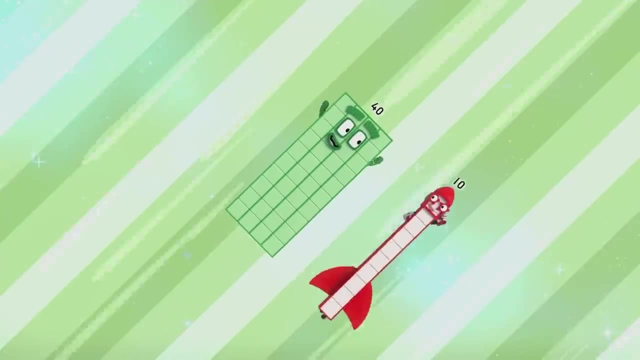 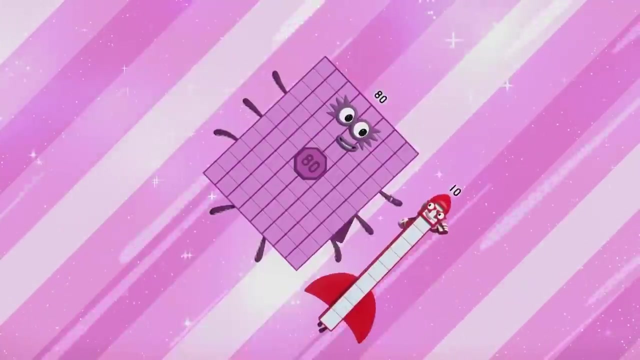 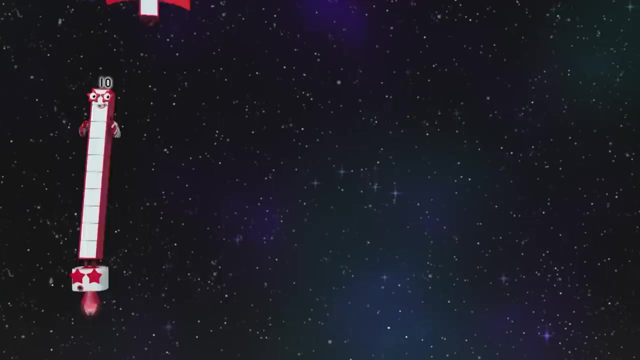 Rocket rescuers. come as soon as you are able. Ten, 20!, 30!, 40!, 50!, 60!, 70!, 80!, 90!, 100! Heroes with zeroes. One ten is ten. Two tens are 20.. 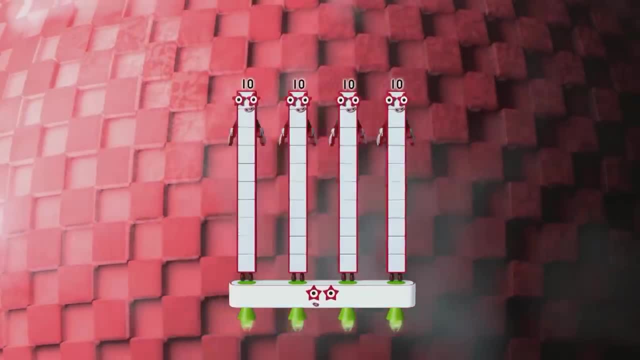 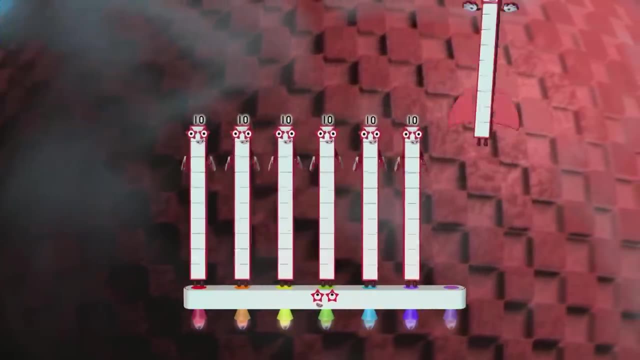 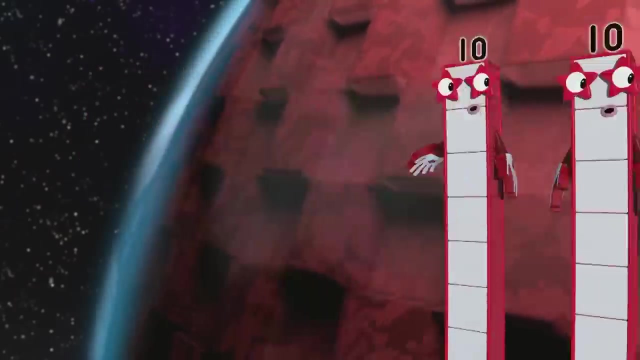 Three tens are 30.. Four tens are 40.. Heroes with zeroes. Heroes with zeroes. Five tens are 50.. Six tens are 60.. Seven tens are 70.. Eight tens are 80.. Heroes with zeroes. Heroes with zeroes. 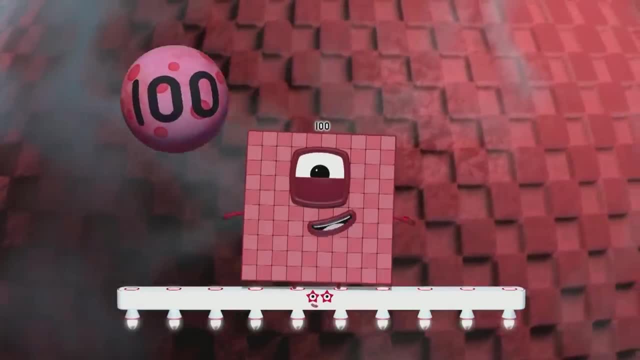 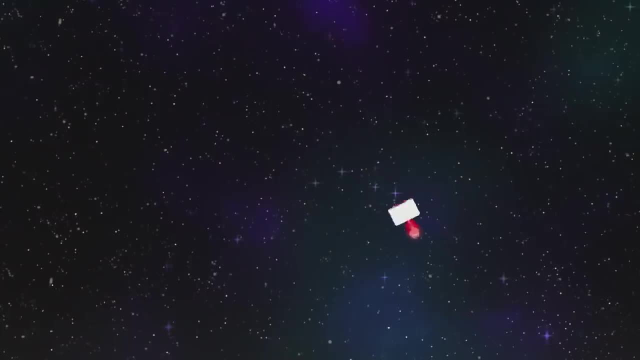 Nine tens are 90.. And ten tens are 100.. Heroes with zeroes. Heroes with zeroes. Heroes with zeroes. Ten is the original. She'll get us underway. Rocket to the rescue. Hooray Twengie has a double boost. 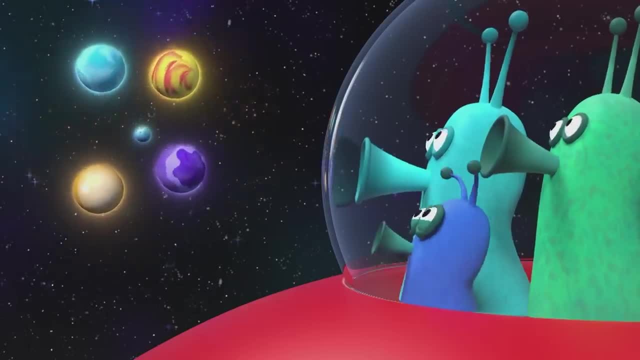 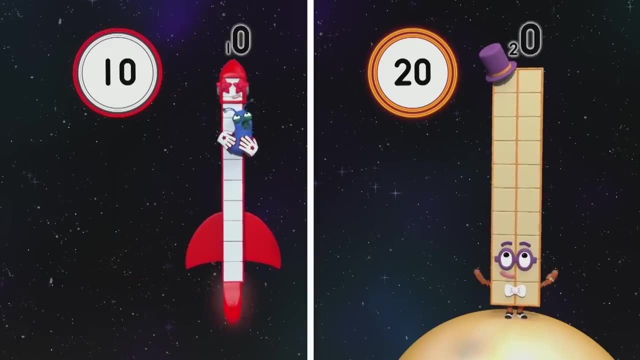 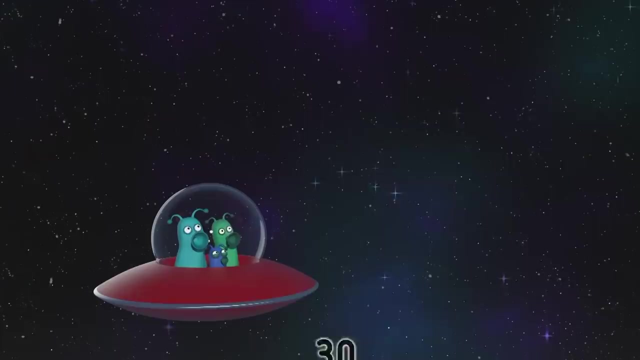 He can dance all day Interterrestrial tango. They know what their zeroes are: One ten, two tens And nothing more. Heroes with zeroes, 30 juggles, asteroids. You ain't seen nothing yet. The greatest show in space. 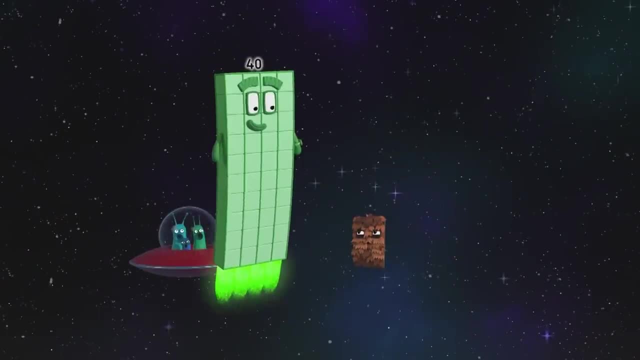 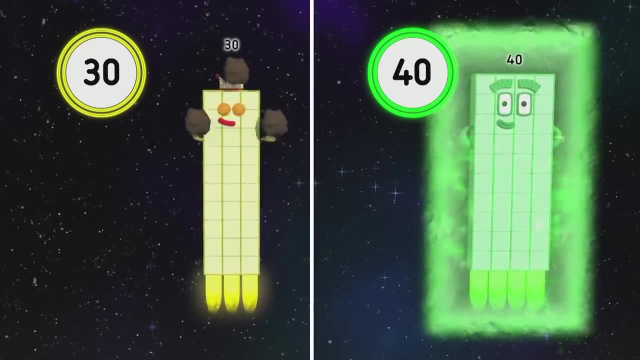 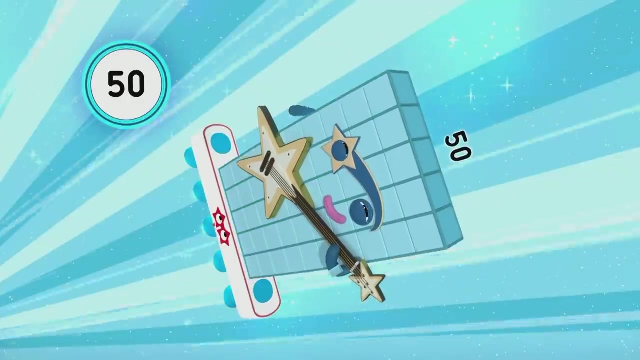 40 is a rectangle with an oblong pit, Intergalactic oblongs Three. They know what their zeroes for Three, tens, four tens And nothing more. Heroes with zeroes. 50 is a super star Who works the satellites. 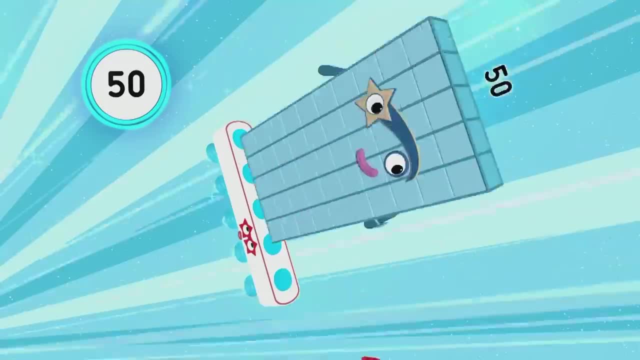 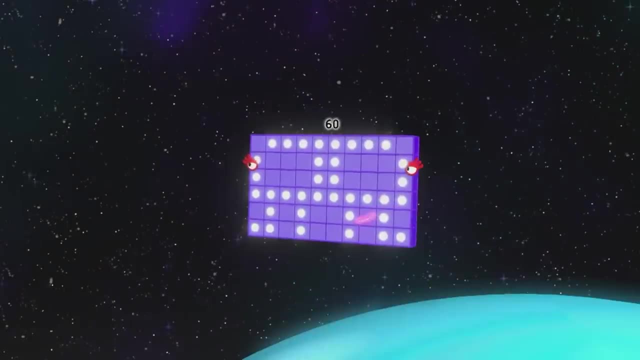 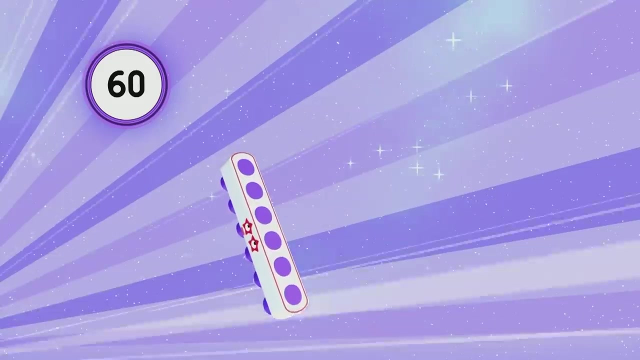 Interstellar overdrive. Yay 60 is a super gamer. She can light the lights. Galactic game over. Yay Five tens, six tens. Heroes with zeroes. 70 has luck times. ten Launching from the dock. 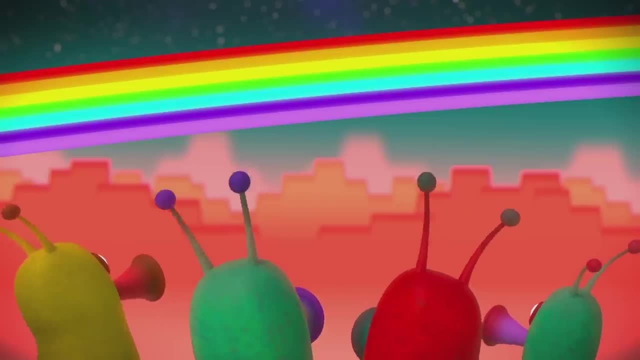 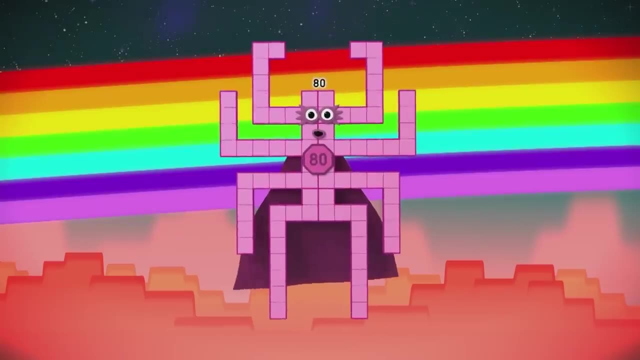 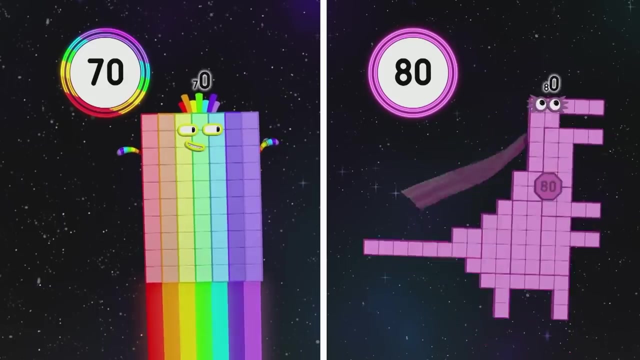 Space rainbow. Oh 80 needs no luck at all, He's super octoblocks. Night octoblock, Roboctoblocks, Night octoblock. Wow, They know what? their zeroes for Seven, tens, eight, tens And nothing more. 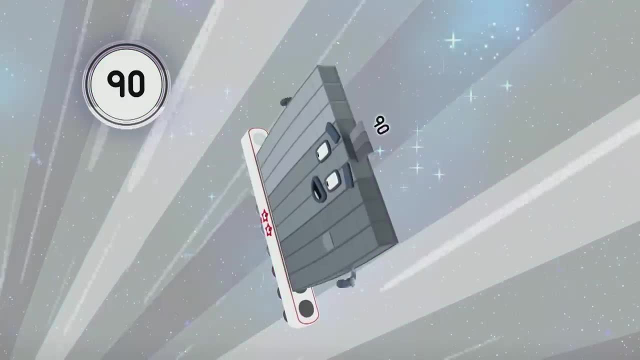 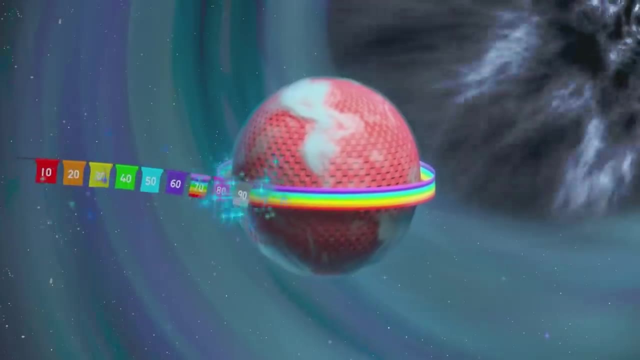 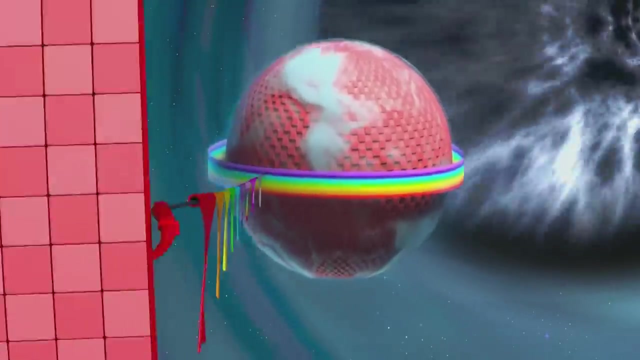 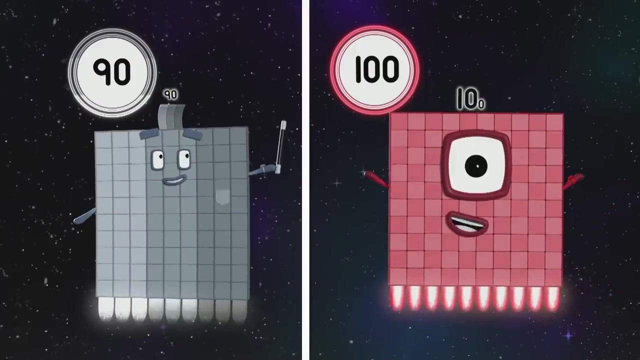 Heroes with zeroes. 90 knows a trick or two. He will heed the call Abracadabra. Oh, And now let's meet 100.. The greatest of them all, Hooray Hero, with two zeroes. Nine tens, ten tens. 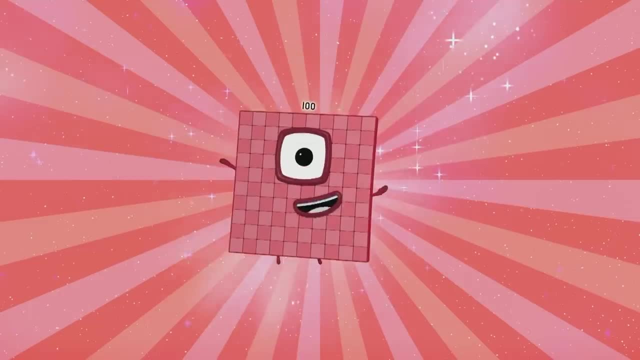 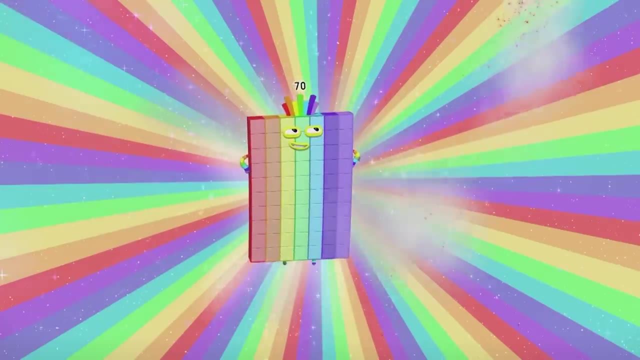 Heroes with zeroes: 100!, Hooray 90!, Hooray 80!, Hooray 70!, Hooray 60!, Hooray 50!, Hooray 40!, 30!. 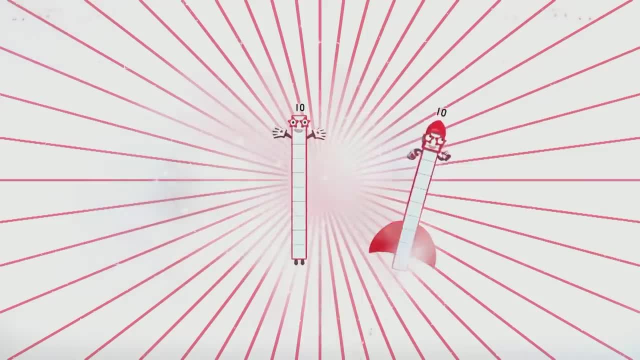 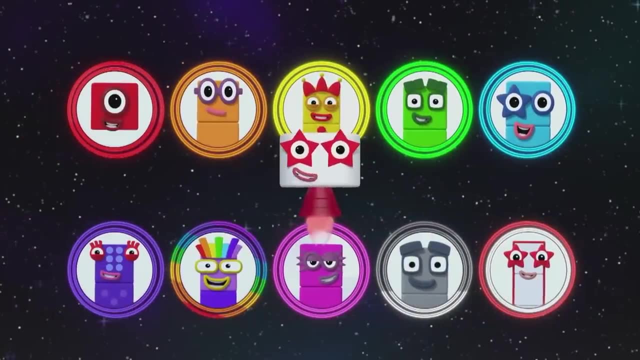 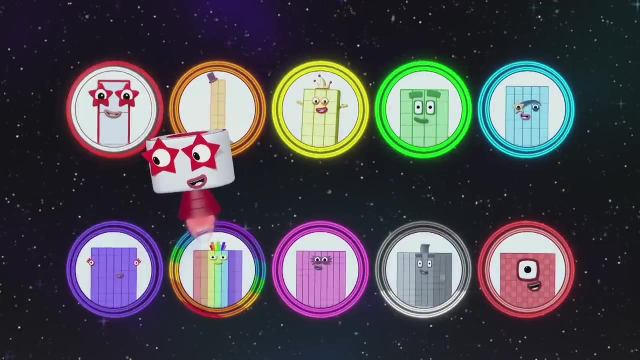 Hooray 20!. Hooray 10! Hooray. If you can count to ten, then you know the ten times table. You just need an extra zero to make your favorite hero. One ten is ten. Two tens are 20..